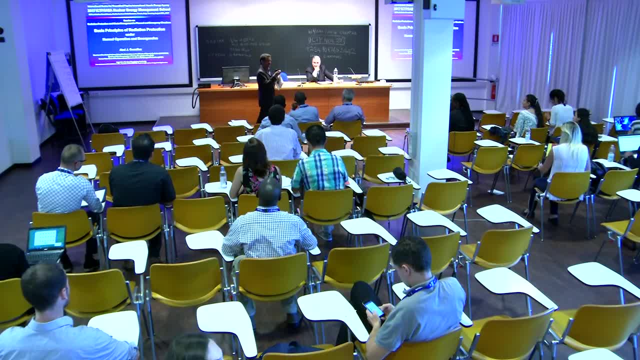 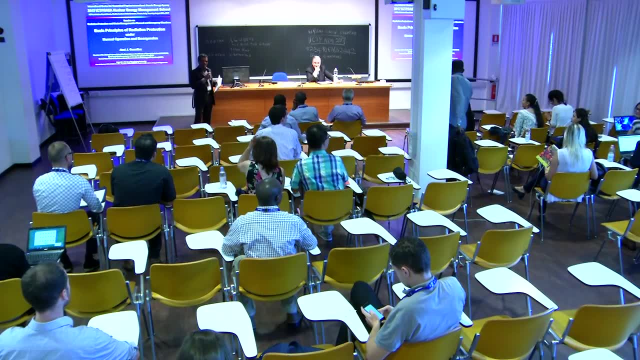 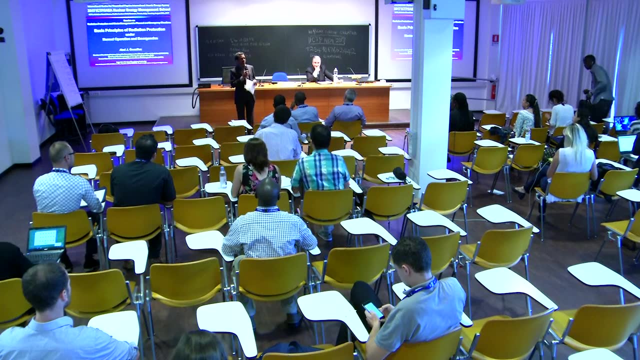 for the group three project. So if anybody by mistake taken, please give it to me. I'll collect it later from you. Thanks for that. That's one thing, Thank you. Then another thing is we are going to have a site visit, the nuclear power plant visit. 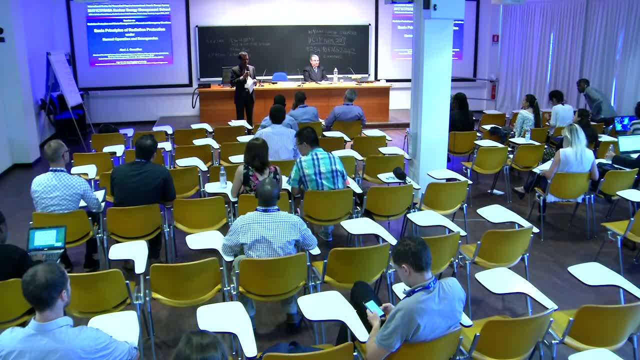 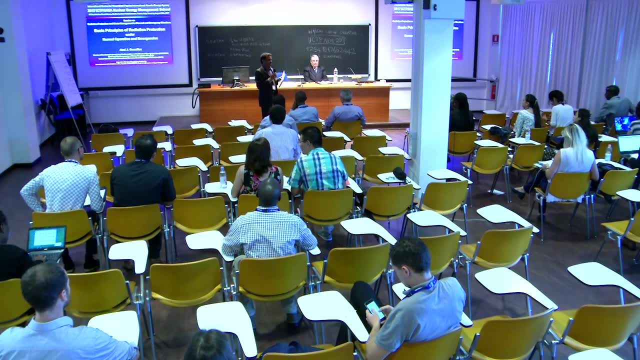 on next week Thursday. It's going to be about two, two and a half hours journey from here. I will give you more specific details. one or two days before Approximately, we would start around 6.30 in the morning and we would be arriving at the nuclear power station premises. 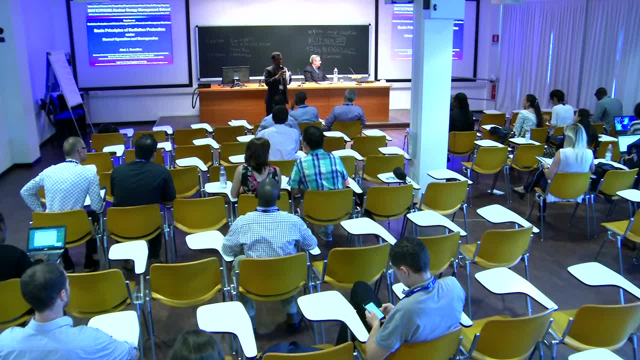 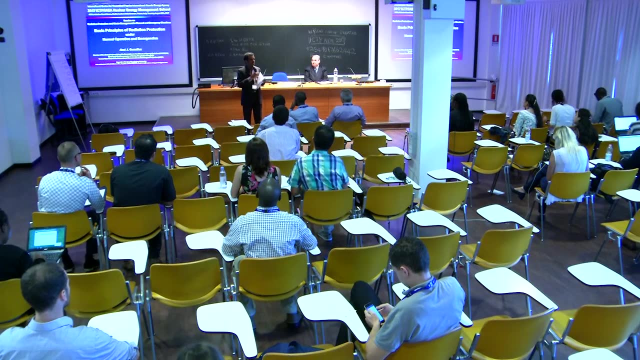 around 9.30.. 9.30 we start information center. They have a nice information center. They will explain how the nuclear power plant works and many models and things like that. I guess That is for about two hours a presentation and a visit to the information center. Then. 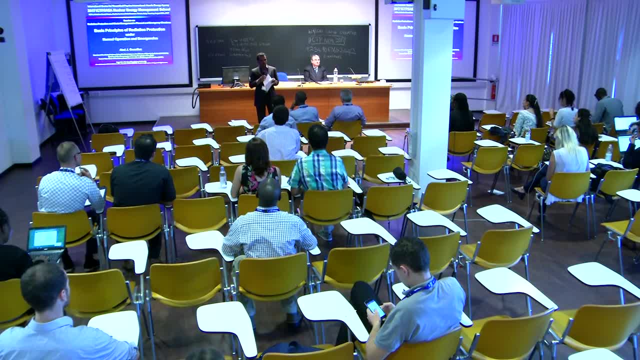 about 12.30, around 12.30 we will be taken to the nuclear power plant and we will see the power plant per se. But you know it's a BWR plant. Most of the BWR plants are having radioactivity. Even the turbine hall you cannot see in a BWR plant. So it's going to be a 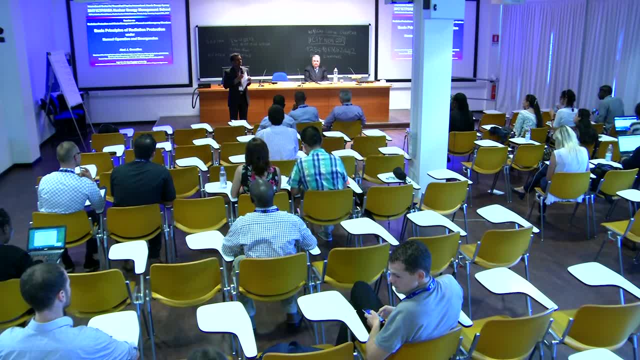 30-minute trip. We also have a power plant, So they have radiation. As a visitor, we have no access to radiologically controlled areas, So they would just show us from outside the control room and some facilities just outside, But you'll have a feel of seeing a nuclear. 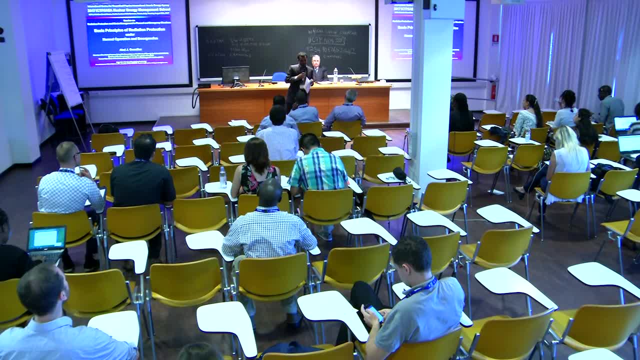 power plant. But I come to the important point Is that I've been negotiating with the plant for a visit of all the 39 people present in the school, but the NPP has a strict regulation: only a maximum of 30 people into the NPP. 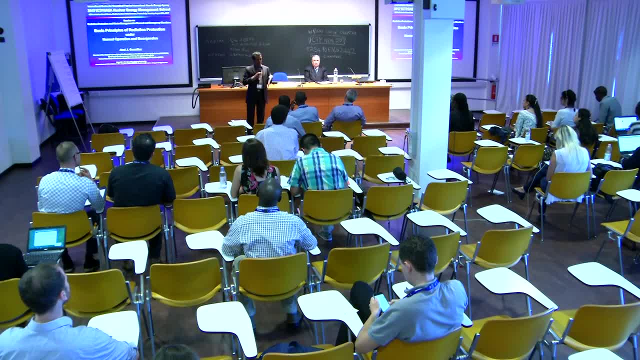 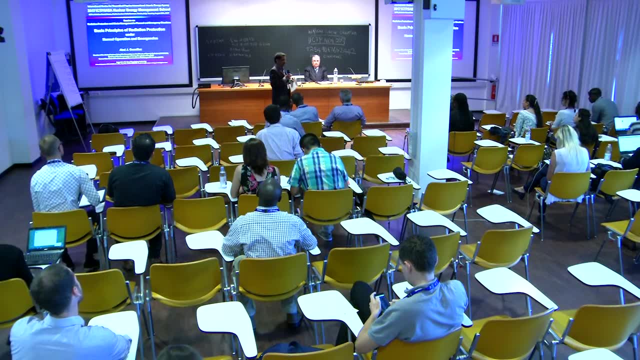 But the information center. visiting the places, no problem, All of us can visit. But going into the NPP they have some security regulations. They can allow only 30s, So it's very difficult for me to choose which 30 out of these 39. 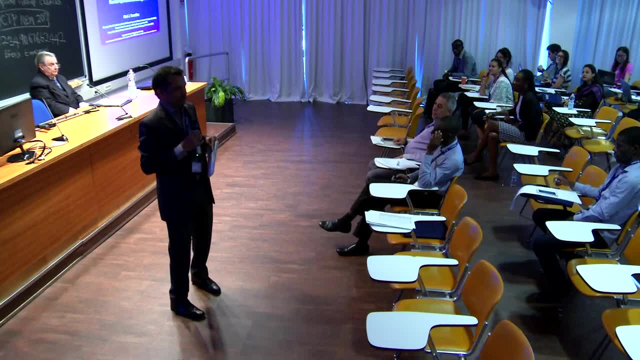 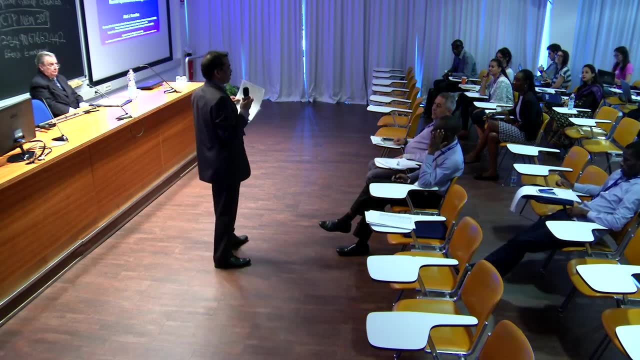 I have. I cannot follow any guidelines, So what I need your help is that I'm going to circulate a paper. If you are very much interested, please sign on this. Suppose you had seen a plan For me. it's not a great deal. 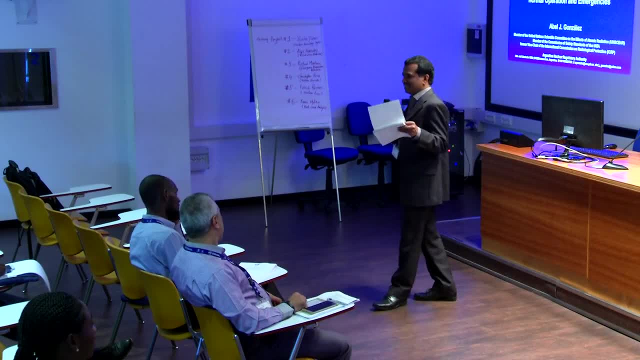 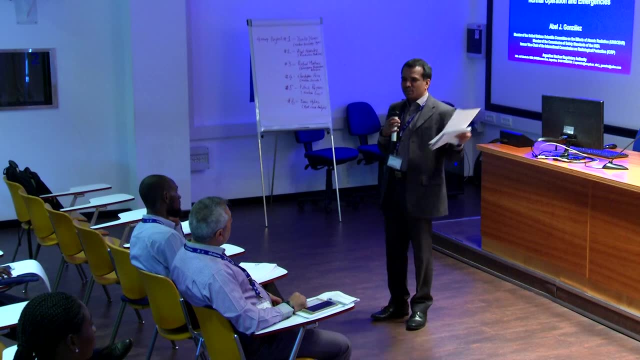 I had seen many nuclear power plants. I lived in a nuclear power plant for 30 years, so it's not important for me, But some of you have come all the way from tens of thousands of miles. I do not know that. So if you are very keen on that, please sign. 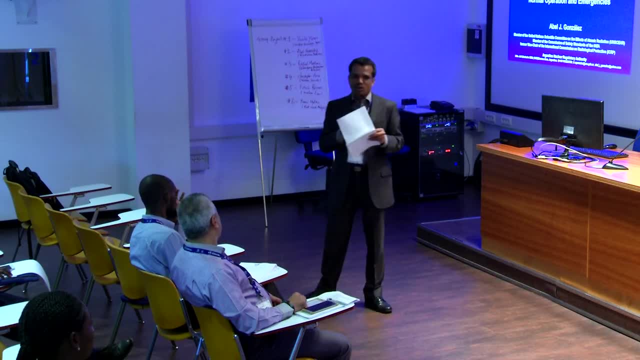 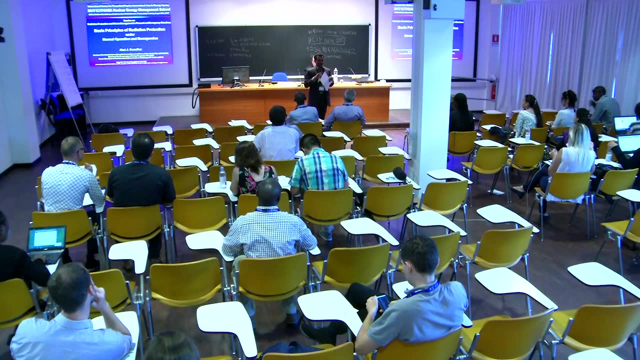 I don't want those people to lose an opportunity to see how an operating nuclear power plant looks like. I hope you appreciate the concern and the situation in which we are working. I look forward to your cooperation in this. Just sign on this At the end if you are very keen. 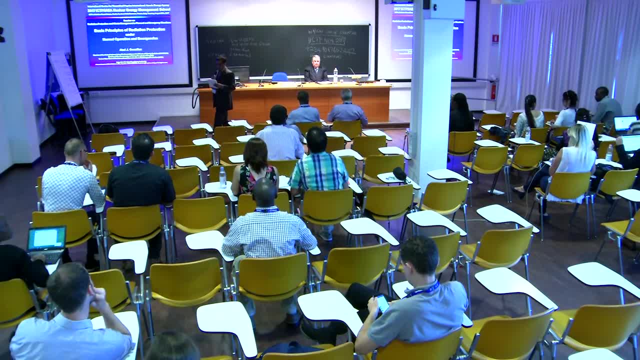 But we have 30 people who can go, So with that we will start the class now. Now it is on radiological protection, the first session Morning we have Abel Gonzalez. You had seen him yesterday. He started a very interesting speaker. 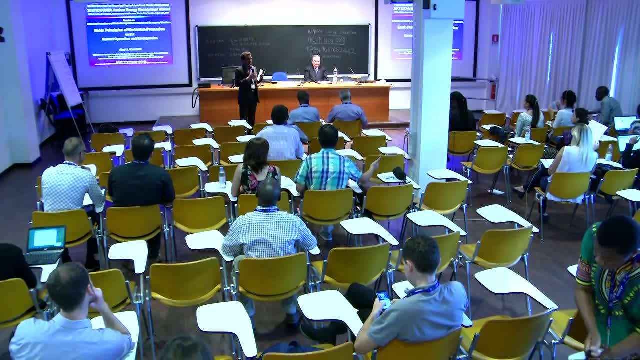 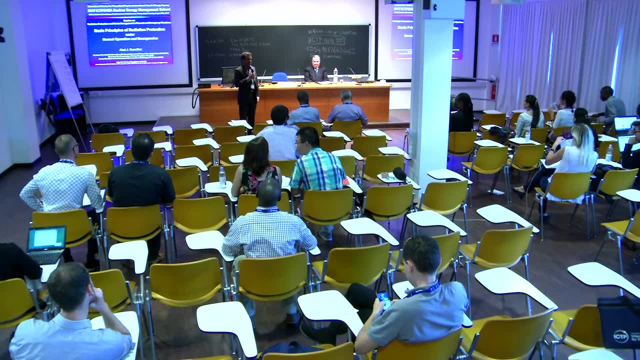 And he has a lot of knowledge and wisdom. I would say, because of his age and experience. He has a lot of wisdom in the area in which he is working And he's an academician. He has, I don't know, maybe more than my age of experience he has. 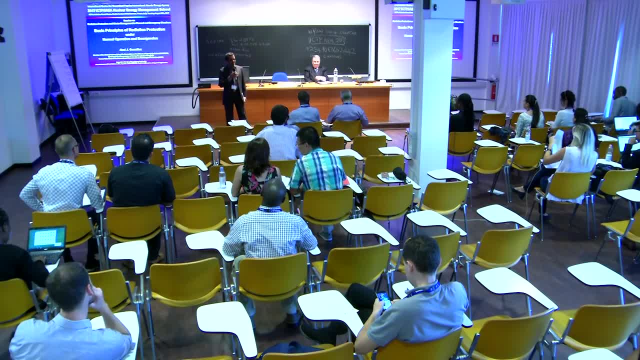 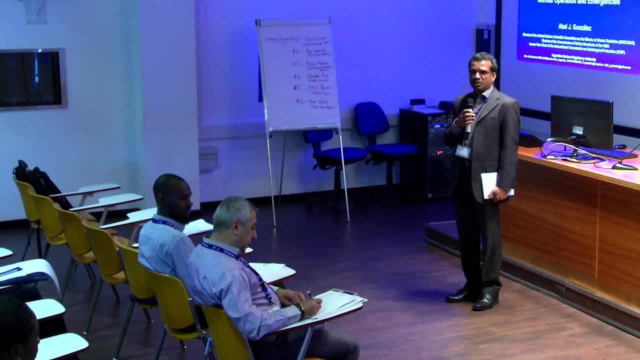 And I am quite older than 50 years, But his experience is much more than that And he represents several international institutes in the world related to radiological protection And he's been to IAEA, ICRP- He was vice chairman or something. 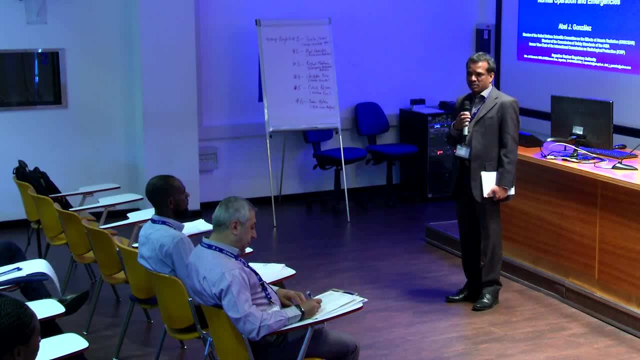 And many, many international organizations which deal with radiological protection you can name. he would be a member of that. So we are very fortunate to have him here in ICTP And I'm sure we are going to have a very interesting and enlightening lecture about radiological protection. 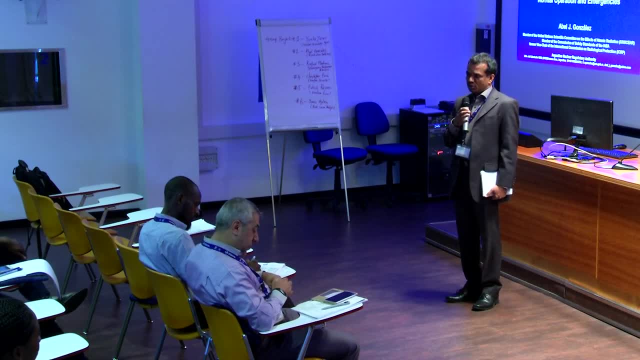 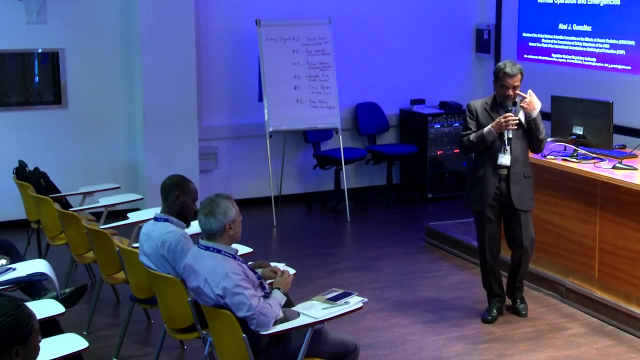 a very key area that he's going to bring And he's also going to talk in a different dimension about the radiological protection. So, without talking much about him, he will explain about himself later. I will hand over the dice to him. 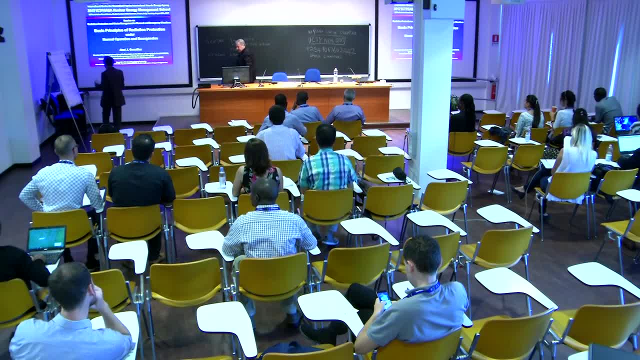 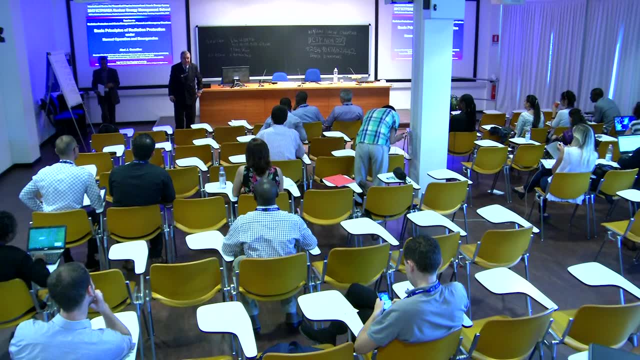 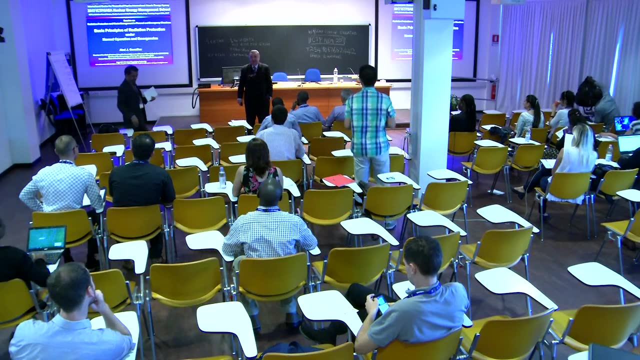 Thank you very much. Thank you Well, good morning. How are you Fine? You had a nice dinner yesterday. I understand. I apologize that I could not be with you, But I was traveling. I was very tired. You know, you can recognize that in Italy people eat well. 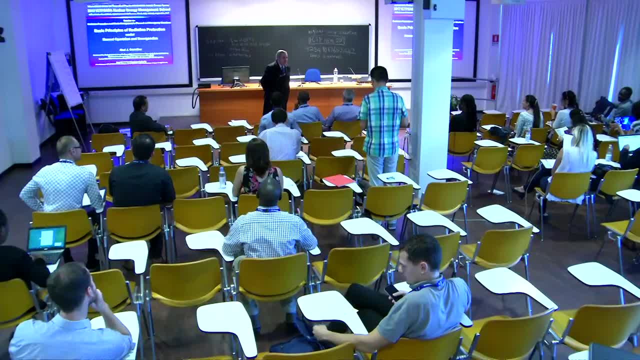 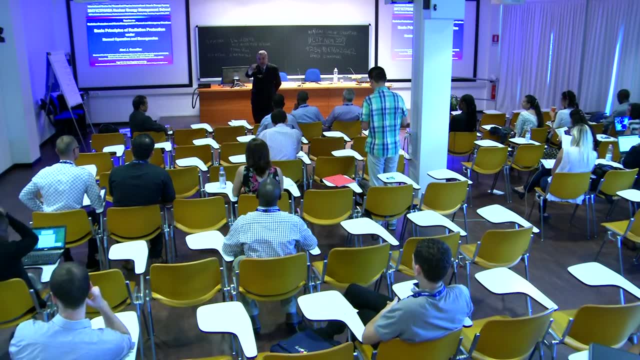 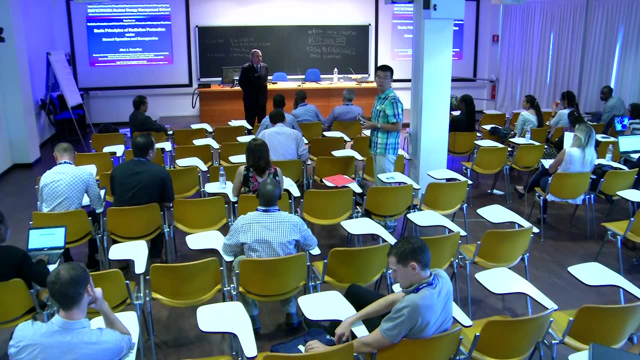 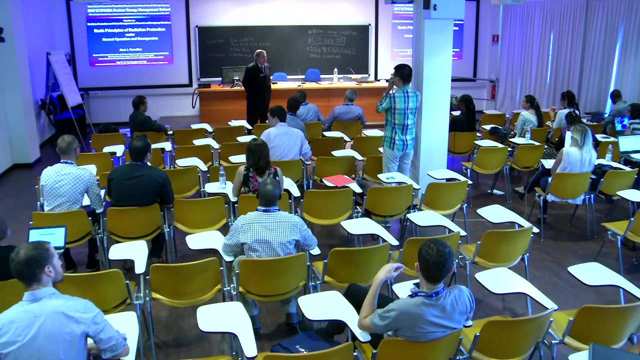 Well, we are here to walk with you on the issue of radiation, with my friends, Rafael Martini that is sitting there, And Rafael is one of the best experts that I know in how to deal with emergencies with radiation And therefore proved from experience today. 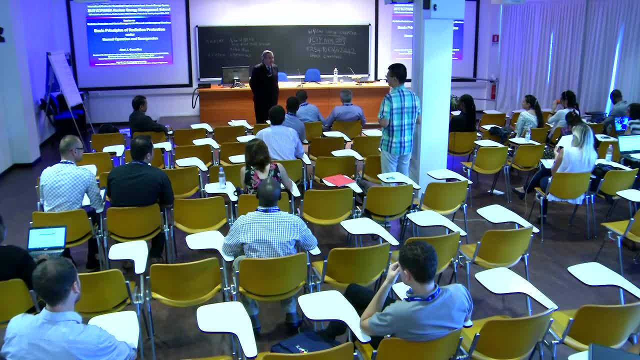 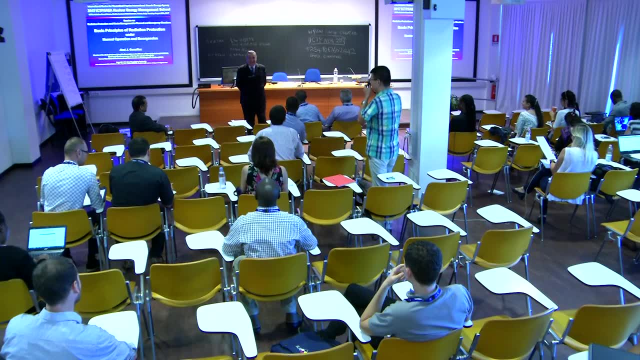 Because he really has a lot of experience. In addition, he's a fantastic friend. You know, You know what is the difference of a friend than a relative. When we are in travel, you never go to a relative, You go to a friend. 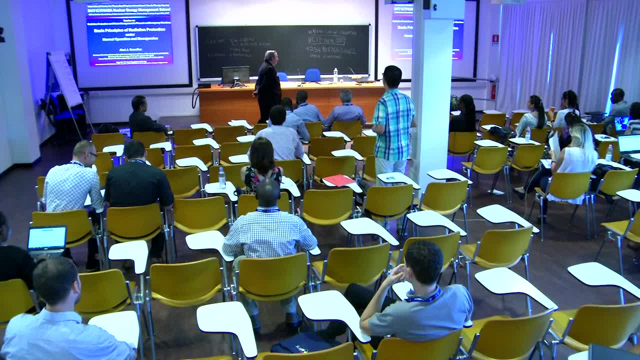 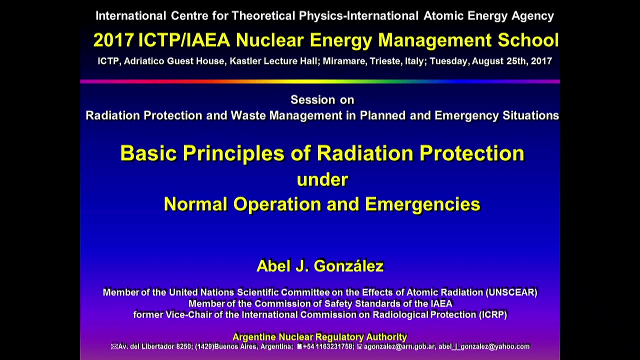 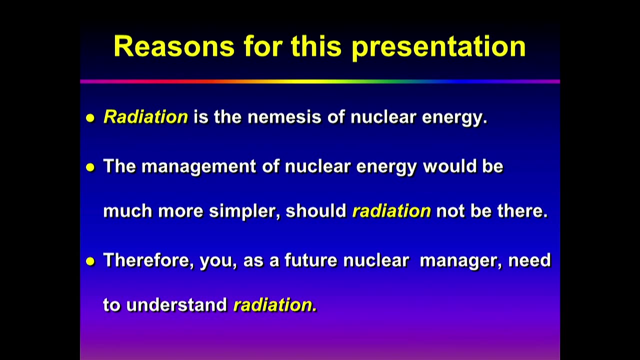 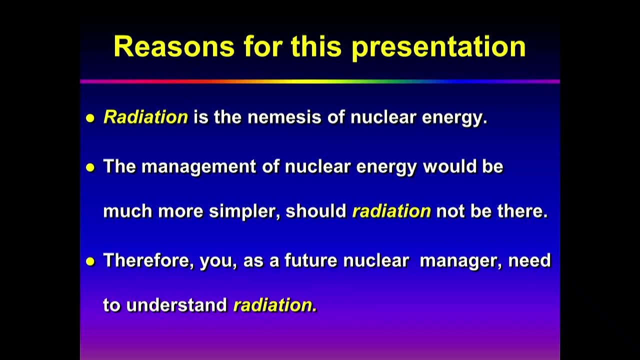 why? Why we are talking about this in this course? Well, because radiation, we like it or not, is the nemesis of nuclear energy. It's a big problem of nuclear energy. The management of nuclear energy would be much more simple should radiation not be there. 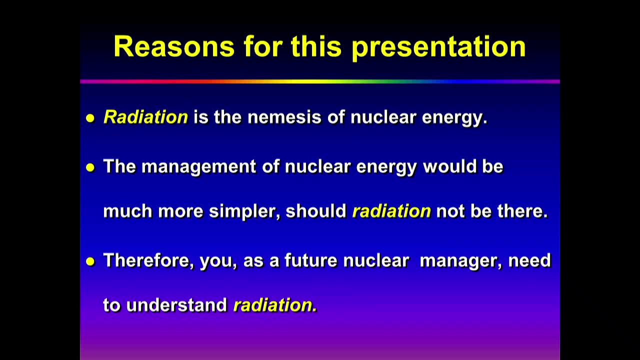 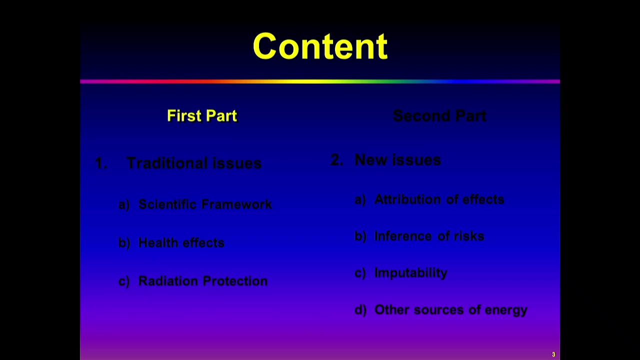 It would be completely different. The reason why we have so many problems with nuclear is radiation. Therefore, you, as a future nuclear manager, need to understand radiation, And that is the feeling of this presentation. This is the reason I will have as a content. as a first part, I will talk on traditional. 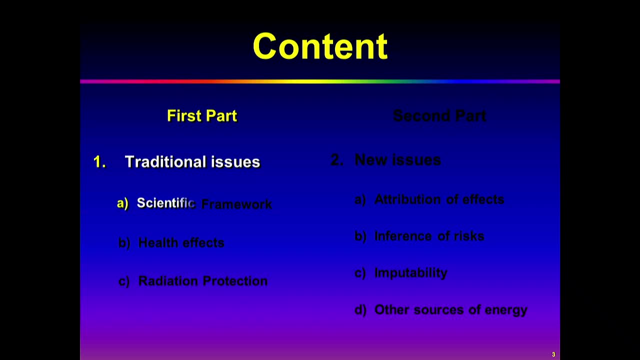 issues, the issues that normally you talk in courses like this: The scientific framework that we have for this, the health effect of radiation that people are always interested, and radiation protection. But I have introduced, after talking for a short time, a second part which gets you to new issues, Issues that normally are not there. 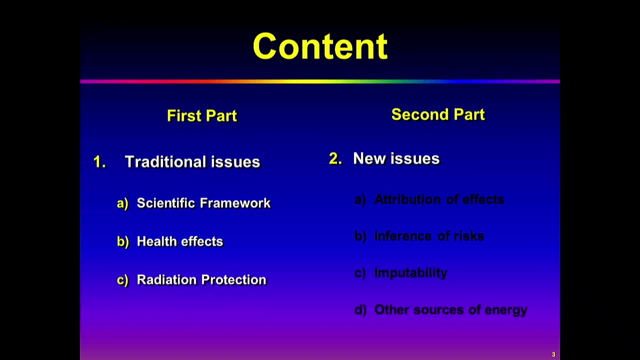 You will not find in books, because they are really very new issues. One very new issue is on whether or not we can attribute the effect to radiation- And that is a very controversial point- in low doses. The second is whether we can still infer risk or not, And that is. 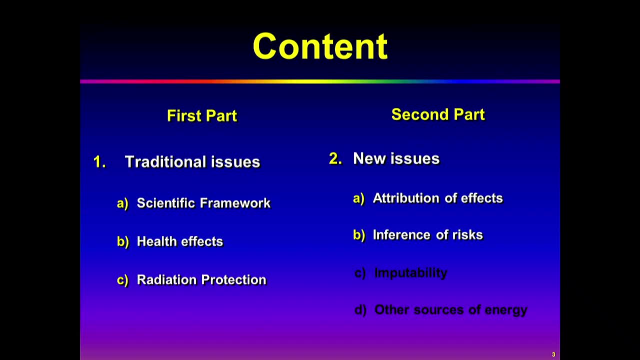 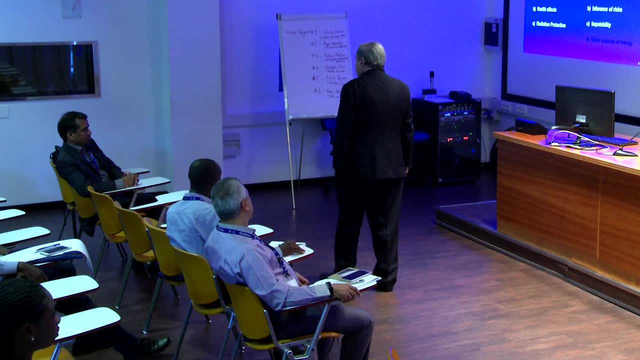 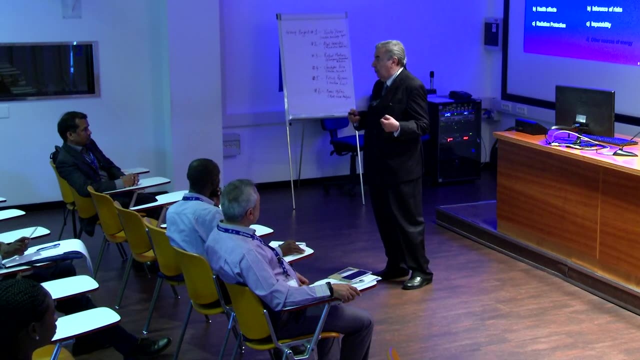 a big difference between attributing something or inferring. Attributing is objective, Inferring is subjective. Then we will talk about imputability, Whether, if you can attribute risk, a good lawyer can impute or not. This is an essential issue for nuclear energy Because in the current 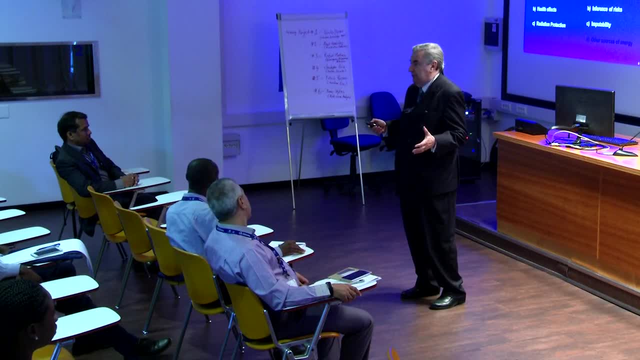 situation. the companies never know what will happen. I mean, if somebody has a good lawyer, he can bankrupt the company For that. it's a very important issue which is open. This is not solved. And the third one I will talk on radiation. 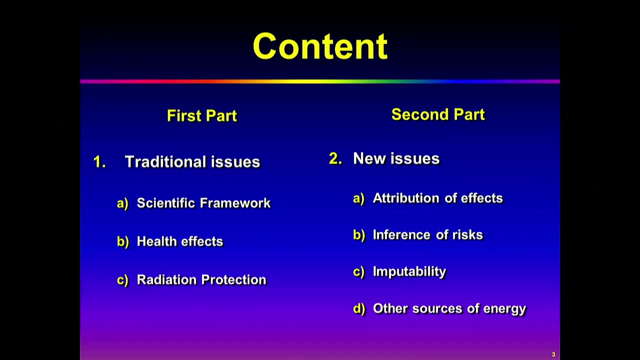 in other sources of energy. This is really very, very, very new. It was approved just a few months ago by the UN General Assembly. Therefore, you are going to have the traditional thing that you will find usually in normal courses, plus very, very new issues. 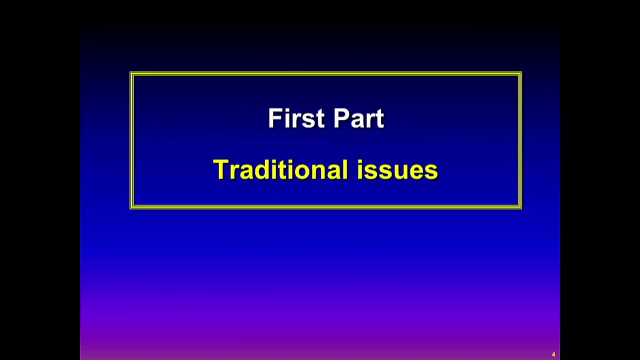 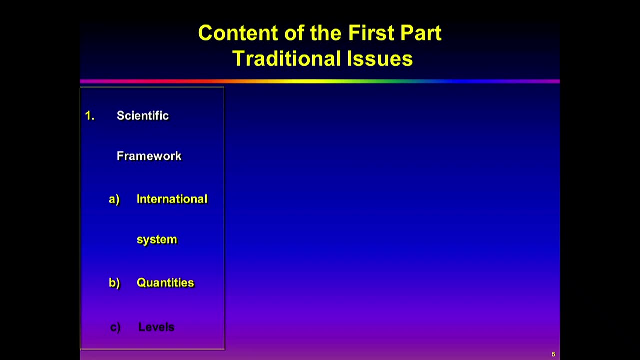 Well, let's start with the first part, the traditional issues. I will talk about the scientific framework, international system, quantities, levels, the effects- biological effect, deterministic effect, stochastic effect- and protection, The basic recommendation, what we call risk-efficient protection in practice, international standard For this. 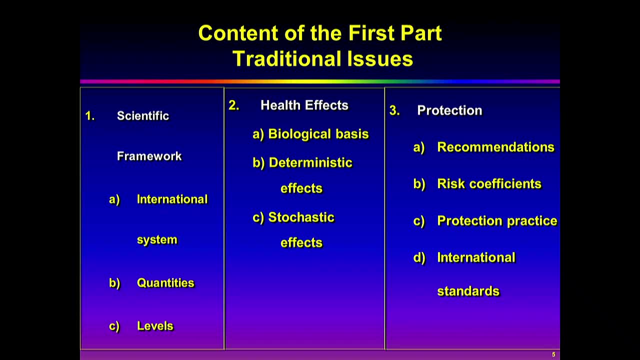 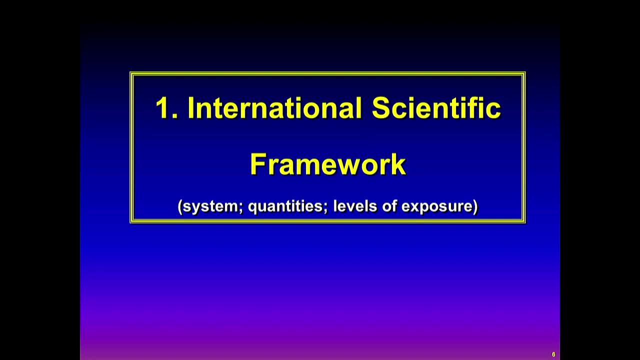 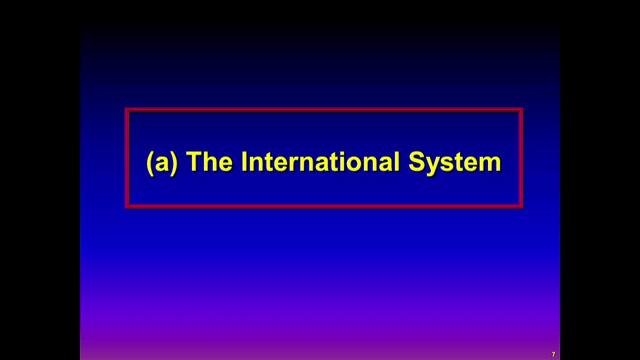 a long, long story. This is the first part of the program, the one that I have in front of you. What is international framework? It's important that you understand the international framework for all this And let's start showing to you how the international system works, for good or for bad. 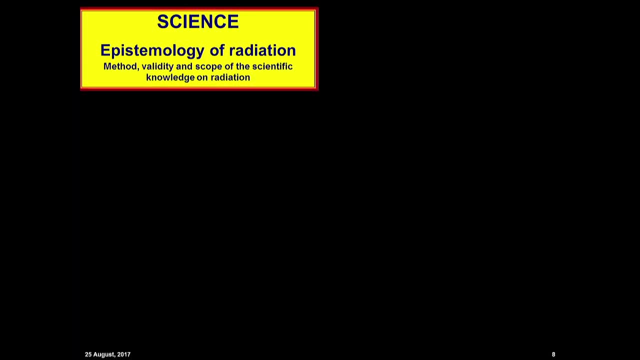 The international system first of all deals with science, which is called the epistemology of radiation method, validity and scope of what we know. And we need an international consensus on this, because if somebody says something, somebody says something else. Then 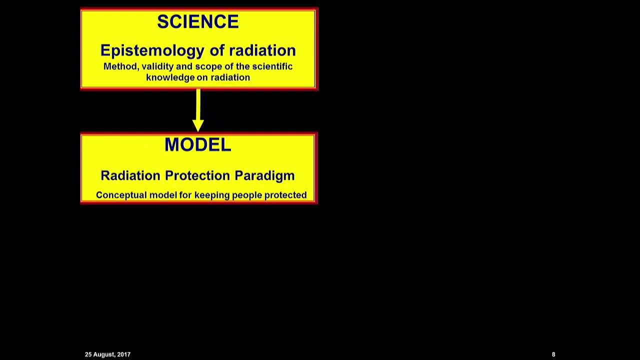 when you know the science, you need a model, or what we call a paradigm. under what model you protect people? You need to assume a model, usually on the basis of ethical rules. You don't want that people be killed, You don't want that people be harmed. Then, once that, 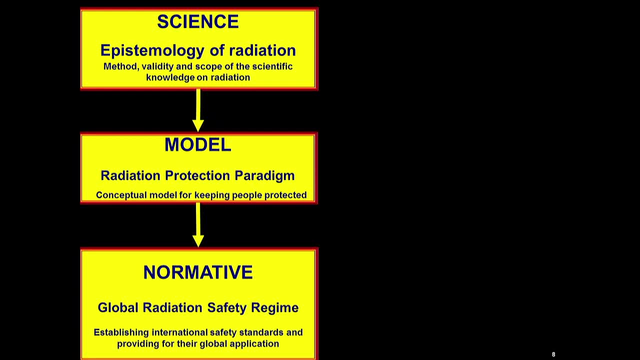 you have the science and the model. well, you need a normative standard. If not, everything is blah blah blah. You need a global radiation safety regime. Well, how this has been achieved internationally? In the following way: The science is concentrated. 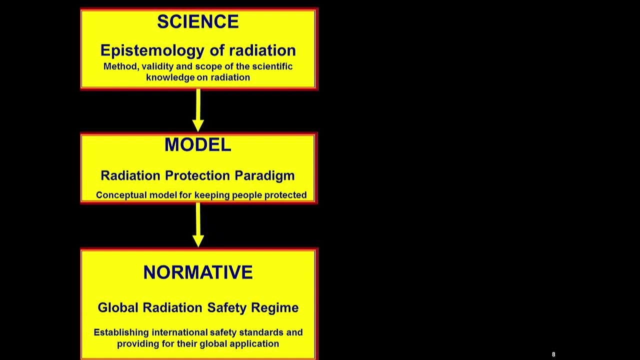 believe it or not, at the top level of the United Nations. The General Assembly takes this on board, not because the politicians in the Assembly are interested in your health, but because the science was very important to see the impact of nuclear weapons And 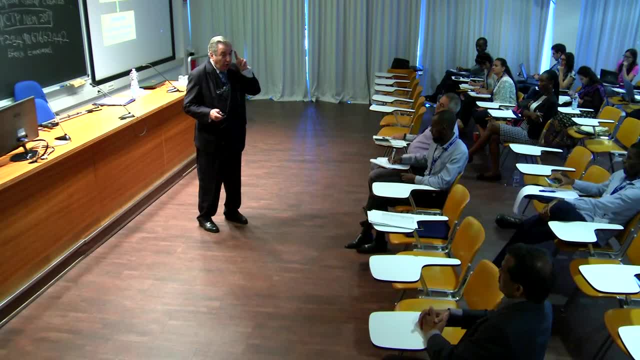 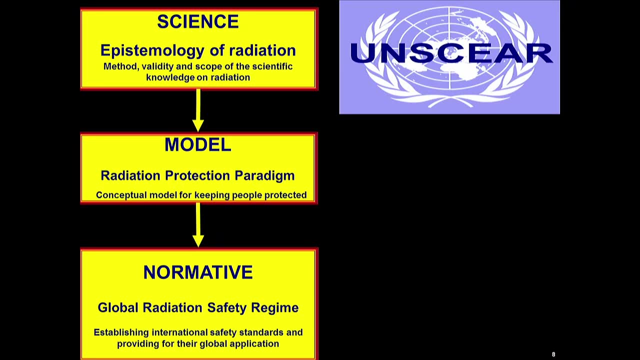 for that reason they created the only scientific committee. the only in the General Assembly is called UNSCEAR- United Nations Scientific Committee on the Effect of Atomic Radiation. Since the year 55, this committee, every year, submits a report to the Assembly on the science. 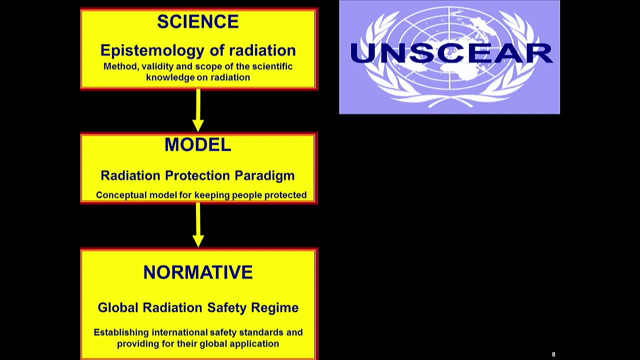 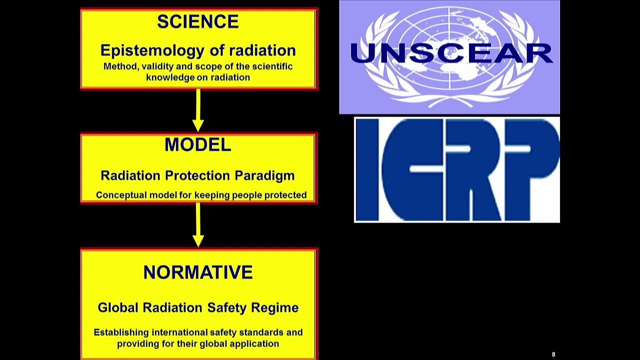 levels and effects of radiation. Thank you. The model, for reasons that nobody understands well, has been in the hands of a non-governmental organization from the year 1928. It's called ICRP- International Commission on Radiological Protection. It was originally created by the doctors that were very afraid of radiation. 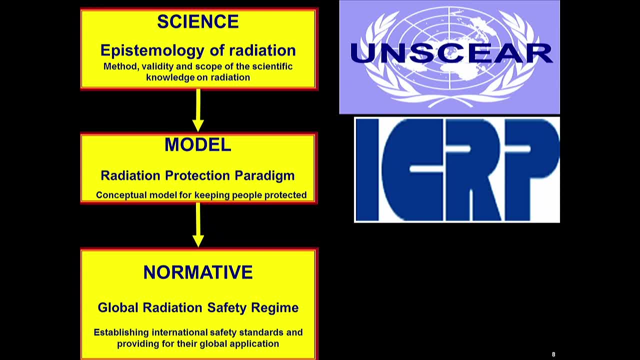 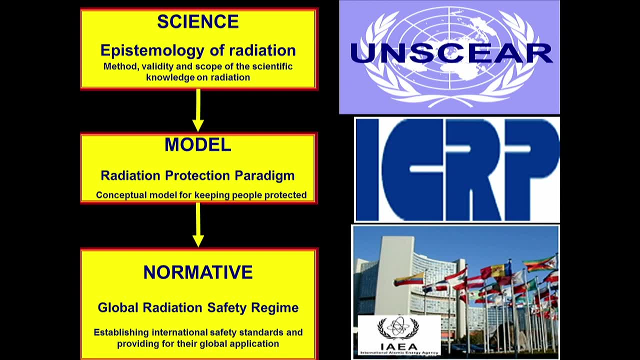 They were being burned in the 20s And they created this organization to give a paradigm how to protect themselves. And the standard, the normative, is in the hands of the UN. The International Atomic Energy Agency is the only body in the United Nations with the 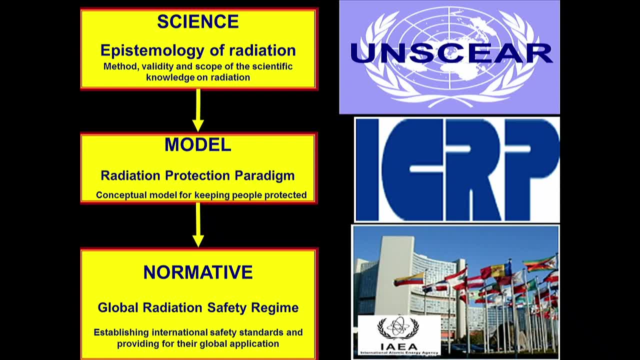 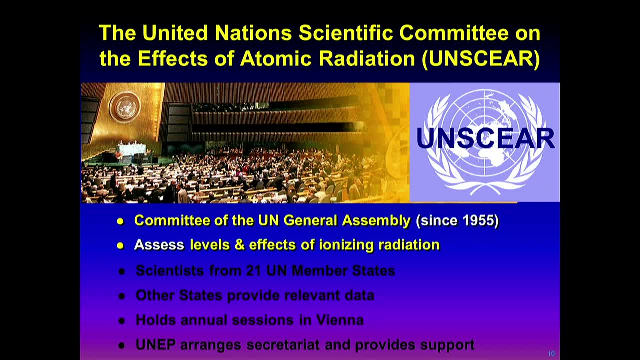 statutory power to impose standards. Therefore you have UNSCEAR. as I said, it's a committee of the General Assembly assess levels and effects. it has 21 member states. Others provide relevant data meetings in Vienna. UNEP arranges a secretariat. The secretariat decides if the results of the UNSCEARs are. 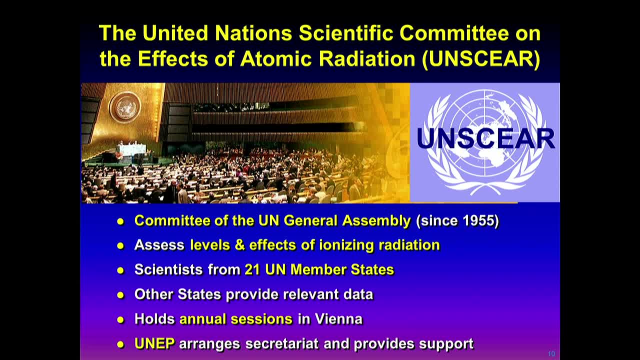 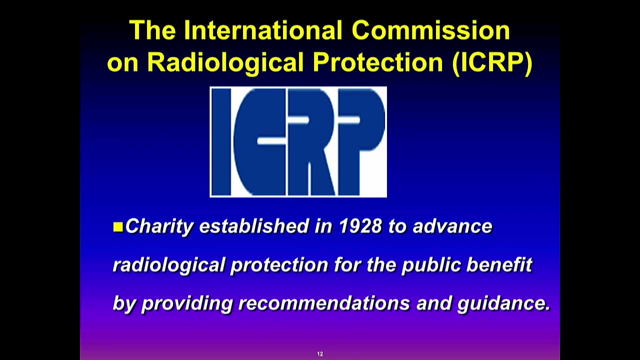 available or not, The secretariat is in Vienna. If you go to Vienna you can see. it's a different building than the agency. It's in the other extreme. ICRP is a charity established in 1928 to advance radiological protection to the public, providing recommendations and guidance. 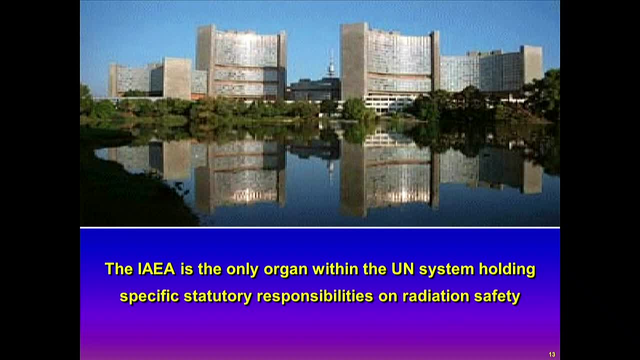 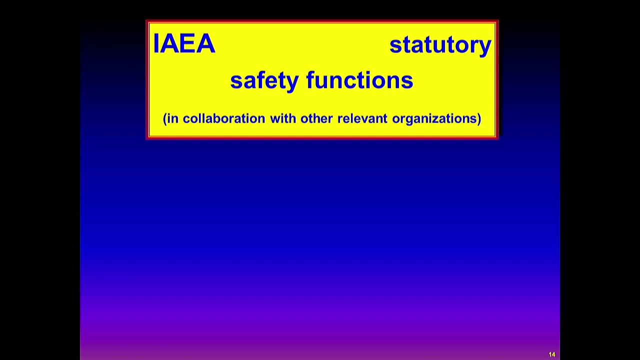 And then you have the agency. As I said, it's the only organ in the United Nations with statutory responsibilities. What are the functions of the agency? This is important for you to know because people normally are confused about this. As I mentioned just in the discussion, the agency has only two functions in this field. 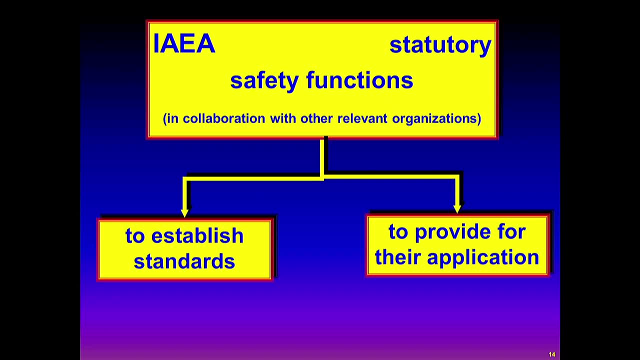 To establish a standard and to provide for the application. Establish a standard means to approve a standard- what Catherine explained to you yesterday- And to provide for the application are all these services that the agency offers and that you can use. The agency also facilitates international conventions, but the agency is not part of the conventions. 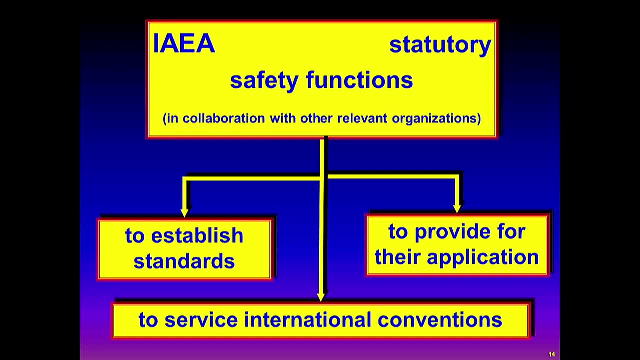 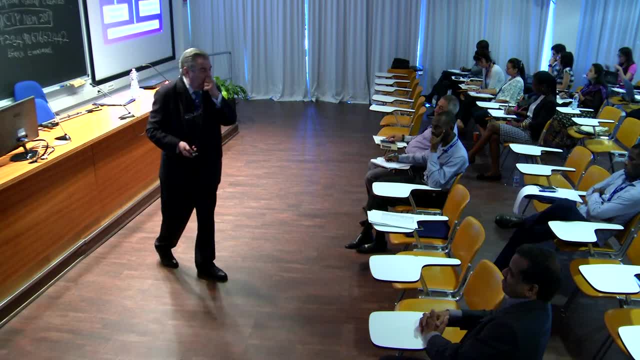 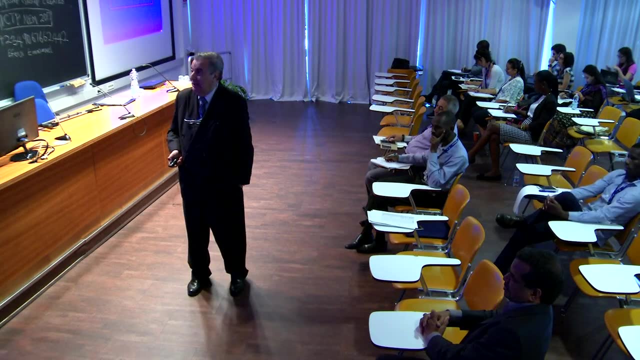 The conventions are agreements among countries, are contracts among countries, And the agency is there to help provide coffee in the meetings, water paper to write a building. That is what the agency does Now, the first thing for reaching an international agency. 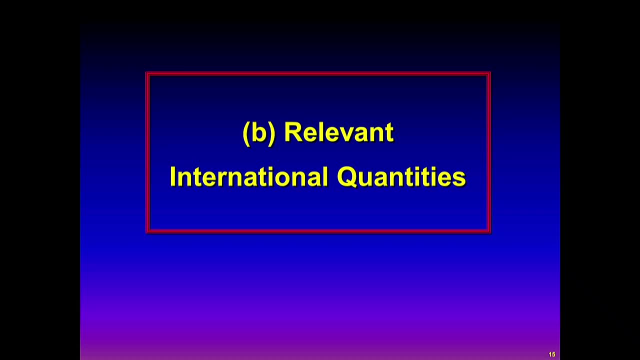 The first thing for reaching an international agency is an agreement on the quantities. I mean, if you do not have an agreement on what a meter means, you cannot build a building. There was an agreement on what a meter means For radiation protection. you need an agreement on the quantities that you are going to use. 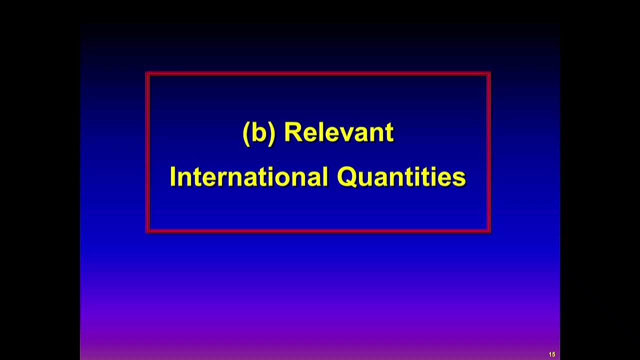 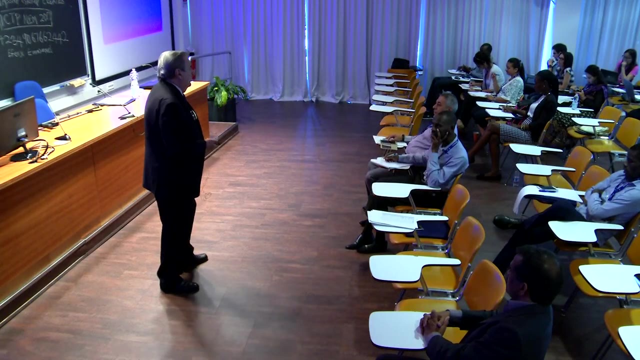 This agreement is very complicated and has caused a lot of problems. I personally believe that it is unnecessarily complicated, but it's there. It has been approved by everybody. First of all, there is a confusion between radioactivity and radiation. For many of you, this is stupidity. 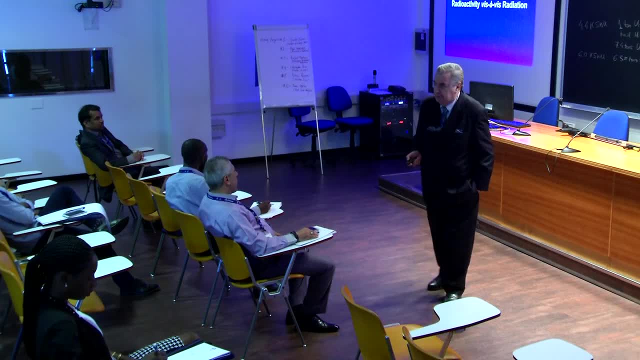 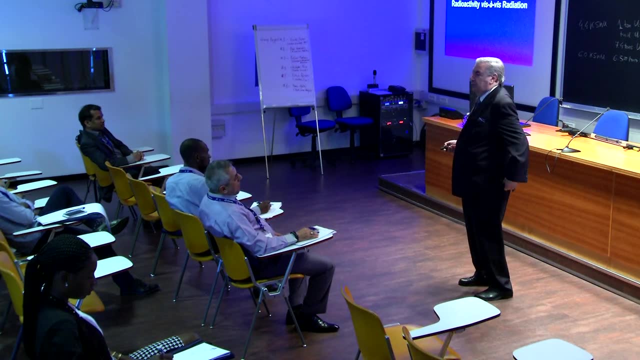 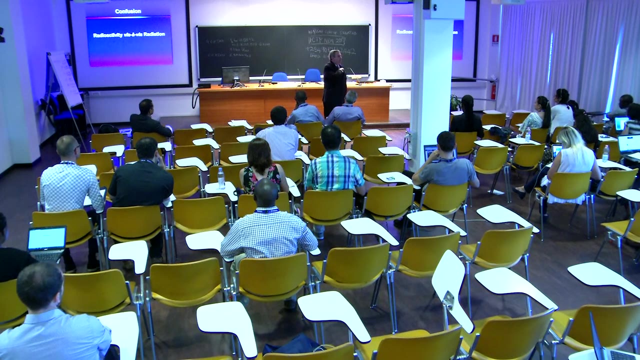 Well, it is not. You will see top people confusing radioactivity and radiation. Typical case is when somebody decides to irradiate food for preservation. People immediately say no, no, no, I don't want this to be irradiated. 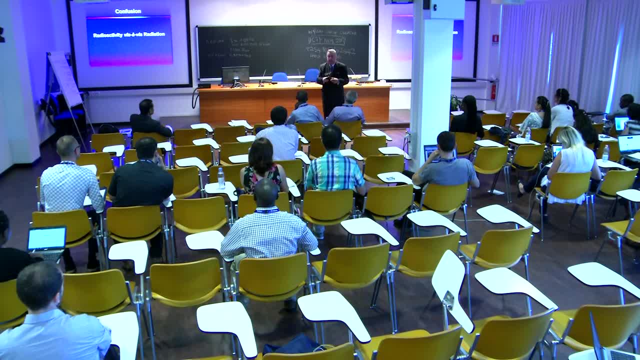 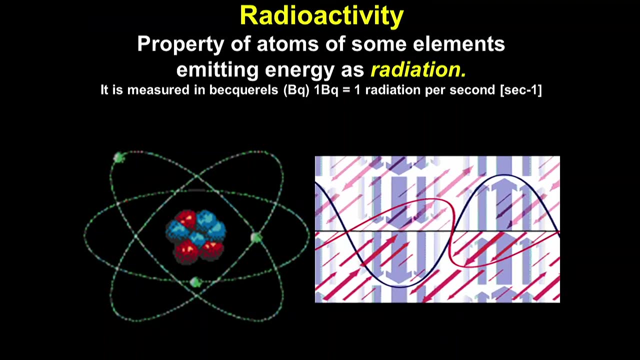 I don't want this to be irradiated, because then I will be contaminated. This is a typical case. Therefore, there are these problems between radioactivity and radiation. Therefore, let's start clarifying that Radioactivity is the property of atoms, of some element, to emit energy as radiation. 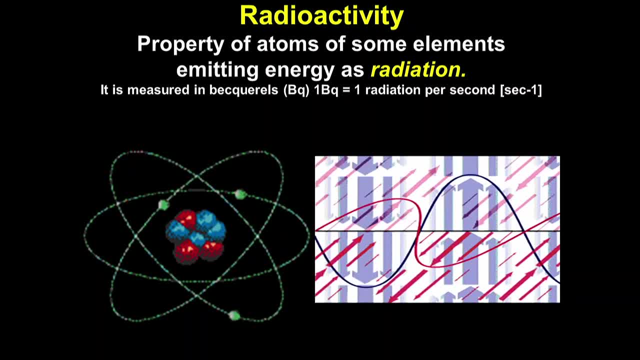 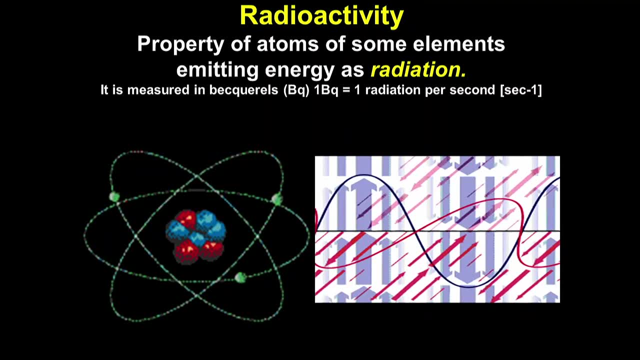 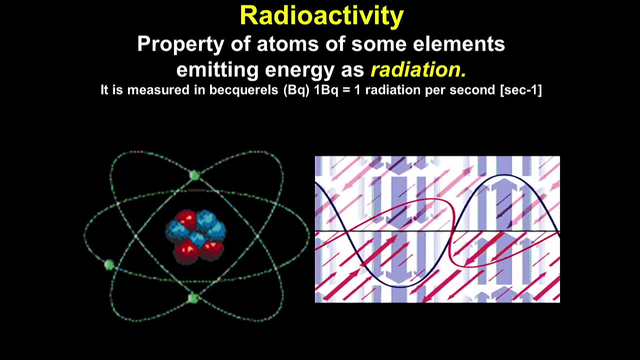 Radioactivity is the source of radiation. It's measured in becquerels. One becquerel is one radiation per second All over the world. But there is one country that does not measure radioactivity in becquerels but in a different unit called the Curie. 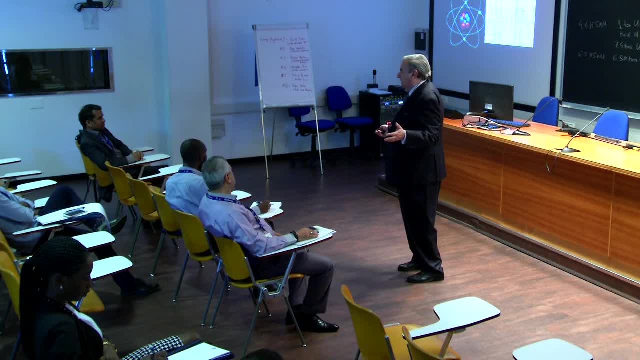 You will say: well, I don't care. I mean, we have 192 countries. There is one that can do that. It's a problem. The small problem is that this country is the United States of America, which is equal to the other battery noise. 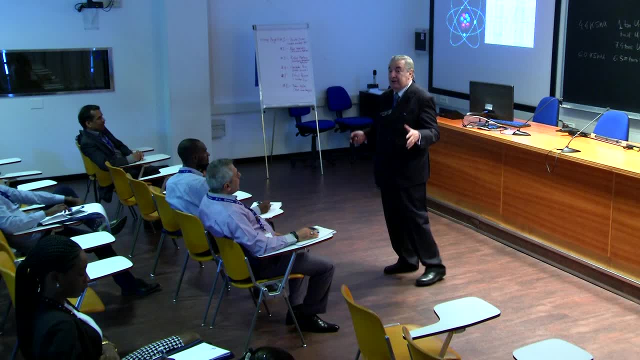 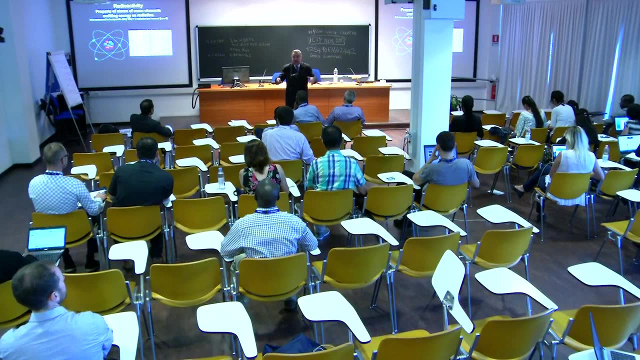 It's a little different, For this creates serious problems. Let me give you an example In Japan, the Japanese people were measuring radioactivity in Fukushima in becquerels And people were sufficiently confused with that. And then the American planes arrived and started to measure radioactivity and informed the people in Curie. 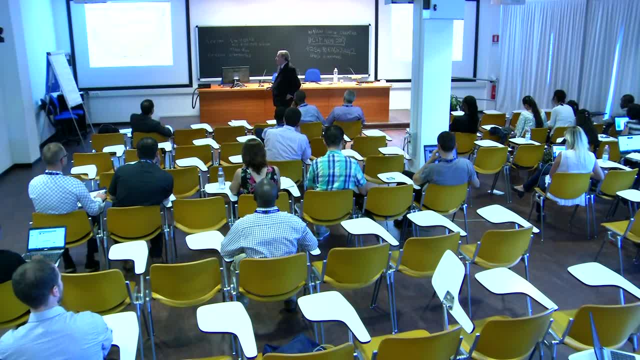 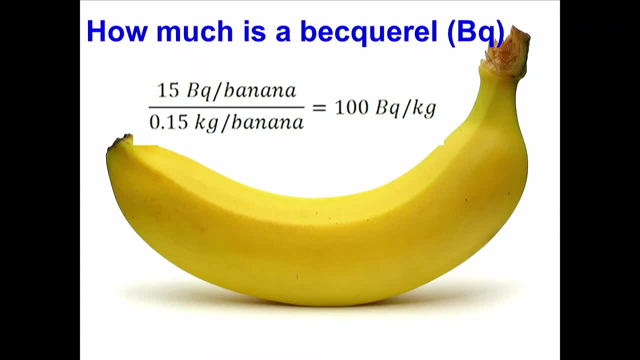 This confused the Japanese for over How much is a becquerel? A becquerel is a very low amount of radioactivity. One kilo of bananas has 100 becquerels of radioactivity- 100. So the becquerel is very small. 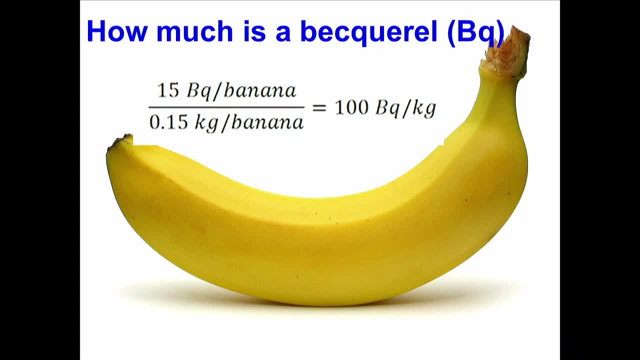 Why the banana? Because bananas, as you know, contain a lot of potassium. This is the reason why you feel very badly if you eat a banana and you get better. Well, potassium is radioactive. One kilo, 100 becquerels. 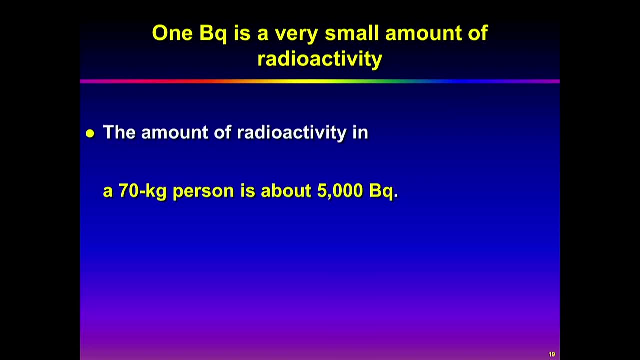 In fact, we have a lot of radioactivity in our body. A person- 70 kilo person- has about 5,000 becquerels of radioactivity in our body, And maybe this is the reason why we took a lot of bananas. 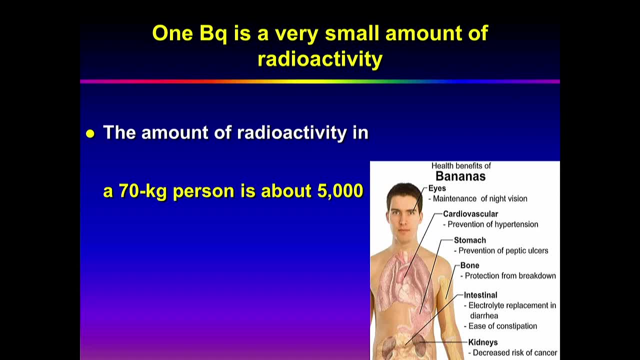 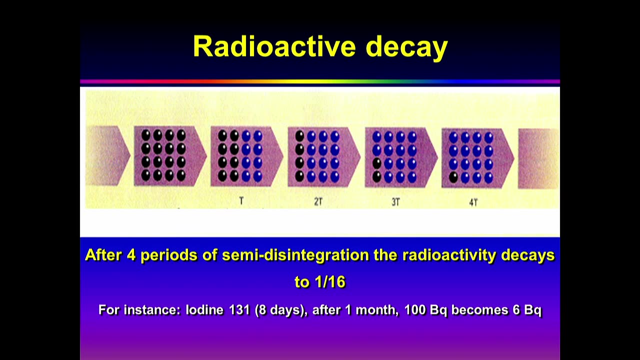 But it's radioactivity that is so important that if we get this radioactivity out of our body, we collapse. For one becquerel it's really very small. The becquerel, in addition, decay, something that people forget when we talk about radioactive waste. 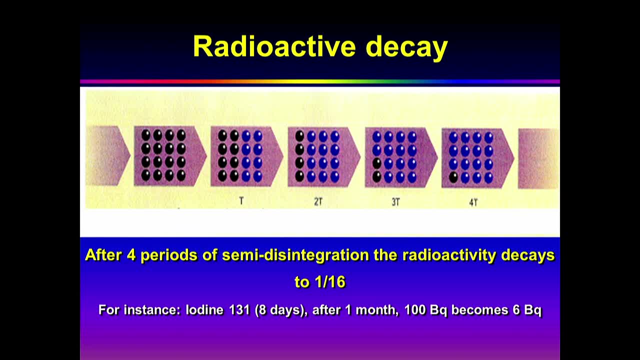 And people say, oh my goodness, this waste will go there for 30 years, 40 years. I normally ask you know, in this moment, everywhere we are changing these low-consumption lamps And we put the new LEDs that China is producing like mad. 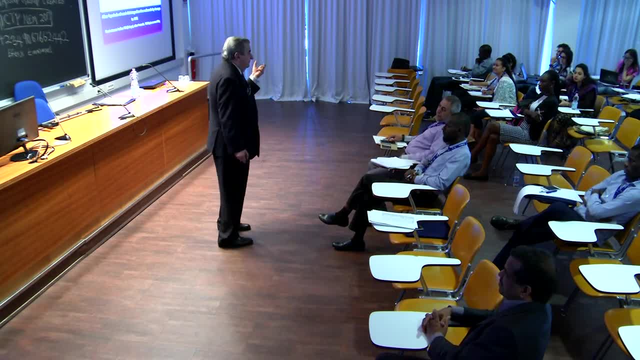 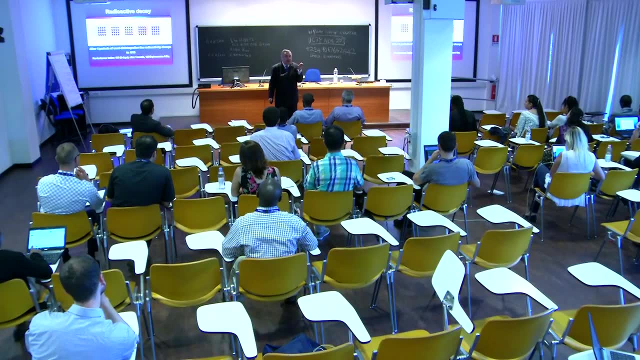 Well, you know that these lamps contain radioactivity. They contain mercury, which is really very serious pollutant. What people do with the lamps? Throw it away And the mercury do not decay, Radioactivity decay. For example, one becquerel. 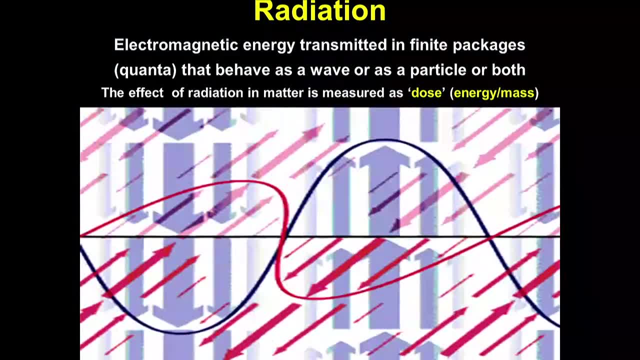 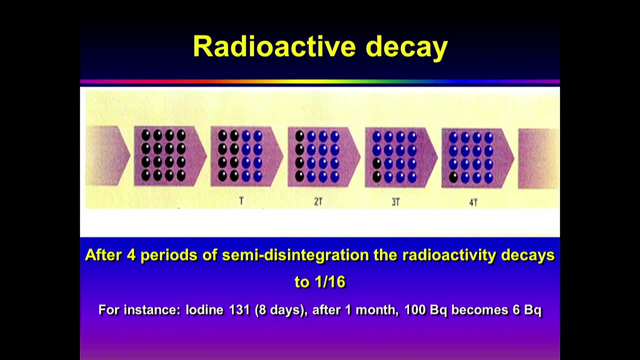 It's here, yeah, No, It's here in the middle. no, Oh, no, here, I'm sorry It's here. 100 becquerel of iodine, one of the more complicated radionuclides in nuclear, became 6 becquerel after one month. 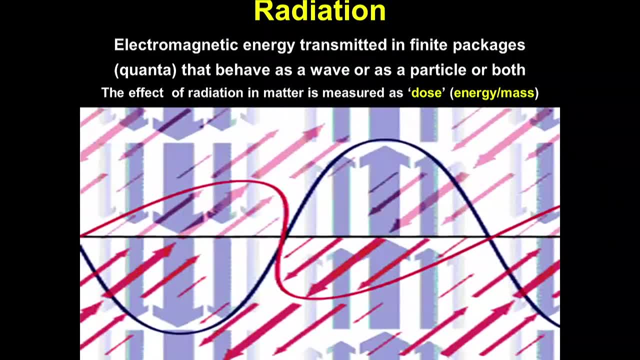 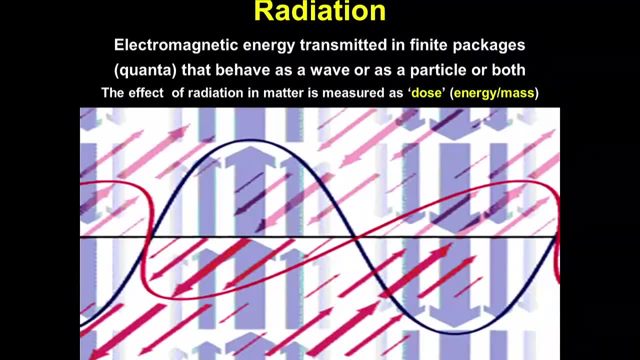 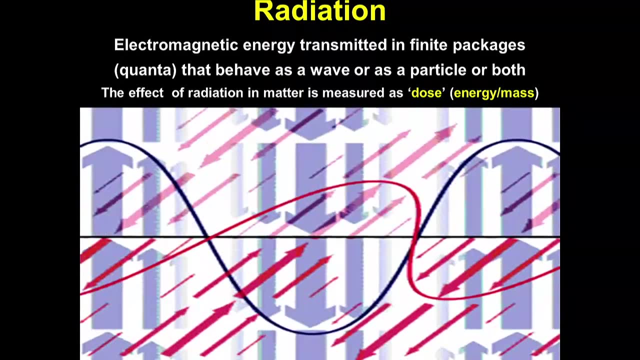 Decay and decay quickly. Now, what is radiation in that case? Radiation is, as I said to you, energy, Energy transmitted in finite packages that the physicists call quanta, just to confuse us. The effect of radiation in matter is measured with a quantity that we have called dose. 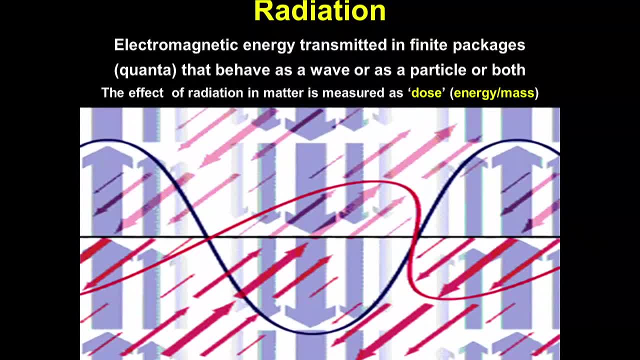 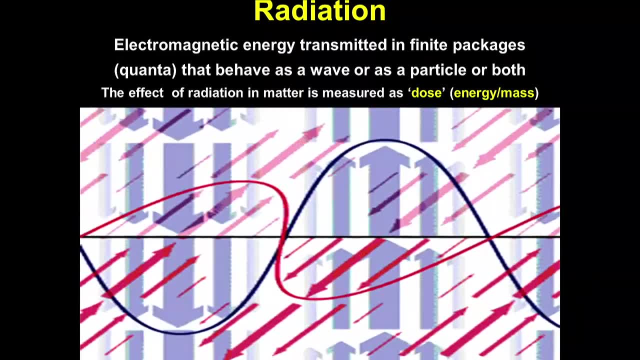 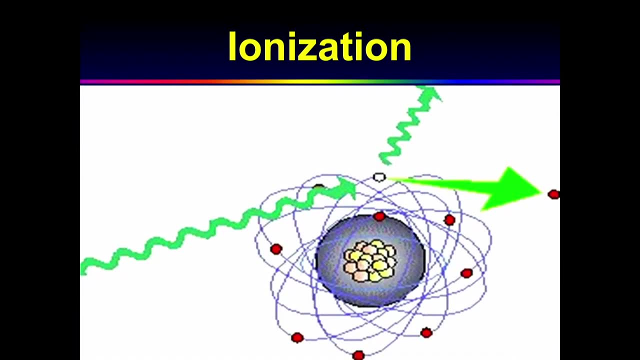 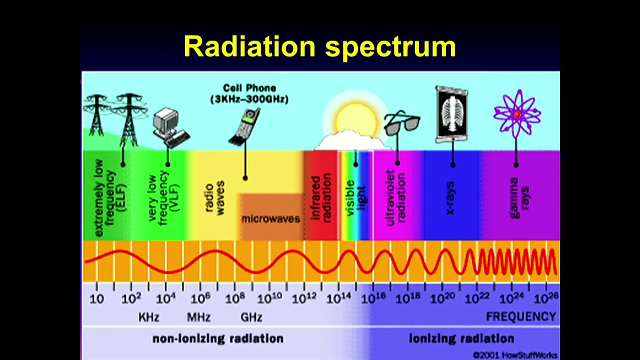 coming from the medical tradition, which is energy per unit mass absorbed. This is the dose. Okay, This has been the basic agreement. The problem is that radiation. Let me see I'm missing one slide here. Oh yeah, It was in bad order. 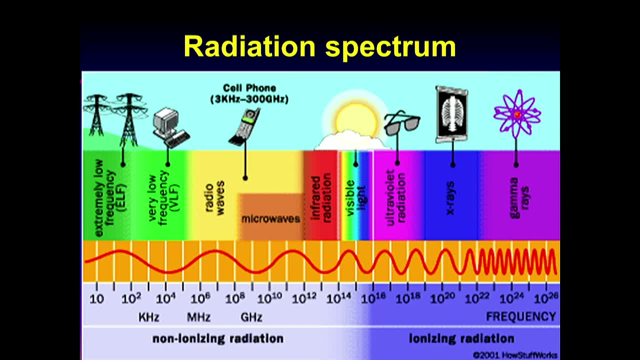 Radiation, depending on the energy that it conveys, can be produced in many different forms from the electromagnetic radio waves. telephones- Everybody asks me radiation about telephone is bad. The visible light up to the radiation that we are interested in, the nuclear radiation. 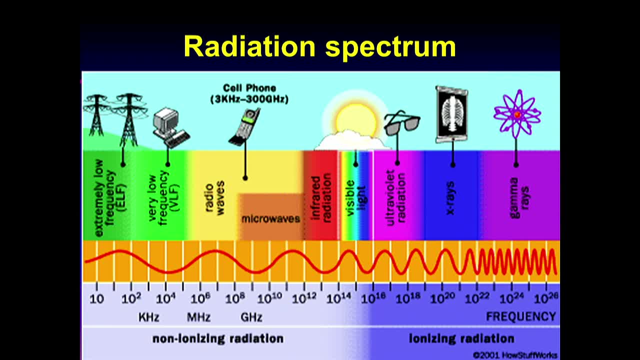 All the radiations are the same physically, but there is a big, big change in a given amount of energy. that is approximately here. Above this energy, below this energy, radiation is non-ionizing And above this energy, radiation is ionizing. 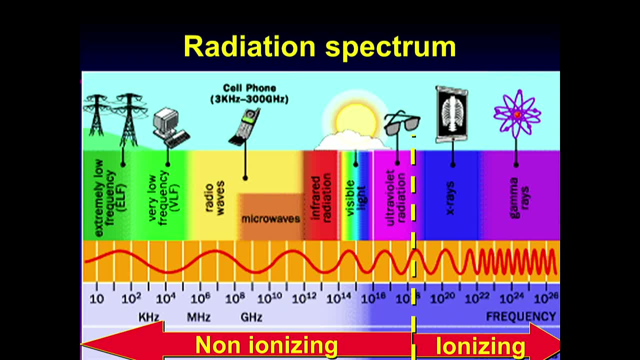 Well, we know that ionization produce problem in our body, and you will see why. And people said: okay, In that case, non-ionizing radiation is good, But, frankly speaking, we don't know. I personally believe that it is not so good. 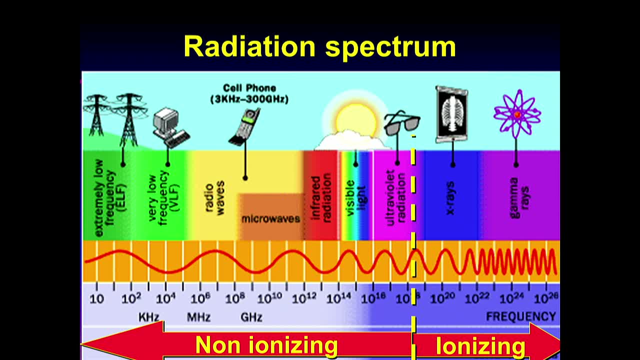 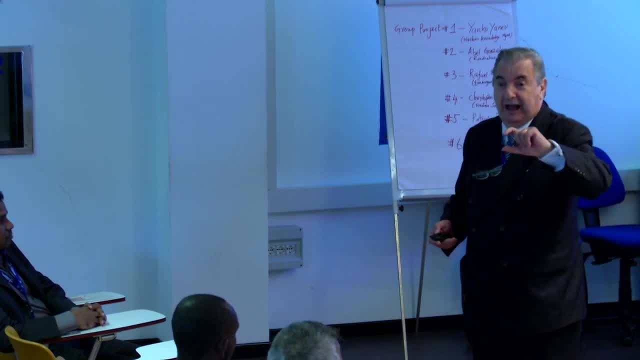 The doctors usually tell to you: don't have a CT, have an MRI, because the MRI is with no ionizing radiation. Well, when you go to have an MRI, all the hydrogen atoms in your body start to oscillate like that. 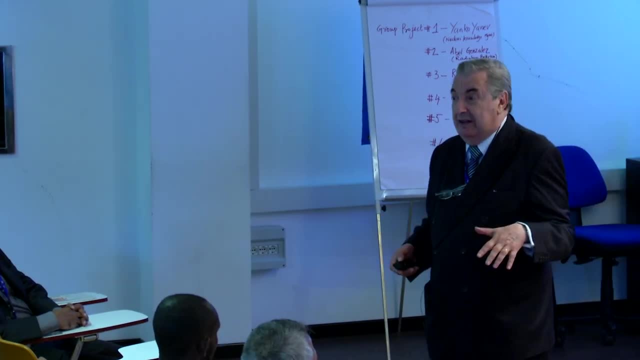 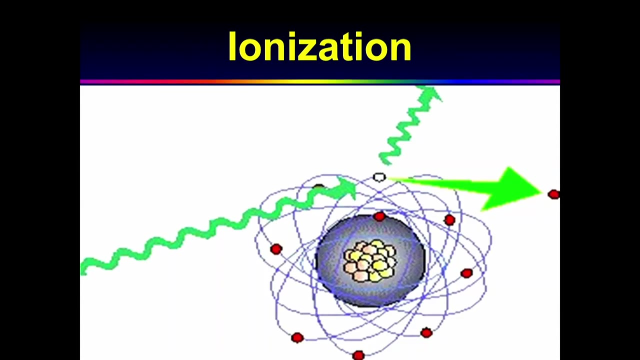 Well, this is producing effect that nobody knows. With the radiation, we know the effect that it produce And we will talk about that. Ionization means that radiation has enough energy to take electrons out of the atoms in your body for exchanging the atoms in your body. 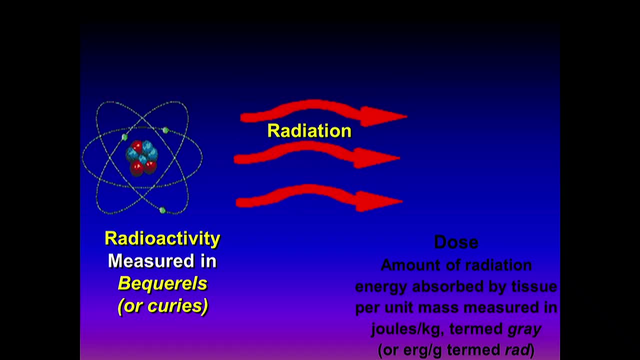 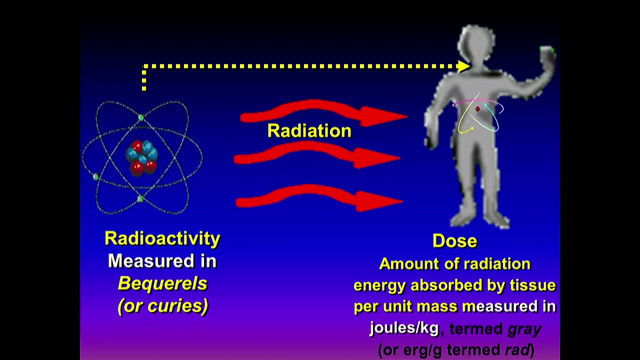 Therefore you have radioactivity measured in becquerels, radiation a person, radioactivity that goes inside the person or outside, And those there is. the amount of radiation of energy absorbed by tissue per unit mass is measured in joules per gray, which are units of energy in joules per kilo units. 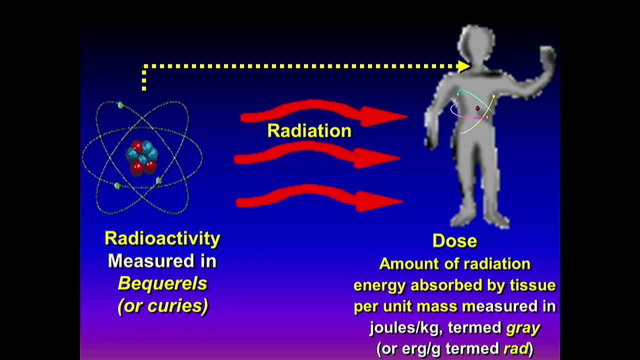 of energy and mass is termed gray All around the world, except in one country where it's measured in erg per gram and termed rough, And again, that country is the United States, Or only this is already a big source of confusion. 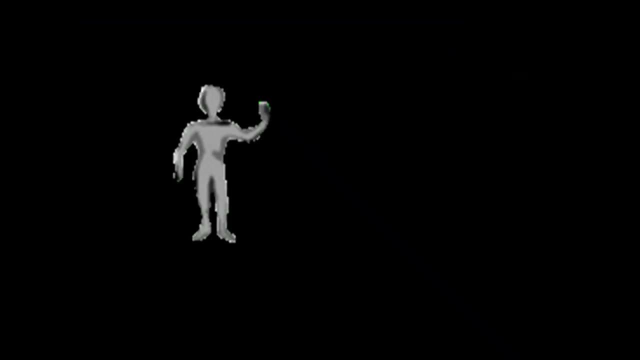 Okay. Therefore, you have a person here can get radioactivity inside because have irradiated from inside, can get radiation from outside and he get absorb those measured in gray or rough. Finish the problem. No, Unfortunately it's not finished. 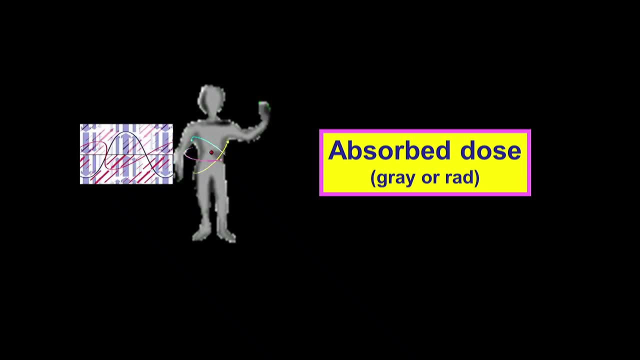 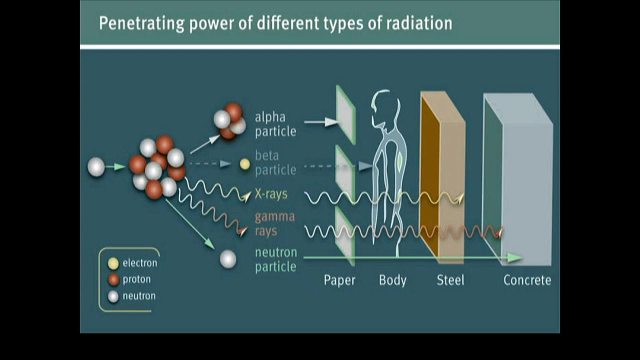 Why? Because the harm do not depend only of the energy absorbed per gram or per mass, but depend also of the type of radiation. Why? Because different radiation have different penetrations. Alphas- you can stop with the paper, you stop the alphas. 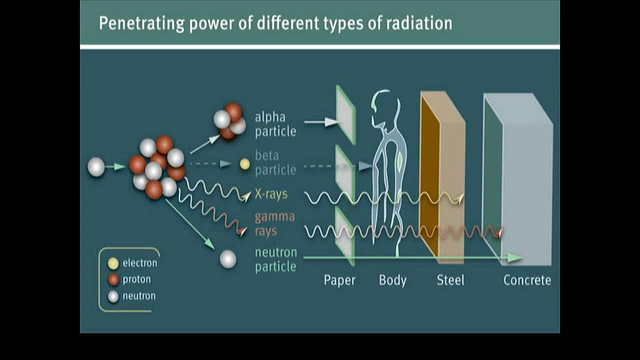 Betas go a little more. Gammas penetrate everything. Therefore, you say: okay, in that case alpha is not a problem. It's true, It's not a problem If the alpha is outside. now, if the alpha is inside, ah, it's a big problem. 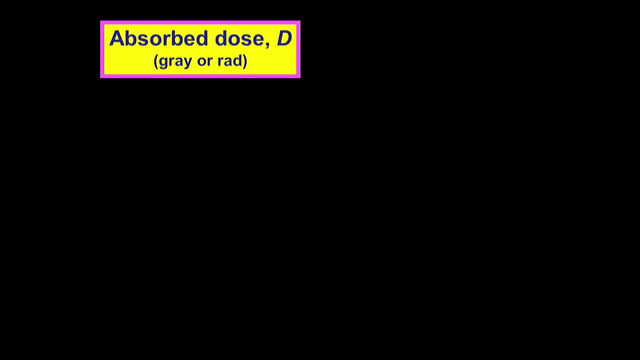 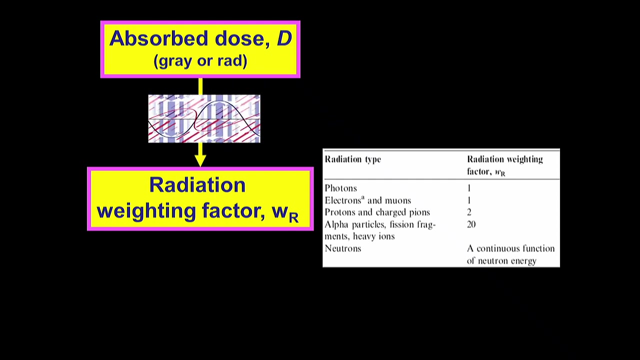 Therefore, to consider this, the absorb, those have to be weighted with factors which depend of the type of radiation. The weighting factors that you can see there is usually one for electrons or proton, but for alphas it's different. For alpha 20 times more dangerous because of the properties of the alpha. 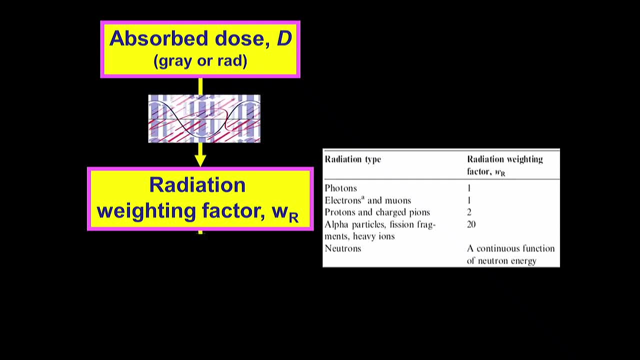 And the result of the weighting absorb those within this weighting factor is called equivalent dose, For in every part of our body, in every organ, we can measure this equivalent dose weighted, weighted, absorb dose. The quantity used. the unit used for this equivalent dose is the sievert. 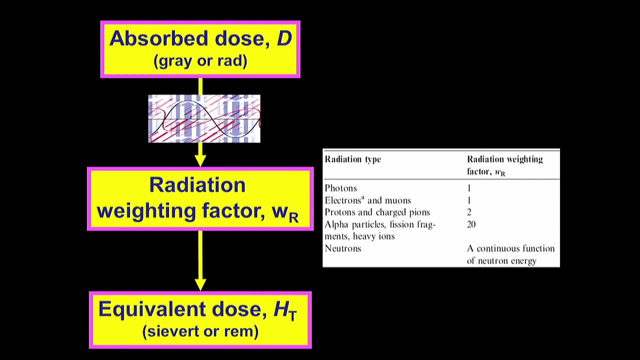 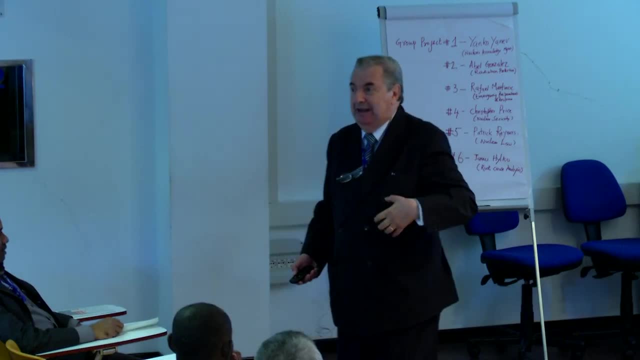 All around the world, except in one country which is used at the REM. The country, yes, is the United States. The issue is finished here. No, Why? Because, in addition, that different radiation produce different harms in an organ different. 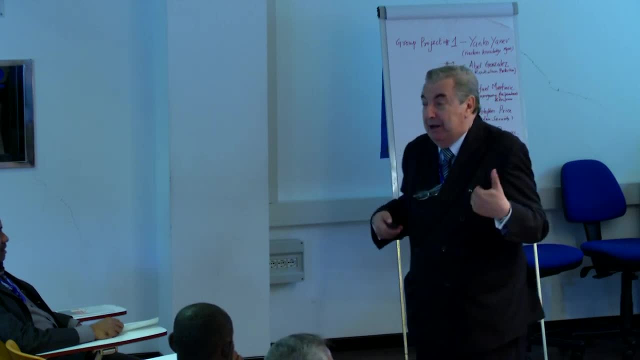 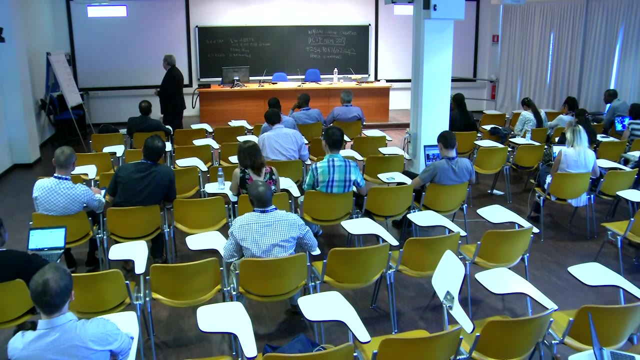 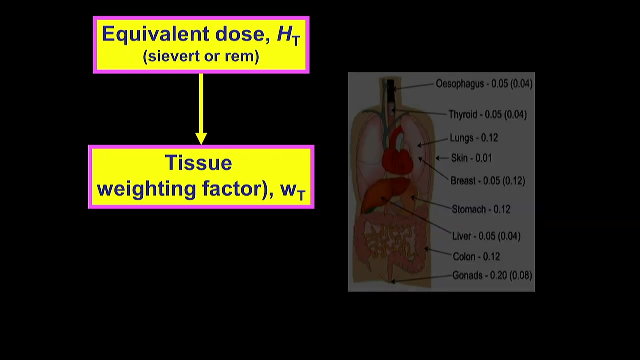 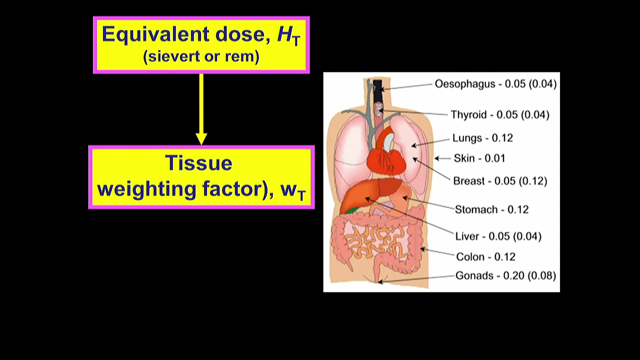 organs produce different harm because every organ has different radiosensitivity to radiation. For we need to weight this again, this equivalent dose by a tissue weighting factor. Here there are the tissues weighting factor. in parentheses are the old numbers which you can see give a little the idea of how sensitivity sensitivity is a tissue to the 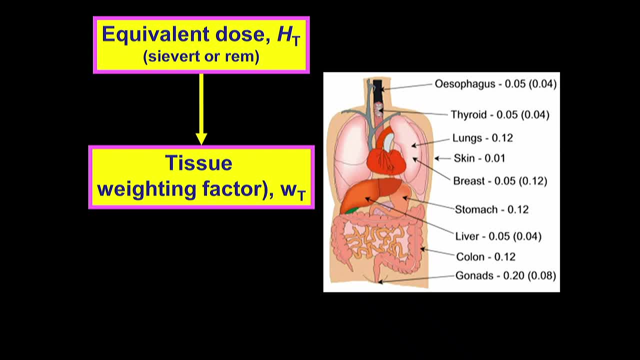 radiation, For instance, stomach and colon and lung is very sensitive, but thyroid is very. the sensitivity is very little And this is important for what we are going to see. The result of equivalent dose weighted by a tissue factor is called effective dose. 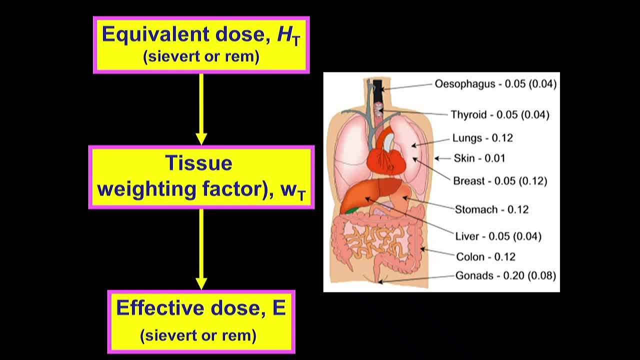 Big problem. The effective dose is measured in the same unit that the equivalent dose. First problem, therefore, is when you as appear in the newspapers, that the people receive so many sievers. First question is: sievers, equivalent dose or effective dose? 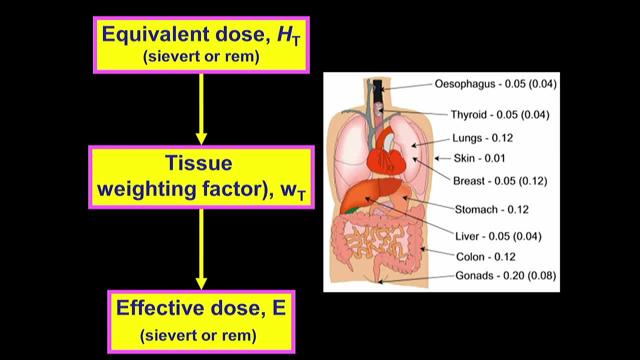 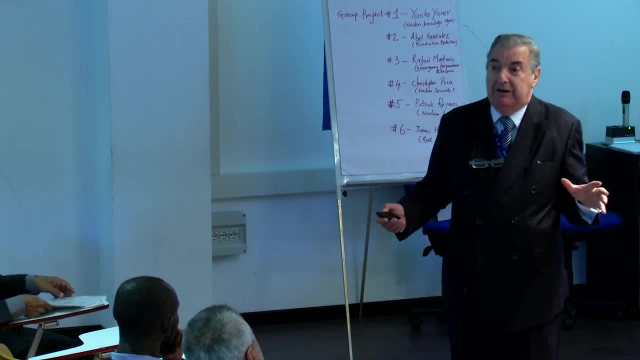 Believe it or not. this was a serious problem in Japan because in a press conference, the prime minister was asked about the doses of due to iodine. People are always concerned with iodine And the prime minister said: well, I am here. 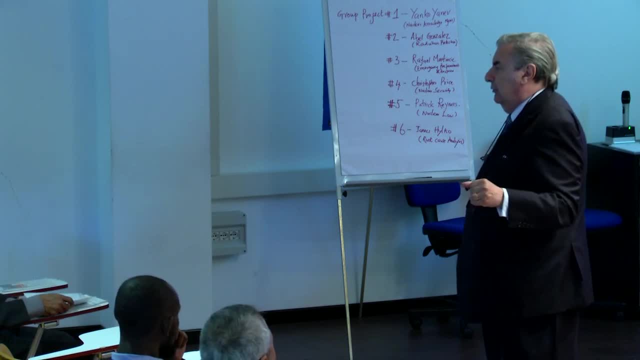 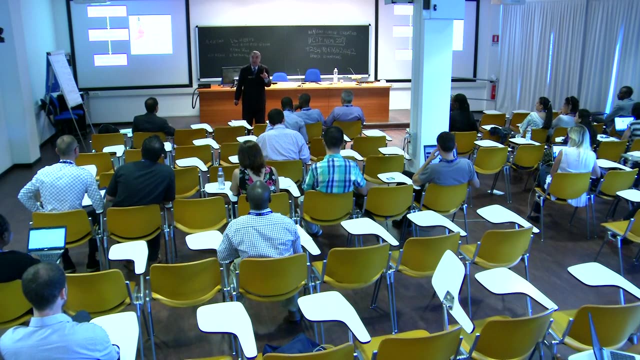 He said: well, I am informed that the doses are not so high, at around 100 millisieverts. And one fellow in the media, because the media now is very well informed, better than the Chinese sometimes, he said, prime minister, is 100 millisieverts of equivalent dose or? 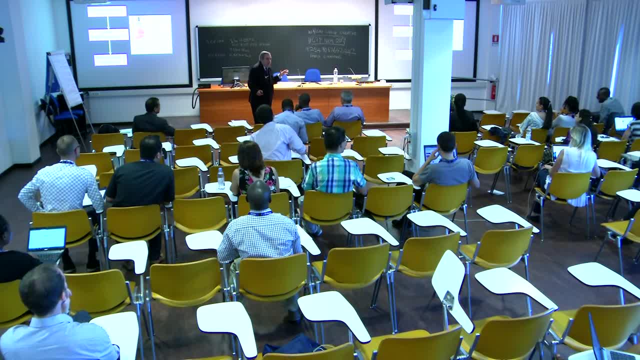 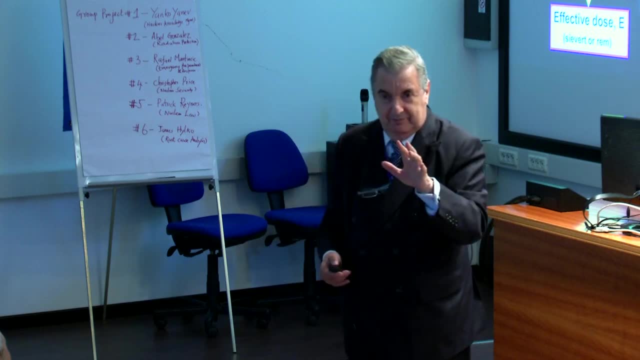 effective dose. The prime minister have not a clue, All the people around the prime minister have not a clue And they lose credibility in one second. And when you lose credibility, Forget it. You don't recover so much And the difference is dramatic because 100 millisieverts of equivalent dose in thyroid 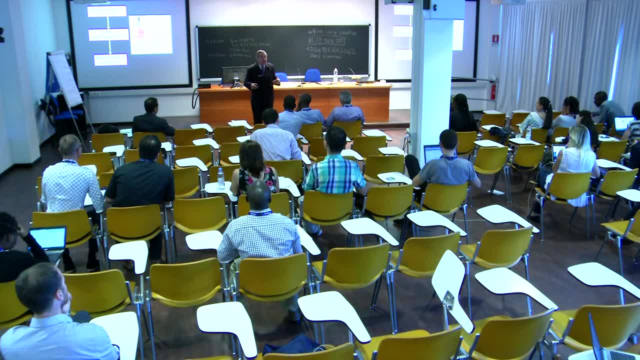 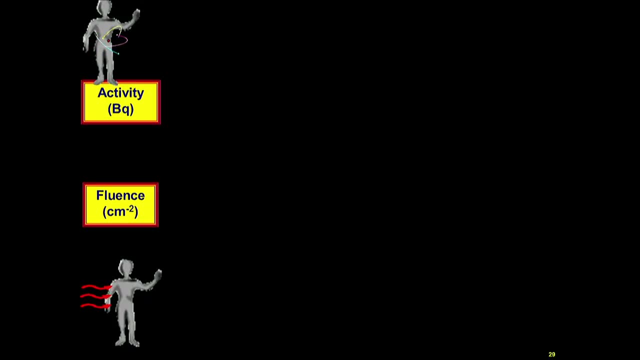 is not so bad, But 100 millisieverts of effective dose means that the thyroid has received an enormous dose because, as you see, the weighting factor of thyroid is very small. OK, In summary, what do you have to know? Activity inside, fluence of particles outside, absorbed dose to people. weighting equivalent. 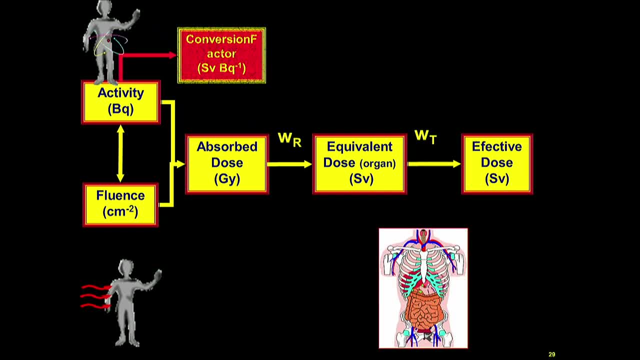 dose in the organ weighting effective dose in the body. The good news is that there are convention factors to convert activity in equivalent dose and effective dose, or amount of radiation in equivalent dose and effective dose, And these factors have been calculated For a standard people and are in international standards. 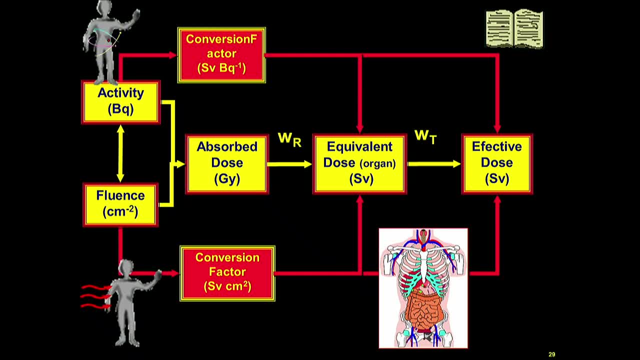 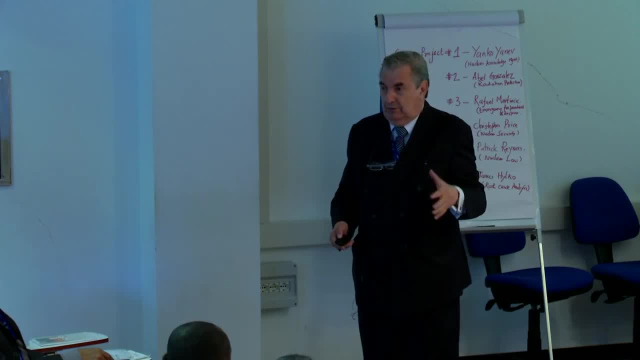 But this is important: that you, as a manager, you know this structure, Otherwise you can get in very big confusion. People normally talk about dose. You can say what dose. It's absorbed dose, equivalent dose, effective dose- a lot of different quantities. 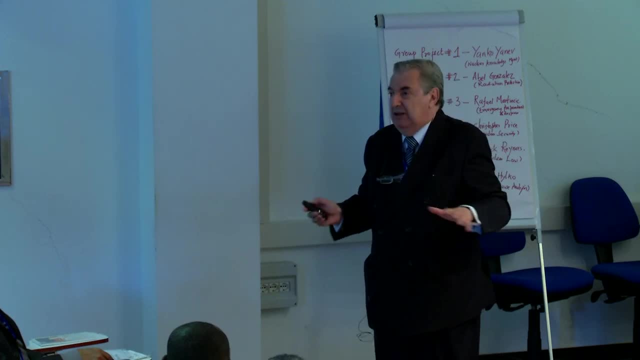 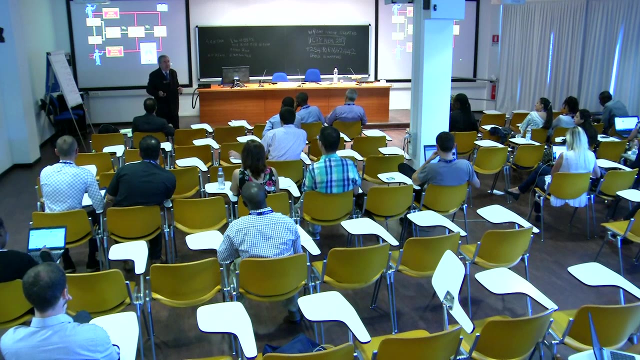 Why we have created such a complicated system. I don't know History, History, You know. you build a house by pieces and the house became chaos. This should be changed. Yes, In my opinion. yes. We wrote a report after Fukushima and we said: this is the need that somebody shake the coconut. 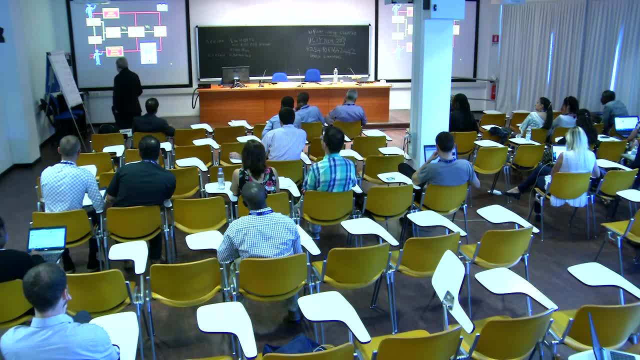 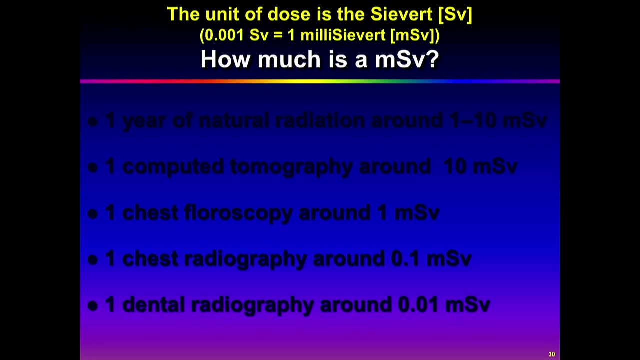 tree of the system Because it's very complicated and very confusing. The unit of the dose is the sievert. Opposite to the becquerel, the sievert is a very big amount. One sievert is a lot of dose. 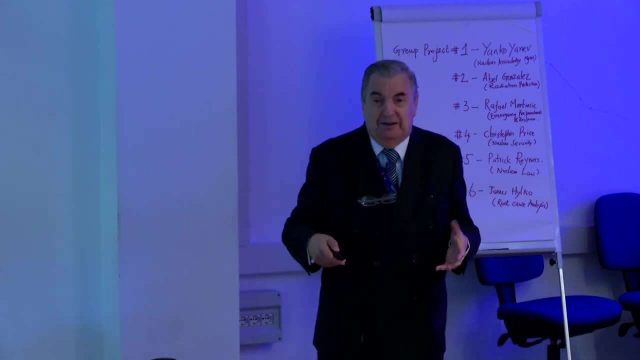 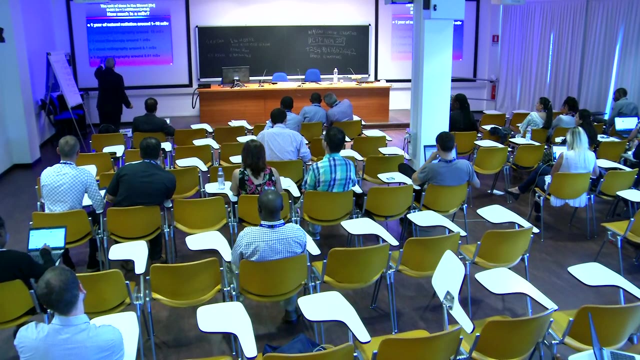 For that reason, we normally talk of millisieverts, a millesima of sievert. What is a millisievert? Well, order of magnitude, One year of natural radiation is around 1 to 10 millisieverts, depending on what you live. 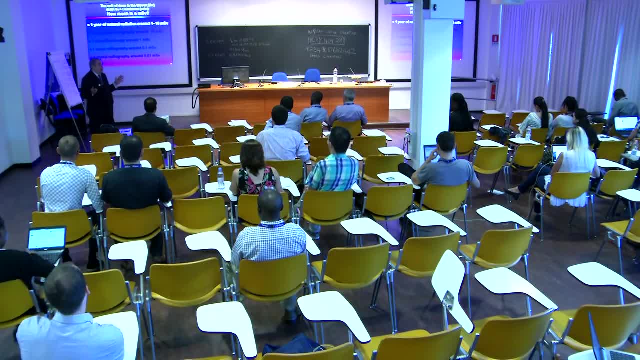 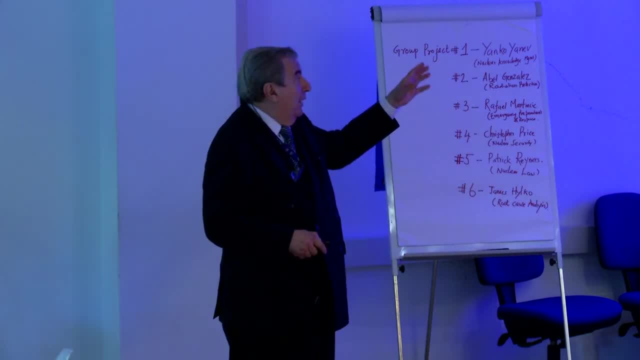 It can be much higher. If you are from Kerala in India, you will receive much more than this Or other places. you will see it. One computer tomography- you probably have one in your room. You arrive, I don't know. 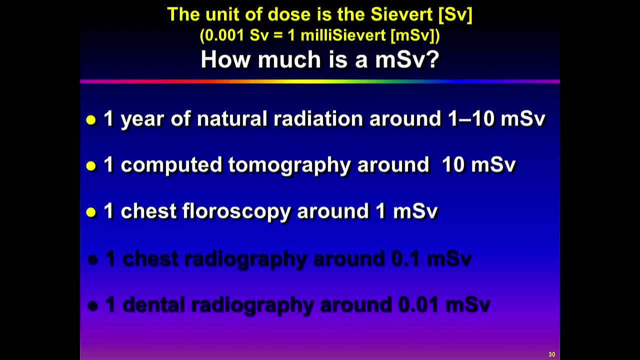 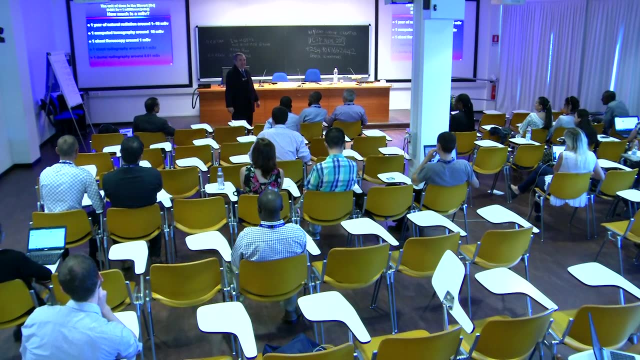 You get 10 millisieverts with a computer tomography. Yes, You are right, It's a unit of effective dose. Very good comment. Very good comment: It's a unit of effective dose. What you are talking here is effective dose. 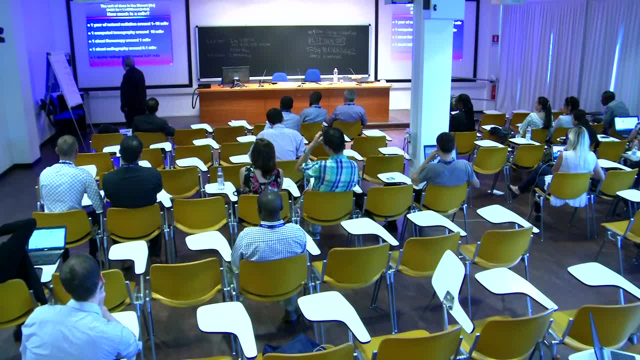 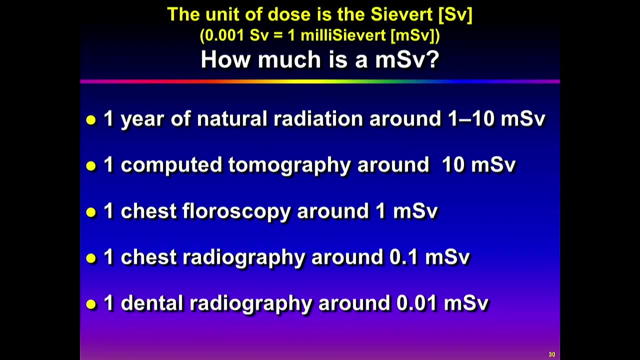 One chance fluoroscopy: around 1 millisievert. One chance radiography with good equipment: 0.1.. Good equipment of dental radiography, very low dose. The old equipment was a disaster, by the way, But the new equipment is not like that. 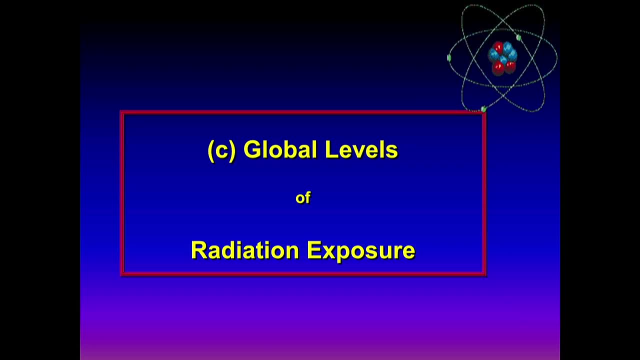 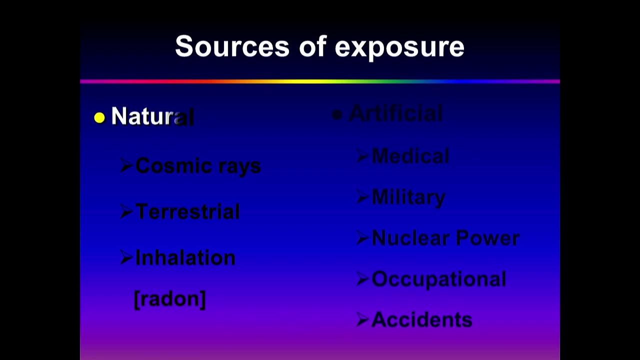 Okay, Let's talk about the global levels of radiation exposure. First of all, what are the sources? The sources are natural cosmic ray, terrestrial radiation, that is, on Earth, Inhalation of a gas ray, and we will talk about that. 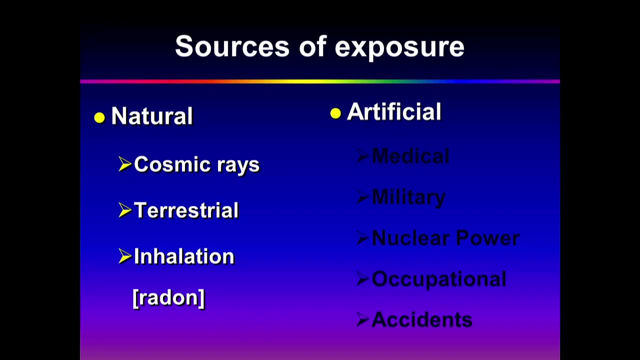 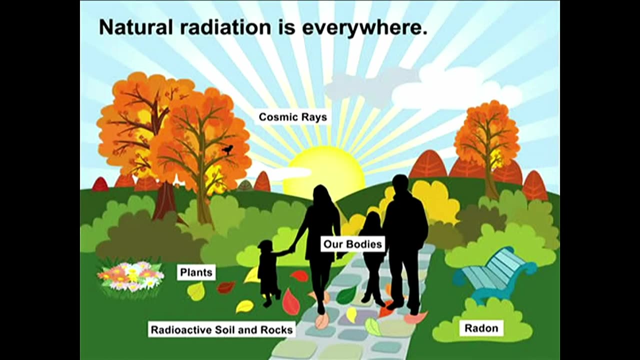 Or artificial, created by man, Medical, military, and we always forget about this. Nuclear power big problem, Occupational workers with radiation And accidents, Natural. well, radiation is everywhere, Cosmic rays in our bodies, in the soils. 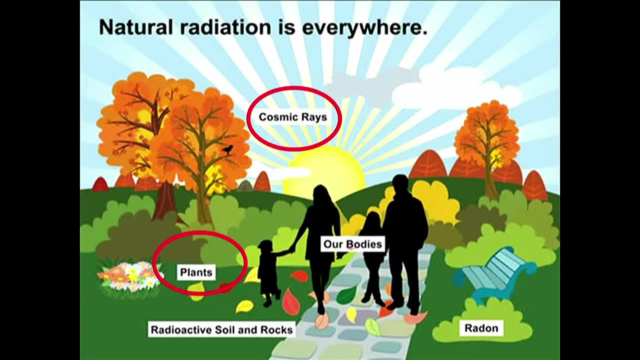 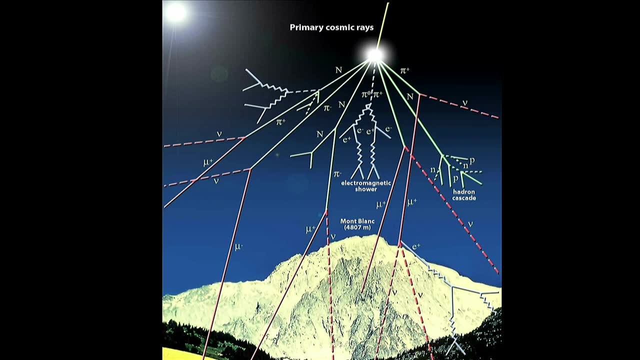 Cosmic rays are produced in some place in the universe. Nobody knows where. There are several theories: Stars will explode, But what we know is our Earth is bombarded with cosmic rays. They arrive in the high atmosphere. They interact with the atmosphere. Fortunately the atmosphere is there, Otherwise they will kill us And there is disintegrate in a lot of particles. Depends where you live. you get more or less cosmic rays. If you live in La Paz, which is the capital of Bolivia, you get a lot. Because, La Paz, the Spanish have the good idea of found a capital of 4,000 meters. If you fly a lot like me, you get a lot of cosmic rays. If you live in the Antarctic, you get more than if you live in the equator. 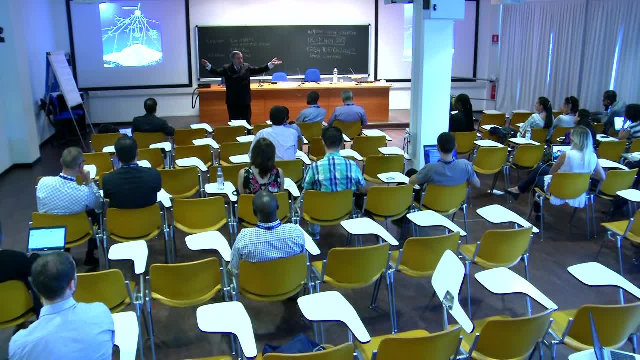 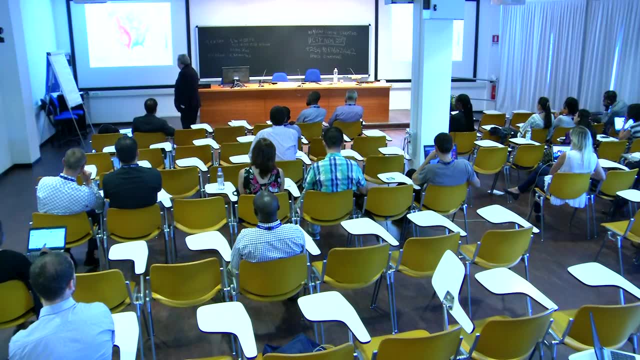 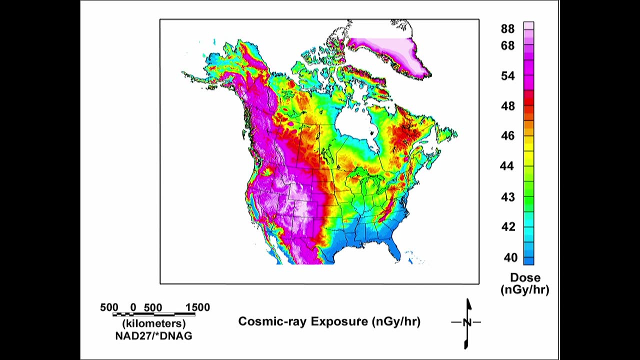 because the cosmic, by the magnetic field of the energy go to the Antarctic, For instance. if you live in the United States- depends where you live- you have different levels of cosmic rays. Here in Miami, in Florida, nothing. Here in the mountains a lot. 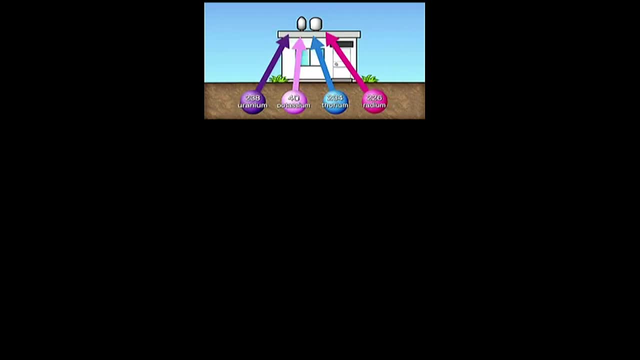 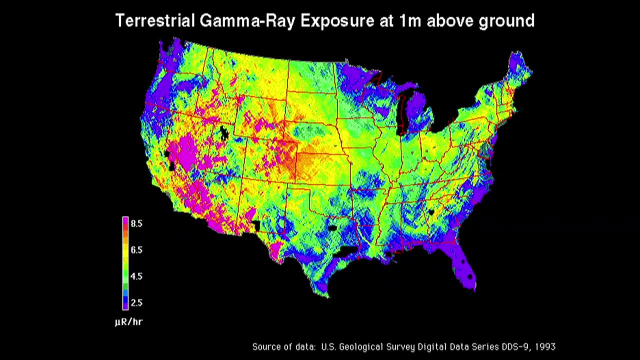 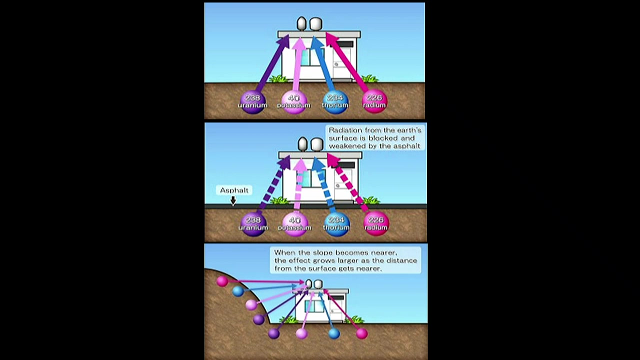 Then you have the radioactivity in Earth. There are several nuclides And again depends where you live. you get different. For instance, if your home is near a mountain, well, you get radioactivity from the bottom and also from the mountain. 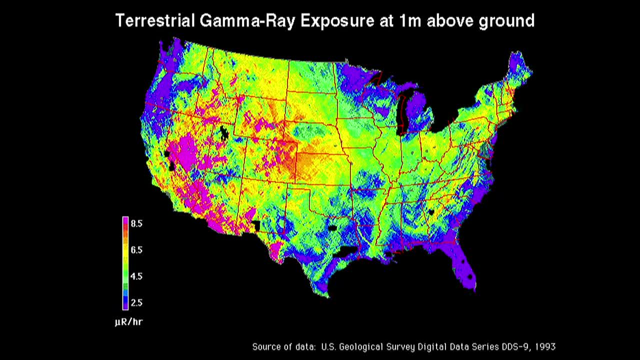 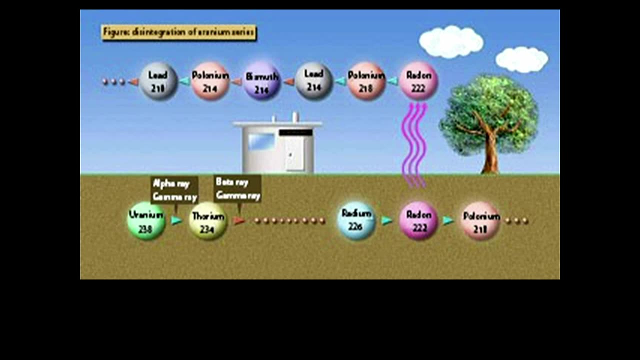 Again, the example of US Depends where you live. If you live in Florida, very low, because there are very low radioactive material in soil. If you live here in the mountains, much bigger On Earth. there is one nuclide particularly nasty. 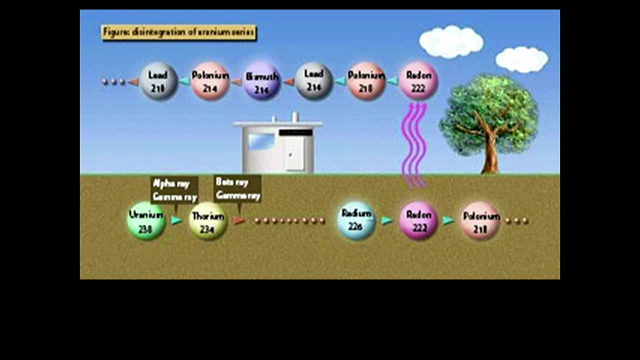 Radium and which decay to radon. Radon is a gas, But it's a noble gas. But in principle, if you annihilate radon, it doesn't get in your body, Go out, But while it's in your lung, radon decay. 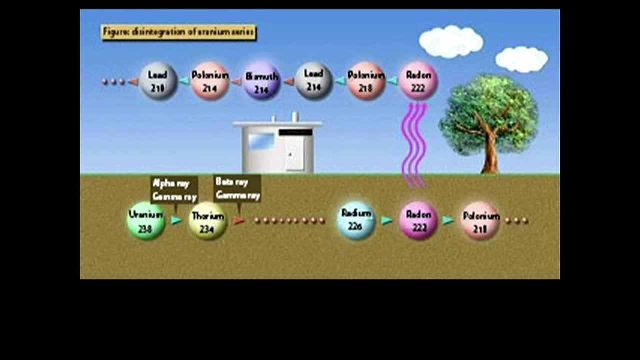 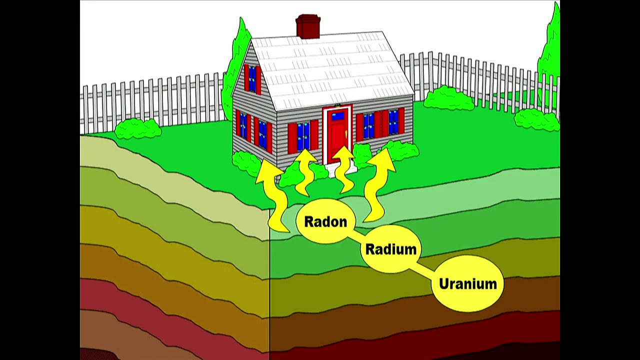 And what we call the daughters of radon. the decay products are very dangerous for your lung, These nasty nuclides, we will talk about them For radon, which is coming from the uranium, which decay to radium, to radon. 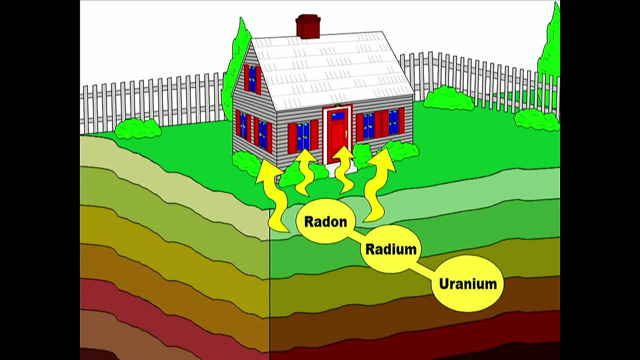 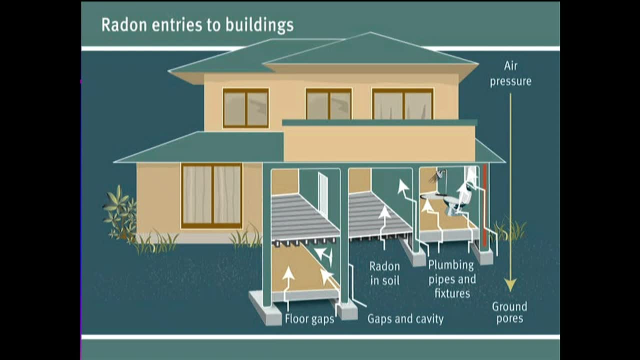 go into your homes And irradiate you from your home Depends where you live. again, If you live here in Europe, in the north particularly, the homes are like this: Radon go from the gaps in the keller, go up from the plumbis. 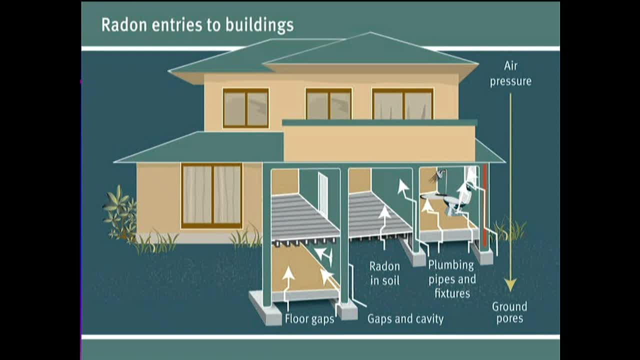 This home has very good windows, for there is no ventilation and radon accumulates. If you live in my country, you have no that problem because our windows are so bad that you know air is entering from everywhere and etc. 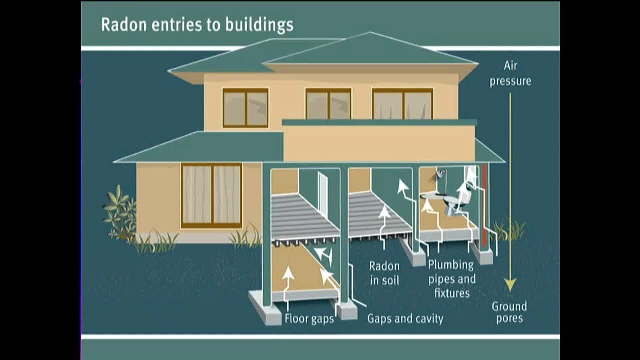 The homes are very well ventilated and we don't have a lot of radon. In addition, we don't have too much in the soil. But in Europe it's a serious problem, Serious problem, Particularly in the north. In the US also it's a problem. 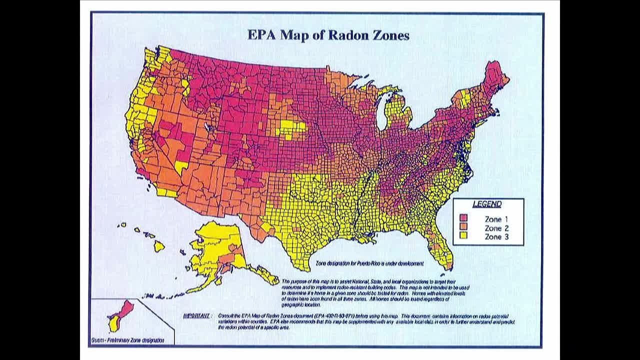 In these areas where there is a lot of uranium, you have radon. Again, in Miami, they have no radon. I can imagine that you try to move to Miami now, you know, because there is no radon. no this, no that. 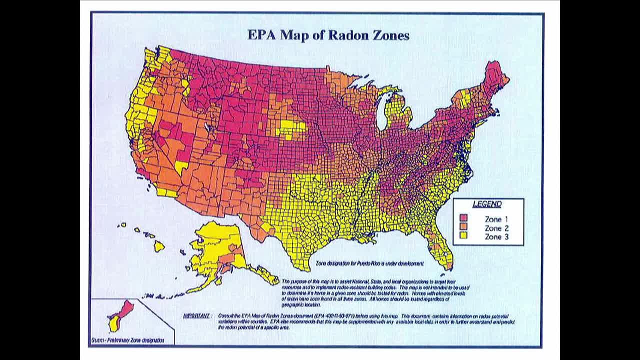 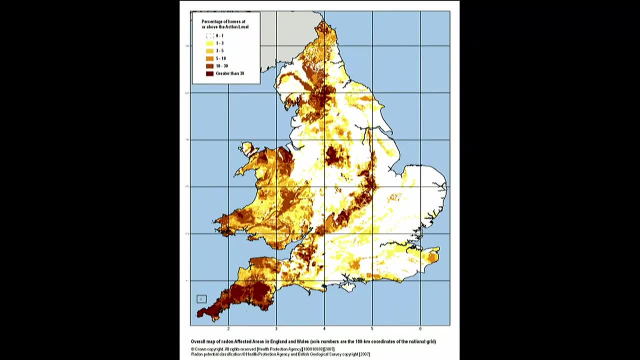 In addition, you can speak Spanish fluently in Miami without any problem. I mean, if you can make a problem, if you only manage English, you can have a problem In England. it's very interesting: England has very low radiation. 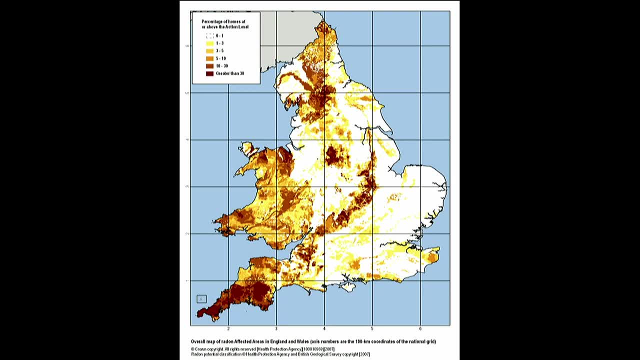 except in this part, in Cornwall. Well, the Cornish people will be furious that I said that they are English, you know, because they believe they are Cornish, not English. But here in Cornwall the level of radon is very, very high. 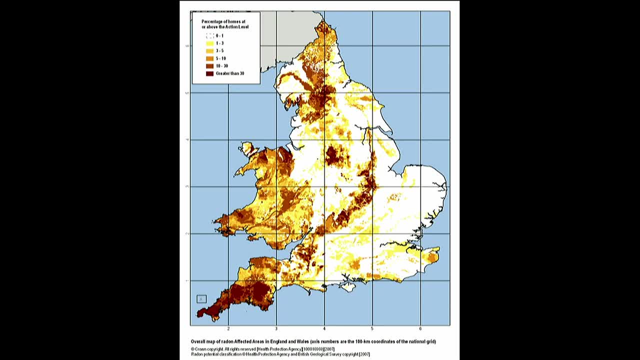 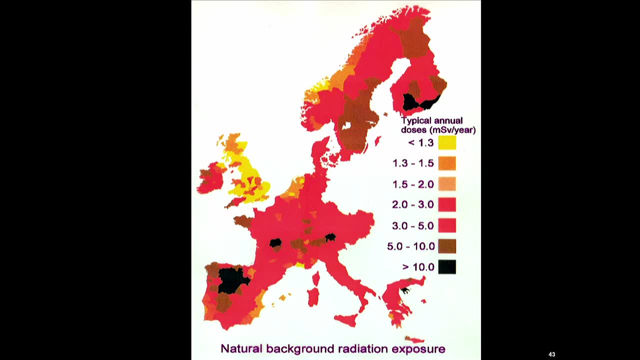 Enormously high For big difference. in England And in all Europe there are big changes. you know Depends where you live. If you live in the north of Spain, in the massive central, not far from here, in France, in Austin, in Finland, 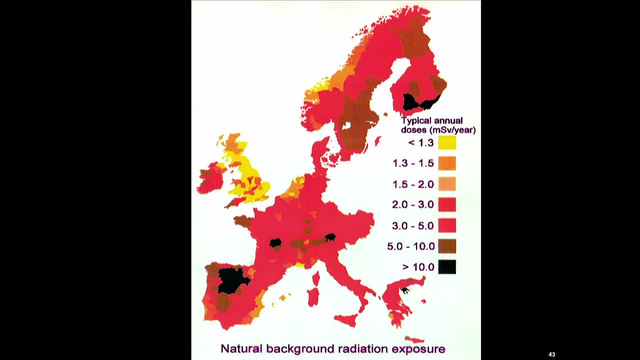 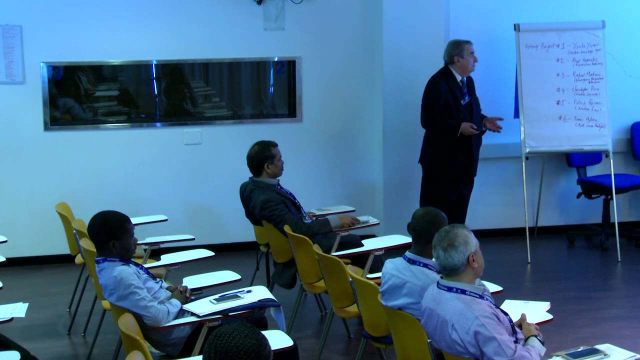 the natural radiation can be very high, more than 10.. If you live in England, it's very low, less than 1.. But depending where you live, it changes a lot. All over the world it changes a lot, For I try to summarize this changing in the following way: The value of natural radiation goes from 1 to 100, approximately. You cannot have less than 1.. Even if you live in a remote island in the Pacific, in the middle of the Pacific, you will have a little more than 1 of radiation. 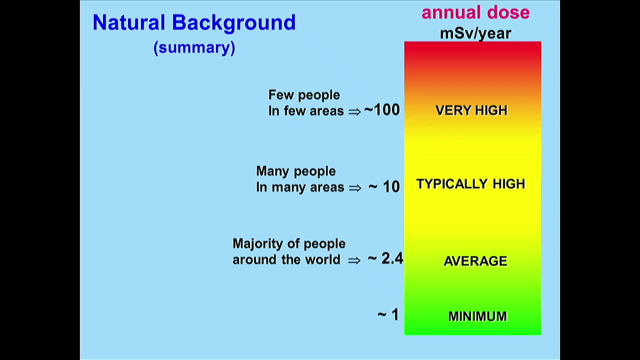 Few people in few areas get more than 100.. Many people in many areas around 10.. The majority of people around the world. the average is 2.4.. This gives you a feeling of the radiation that we receive. This is important. There are areas with very high level of natural radiation. For instance, one beautiful city in Iran, Ramsar, has levels up to 260 millisieverts. Why? Because they have water coming from the travertine, water full of radium. 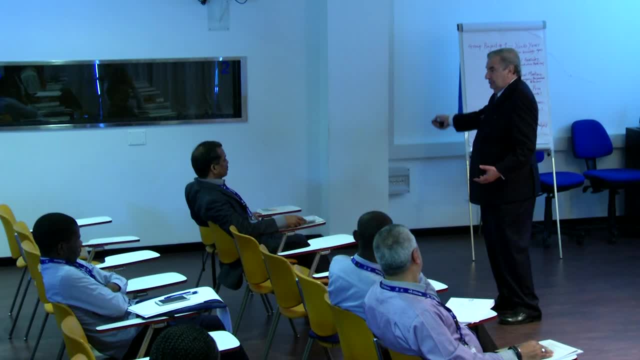 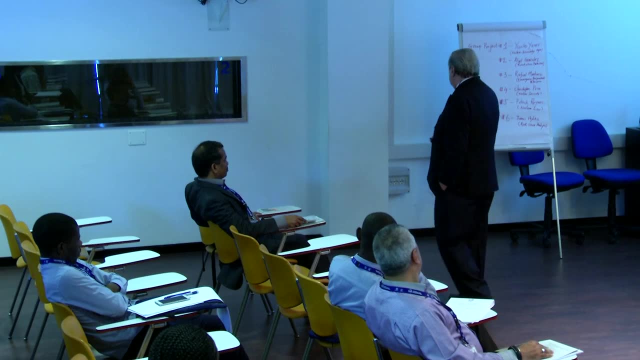 And they have used this water to build their homes, to make concrete, For the homes are really big irradiators, Not all Ramsar but a big part of Ramsar. Then in Kerala, in India, the south of Kerala, Kerala is beautiful. 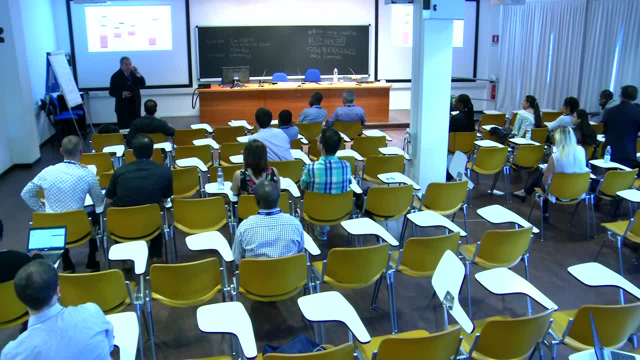 Kera means coco and Kerala coconut, And Kerala is a forest of coconuts. It's a beautiful area, But in the soil there are thorium in the part of Kerala. Due to that, the radiation is relatively high. 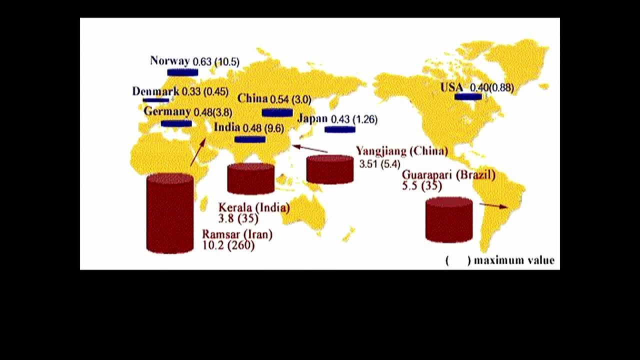 It can be around 30,, the maximum 35. The average is 3.8.. And there are areas in China, in Brazil, Brazil, the beaches we go there, beautiful beaches that contain a lot of thorium. Well then, we have the medical sources. 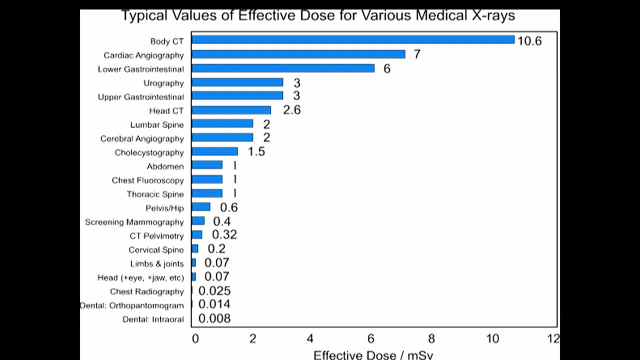 These change very much depending on the procedure that you do. The body CT is 10, up to the dentals that are very low. Angiography is 7.. Gastrointestinal is 6.. Depending on the procedure, it goes between very little up to 10.. 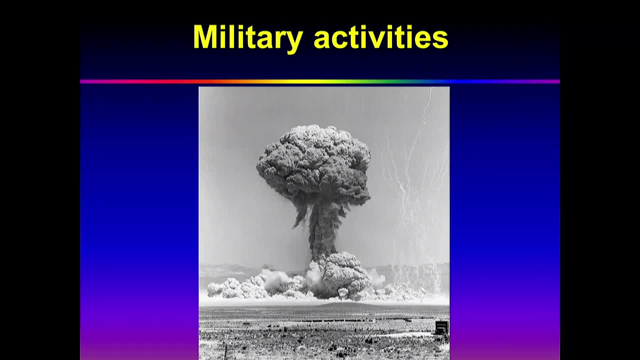 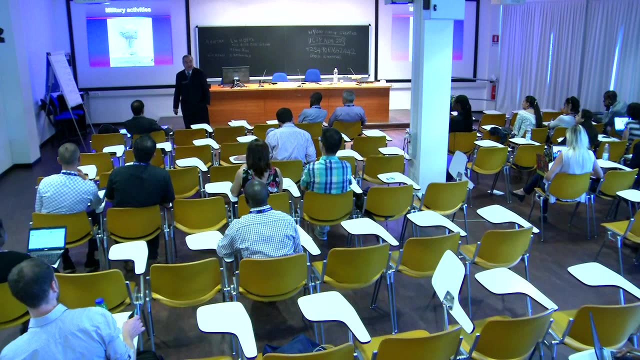 And the military. Well, we forget about the military activity And well, I don't want to make a joke that we used to make in Argentina with the five powers- you know, the five powers- recognized power of nuclear weapons that can make thousands of nuclear weapons explosion. 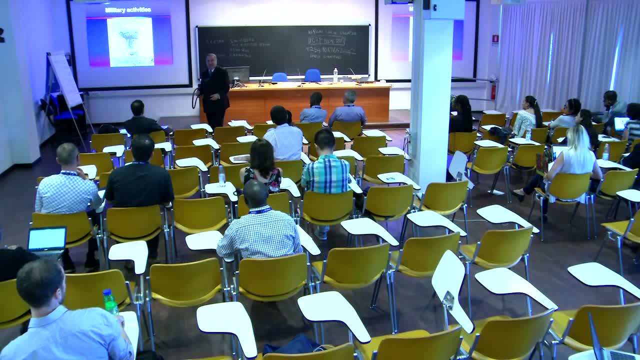 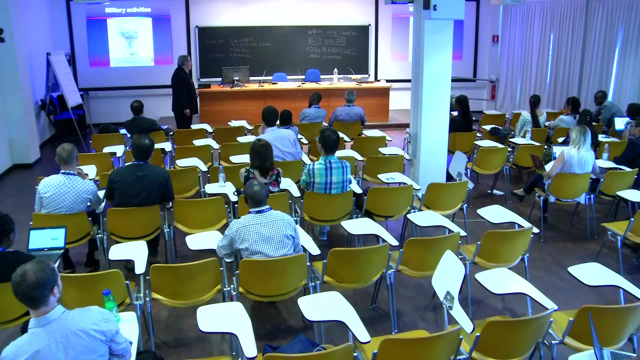 And we were very concerned, you know, on India, on Pakistan, And we used to say that these five powers are like five prostitutes, which are very concerned because they saw a nun being scared, And anyway, these powers have produced a lot of explosions. 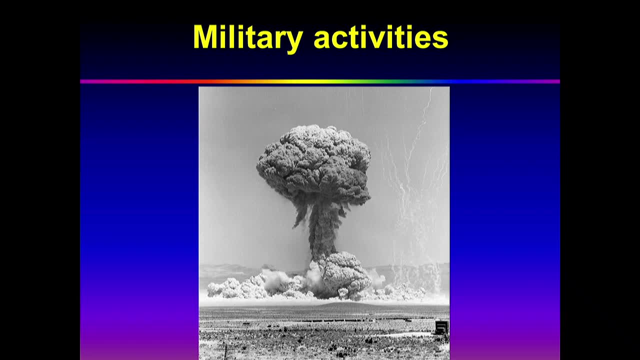 in the atmosphere, sending radioactive material all over the world, Radiative material that we still have in our bodies. If you measure yourself in the whole body count, you will see cesium in your body coming from a nuclear explosion. Moreover, if you're in the North Hemisphere, 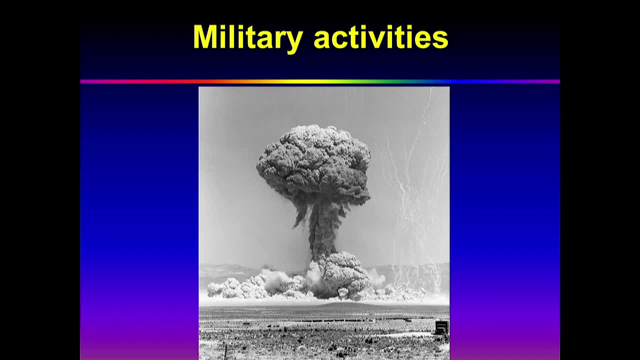 you will have more cesium than if you're in the South Hemisphere, Because the radioactivity put in the atmosphere do not mix the hemispheres And since in the North Hemisphere were much more explosions than in the South, in the South were only the French. 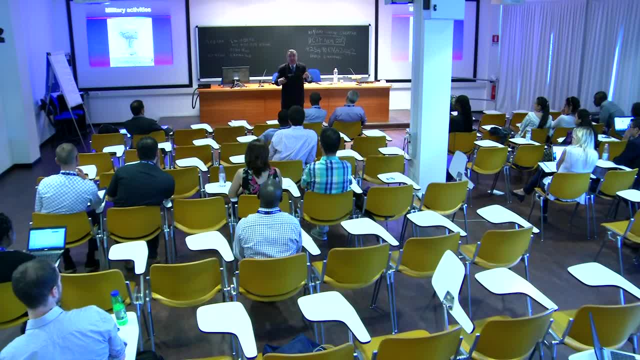 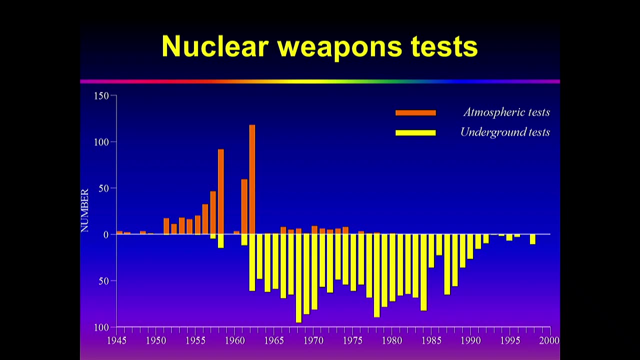 and the British in Australia, But in the North the Americans and the Russians and boom, boom, boom, one after the other, thousands of explosions. You can see here the problem, particularly in the 60s, you know, only in the 62, I believe that was. 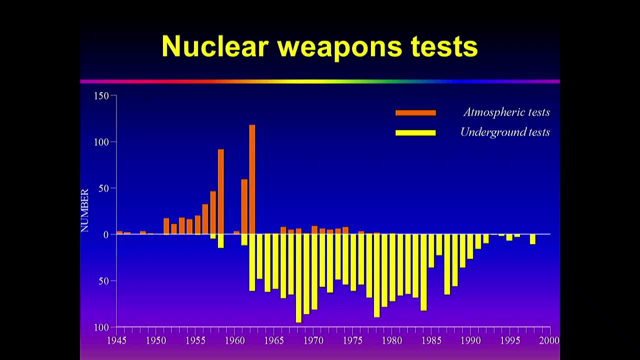 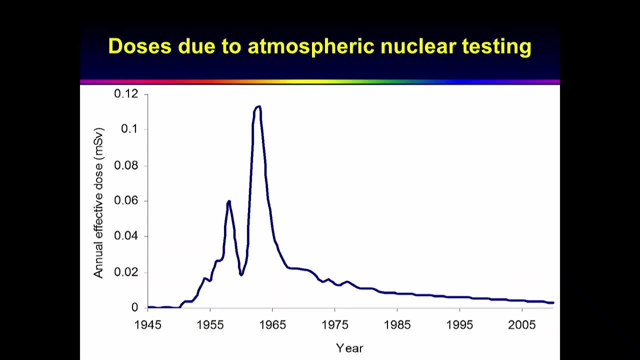 there were more than 100 explosions in the atmosphere. The yellow is an explosion underground, which of course is not distributed material. but you know, you have a lot of radioactivity underground and sooner or later it goes to the medium as well. 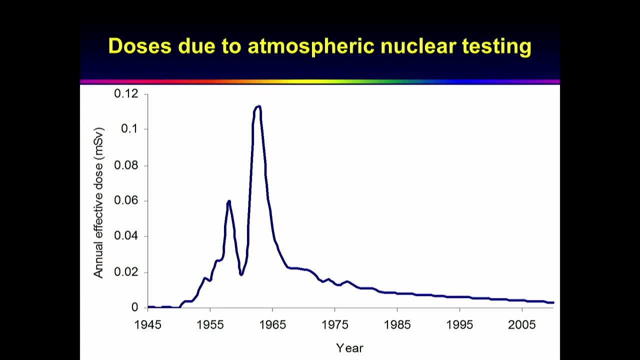 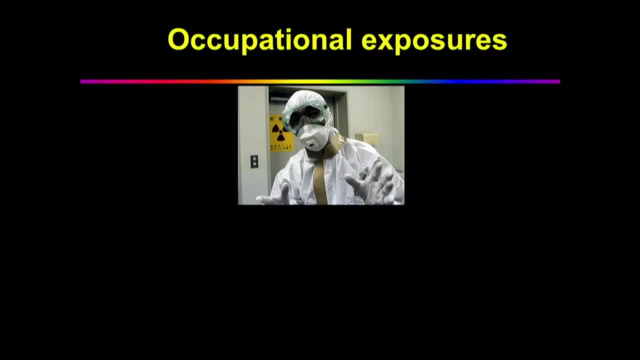 And the dose due to that were moving on the Earth in the 60s was a very big peak, depends where you live it and now it's a little lower Occupation workers. Of course, everybody said, well, the real problem is this fellow. 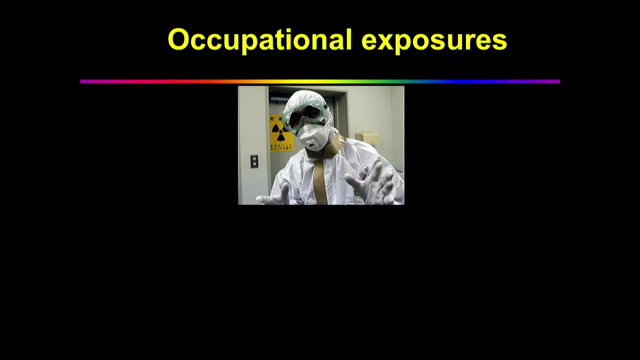 you know, this is a nuclear operator, Nuclear operator with a mask, with protection, with a special suit. My goodness, this fellow is in real danger. The reality is a little different. Apart from this fellow, you have medical doctors and you have pilots. 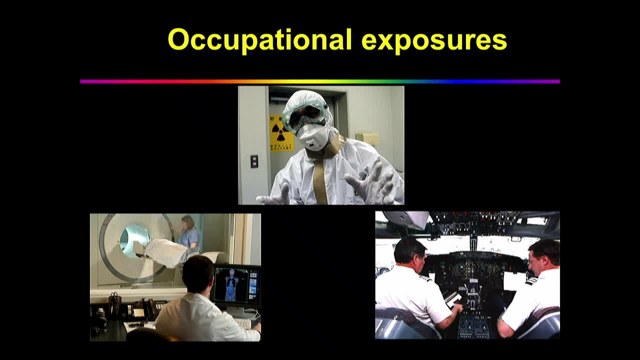 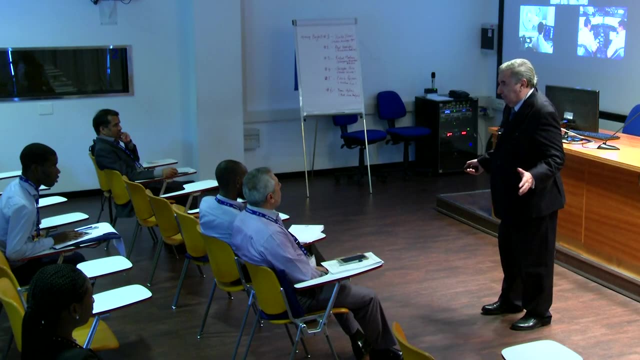 and they still were there. Well, believe it or not, something very few people know, the people who received the highest dose due to his work are pilots, Due to COSMIC, And you cannot stop those because you cannot shield the plane. 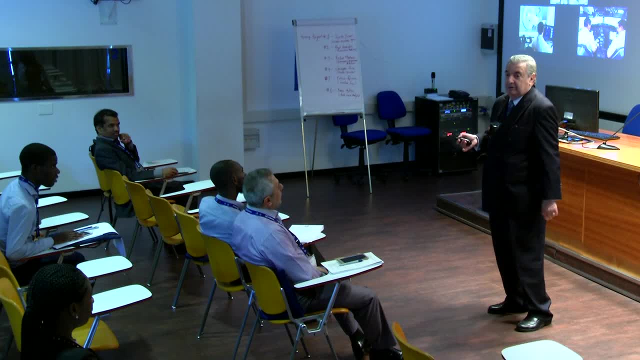 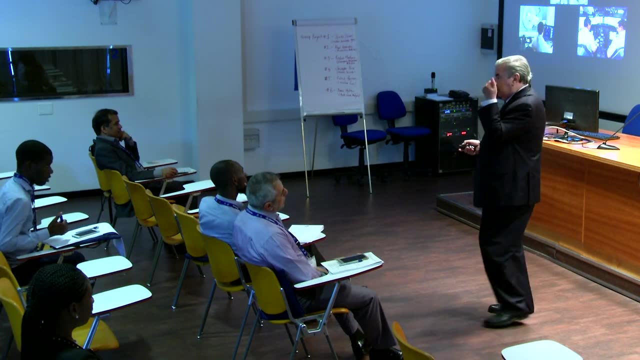 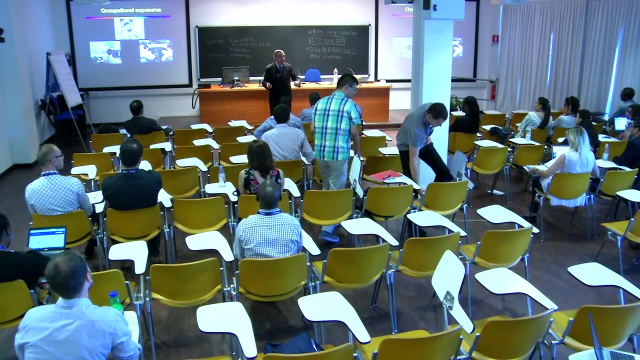 You cannot fly low. The only thing that you can do is to remove the crews from one position to the other. but the crews doesn't want that because they lose money. Argentine Airlines is one very serious affected airline because we fly the South Polo. 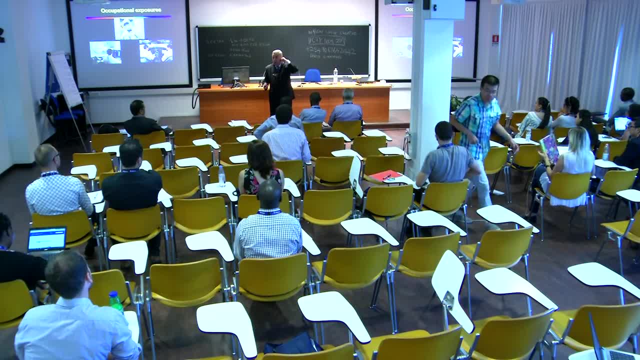 Also fly to the North, because we fly to the North And we try that the crews were changed from the South Polo to No the crews. no, no, no. I want to go via the South Polo because I go to Australia. 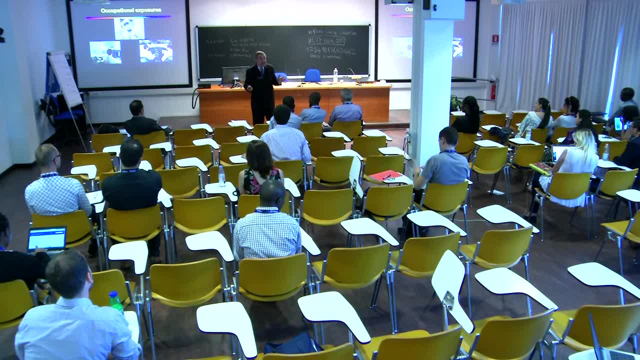 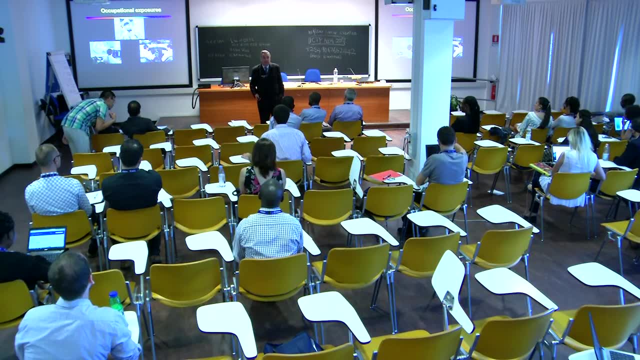 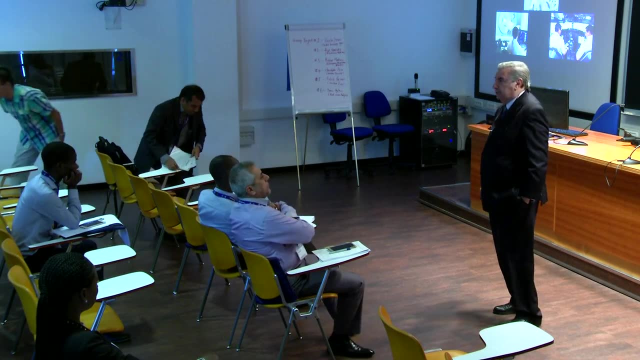 I go to New Zealand. I get more money. it's very nice, It's complicated And the doctors, particularly the interventional doctors, get also very high doses. It's not the work of a nuclear power plant. the more exposed person. 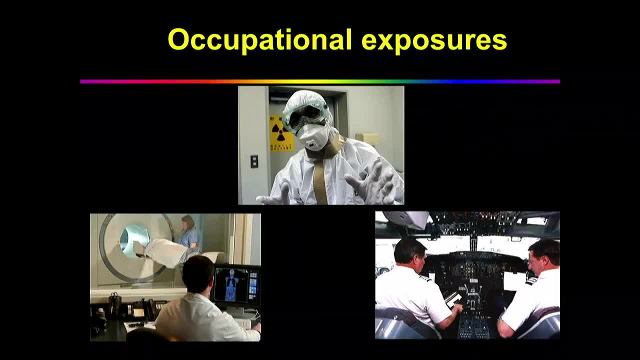 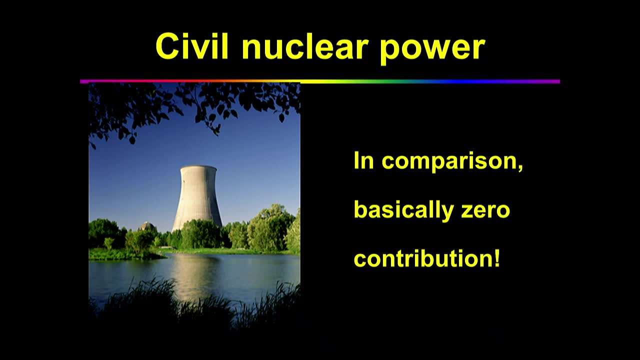 They are pilots- Pilots and stewardess, by the way- And civil nuclear power plants, which is our concern, the reason that you are here, the reason of all the paraphernalia of international standards and regime. basically, zero Radiation from nuclear power. 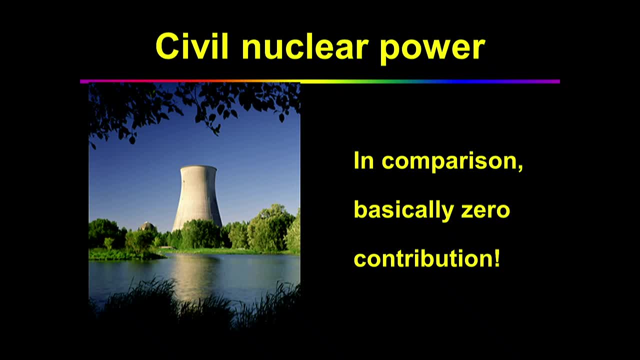 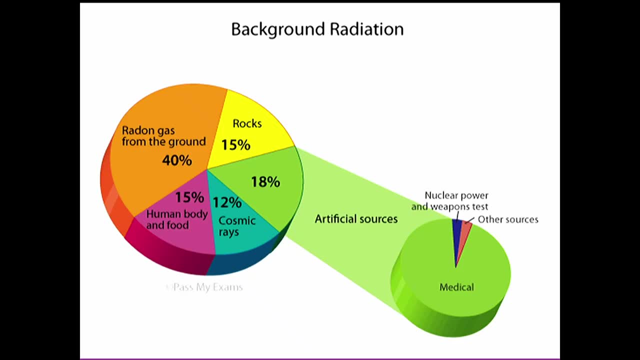 is basically zero, For that is the problem: that we have A completely different perception. In summary, look, the pipe of radiation in the world is a natural carry. the more part of human exposure Rocks radon, the one that we have in the human body. 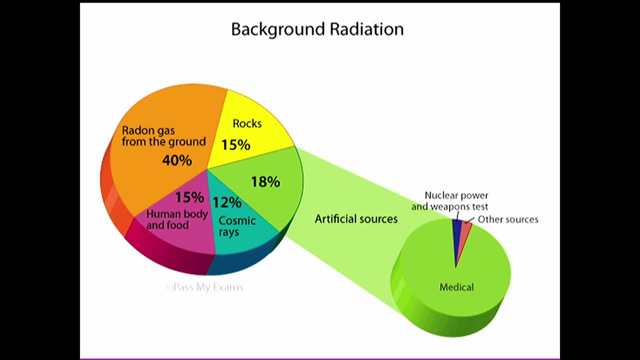 that we needed cosmic rays. The artificial is only 18% in the world And of these artificial, the majority is medical. The rest is basically nothing. The perception of people is exactly the opposite. You can check in your home with your relative. 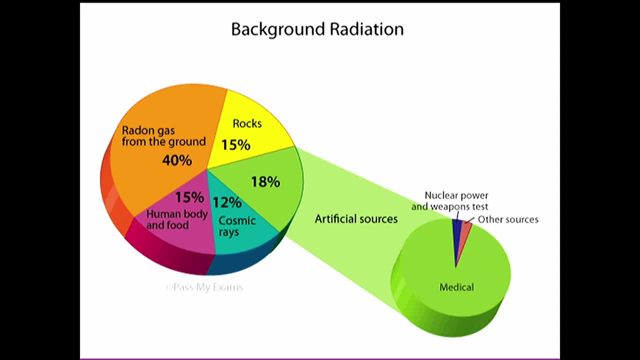 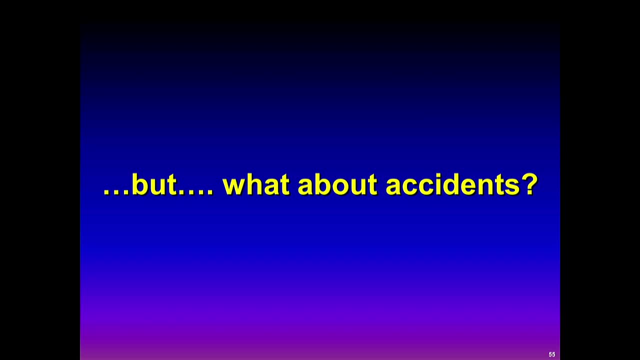 you said to them this and they say, no, you're lying, It's not true. But people, people who really know this, say: ah, but what about accident? You are not saying the full truth Because, in addition to the normal operations, 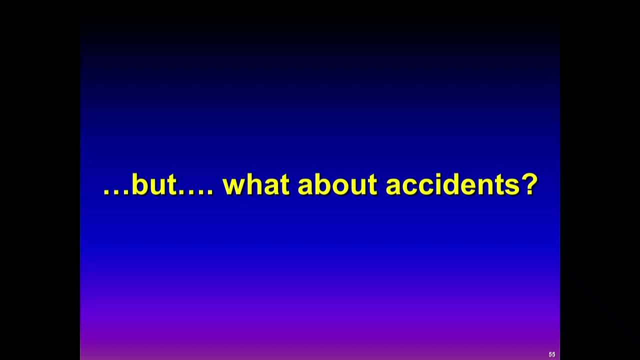 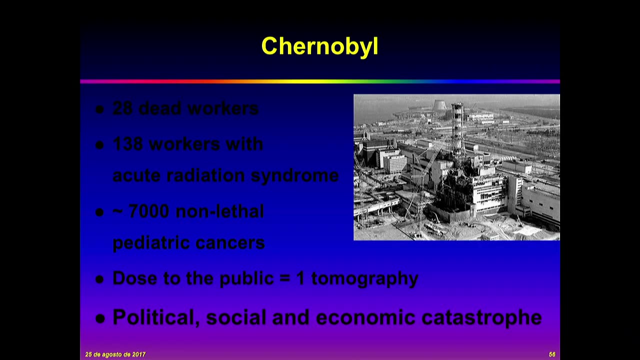 you have accident. Well, this afternoon we are going to talk about that. Even if you put accident into the picture, the thing doesn't change. There were two accidents, you know? Yes, please, How do you distinguish between the origin of the radioactivity? 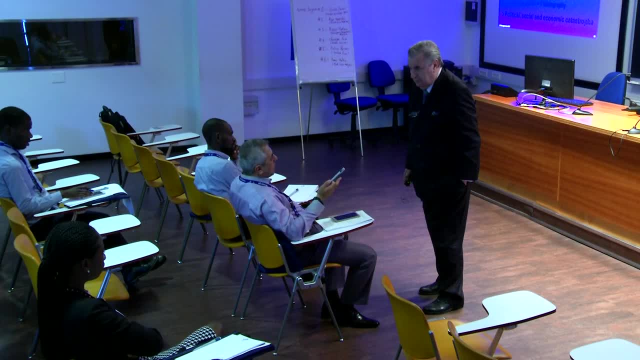 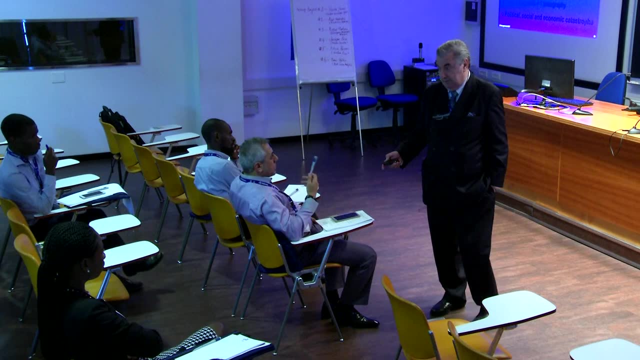 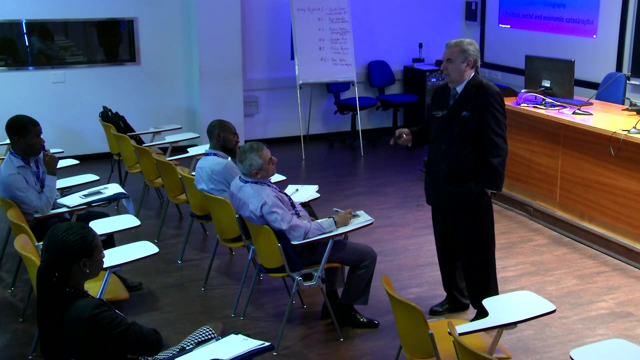 and the origin of the radioactivity. Does it come from this thing or this, or from activity? Well, it's impossible to distinguish, And that is a problem of which we can talk about. For instance, in my country we have a very serious problem. 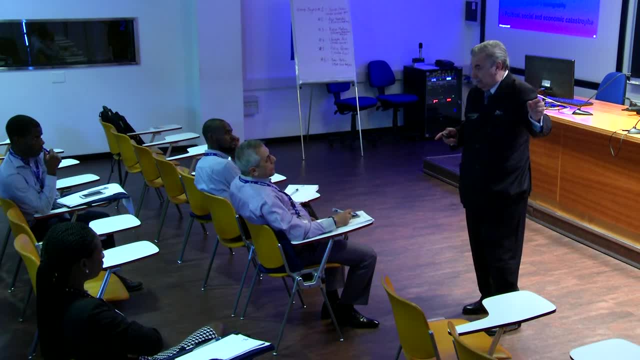 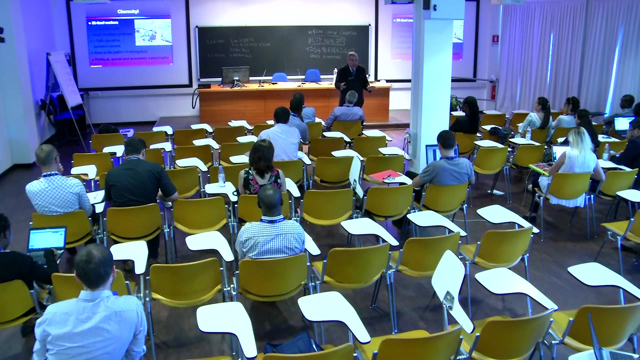 trying to distinguish uranium coming from a factory and uranium coming from nature. You can't do it. There are very complicated chemical processes in the equilibrium with radium etc. But just to make it simple, in my country a problem like this: 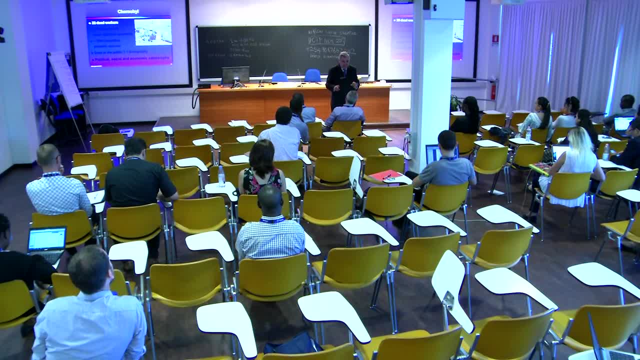 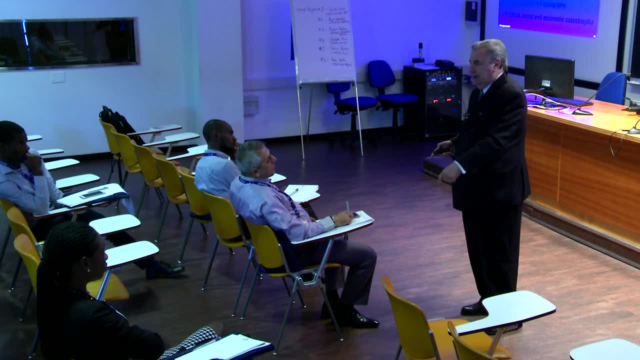 trying to distinguish. it costs one million dollars For- and many times people use this. you know, I don't know. this uranium is not coming, was not put by God there, it was put by the, by the fuel fabrication plant. 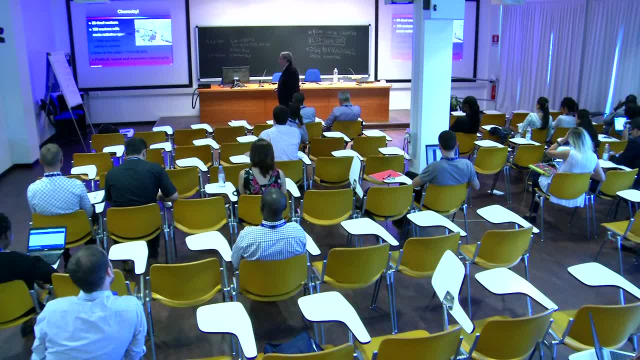 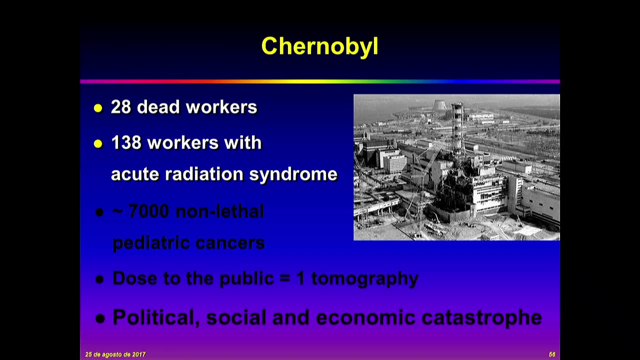 Well, in Chernobyl there were 28 deaths workers- one we will talk in the afternoon on this- 138 with radiation acute syndrome. There were 7,000 non-lethal pediatric cancer because people would not protect themselves against iodine. 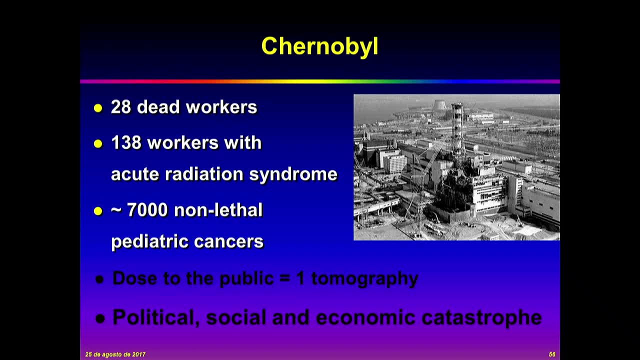 and it's so simple to protect iodine. The mothers didn't know that it was an accident, but they were given milk with contaminated iodine to the children. There were 7,000 cases of thyroid cancer in children. Fortunately, thyroid cancer is not lethal. 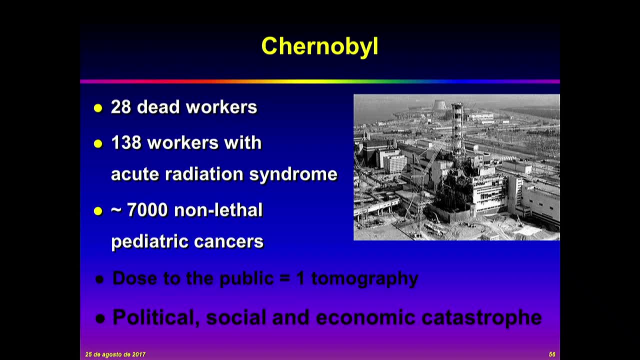 but you know I don't want my children to have thyroid cancer. not that I'm diminishing the problem. The dose to the public was very low During all the period was less than they would receive if they have a tomography. 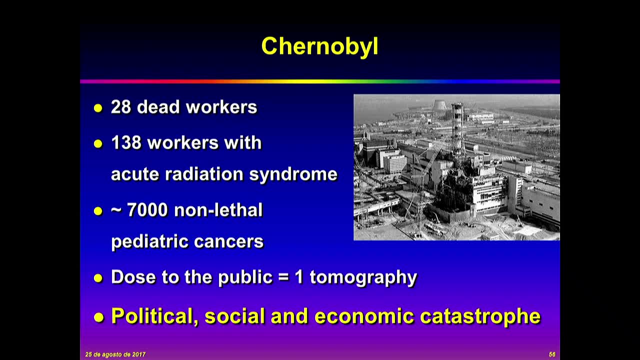 was very low, But it caused a political, social and economic catastrophe- Not radiation, but really social and economic catastrophe. Nobody believed in this data. but this- it was a more study accident- We- I was the head of the group. 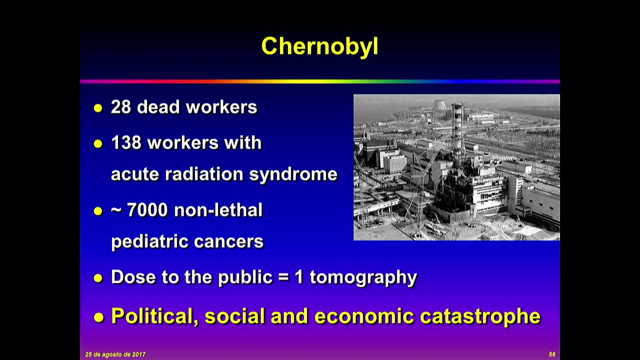 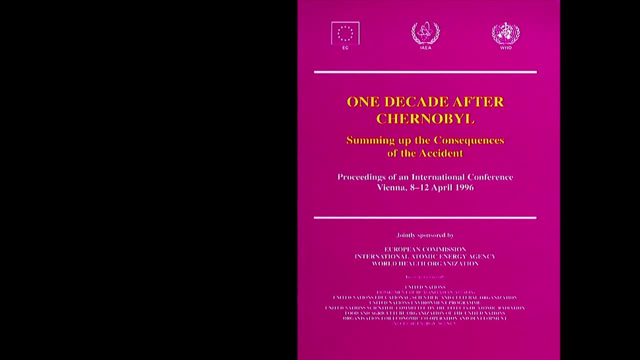 who did that, and we conveyed all that to a very big conference that was chaired. You can have this in the web, in the agency. Here you have all the information about Chernobyl. The conference was chaired by Angela Merkel. People forget that. 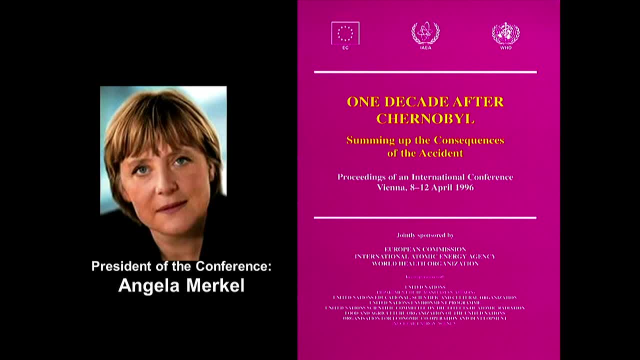 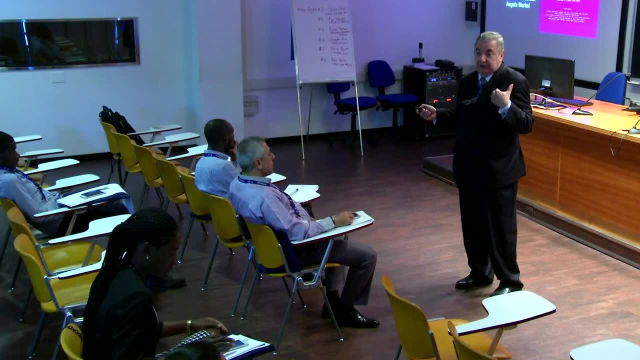 Angela Merkel at that time was Minister of Environment for the Government of the Court. My recall of her is cannot be better. She's the only politician that I met who knows what she's talking about. She's really very good. She's a doctor. 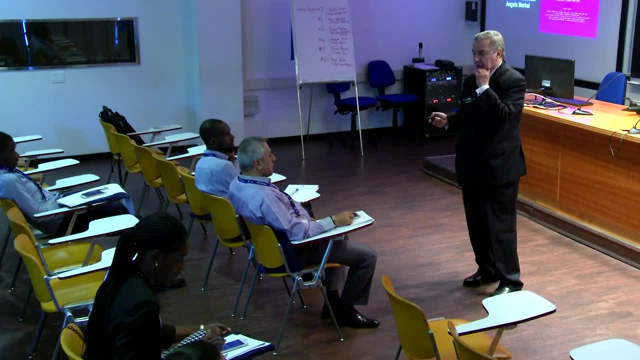 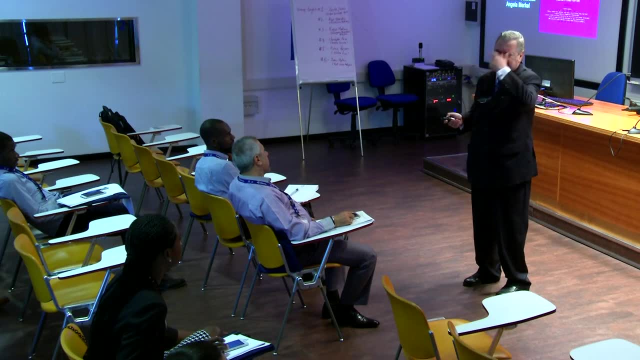 in in quantum, quantum chemistry, Extremely cultivated person. She speaks Russian, French, German, of course, English, whatever language that you want. Therefore, my recall of her at that time was super. Then politics changed people, you know. 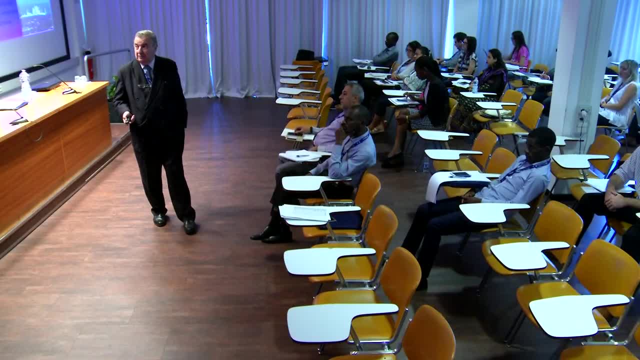 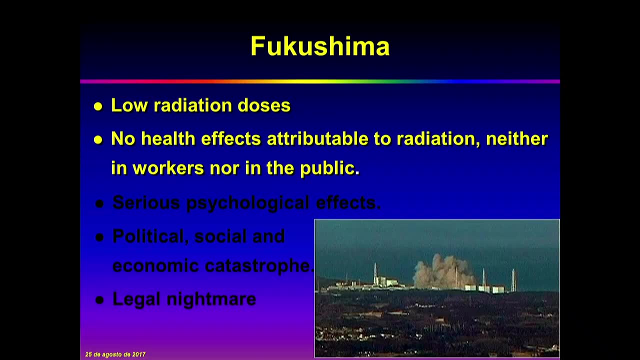 but Fukushima: low radiation doses, extremely low. We will see this in the future. We will see this in the future as well. No health effect, of course, but serious psychological effect Again. political, social and economic catastrophe. 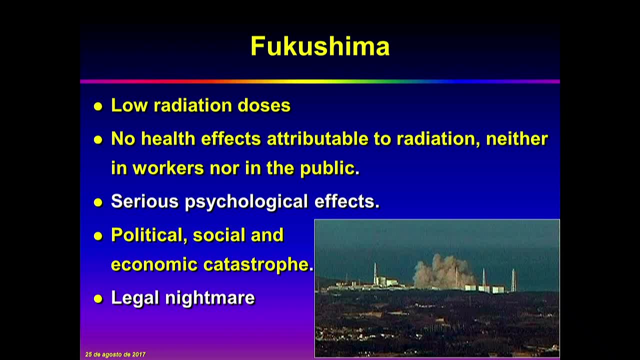 an illegal nightmare for the Japanese government. No radiation, not effect, but big drama Again. this was very deeply studied. I was the head of the group of the agency that studied the consequences and we produced a very big report that you can find. 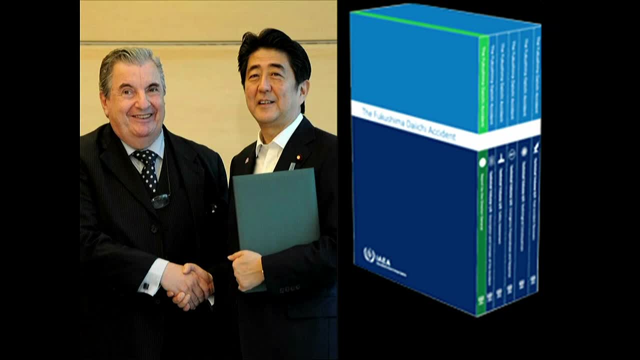 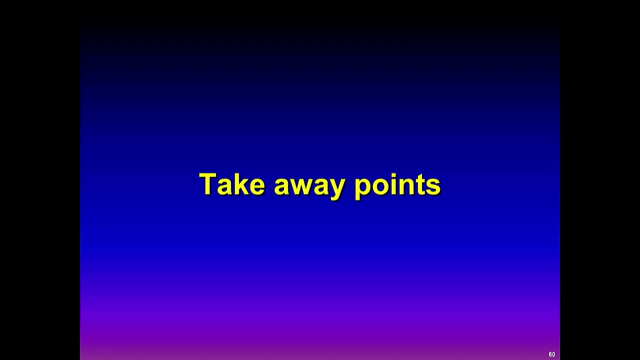 in the web. I am here with Prime Minister Abe and the report has six volumes and you can get in the web. One volume is dedicated to the concept. My takeaway point from this first part: remember activity becquerel. 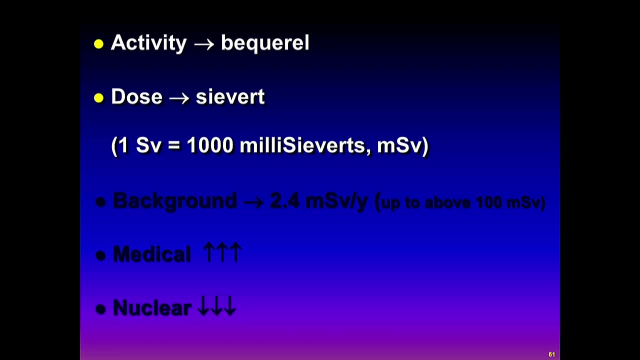 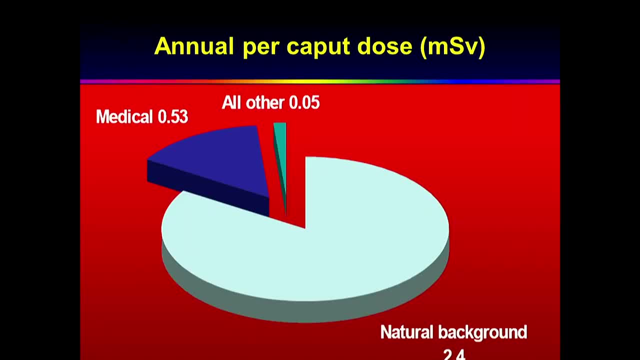 Thank you. Any other questions or any other information that you'd like to add? Thank you so much, President McG savory. Many, many privileges have been presented by MMDCC. In fact, they've been monded over 7.5 years. 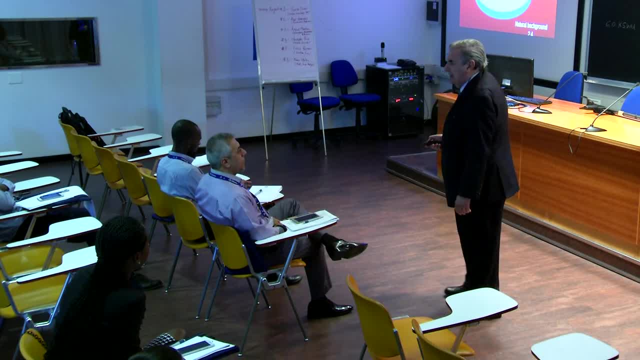 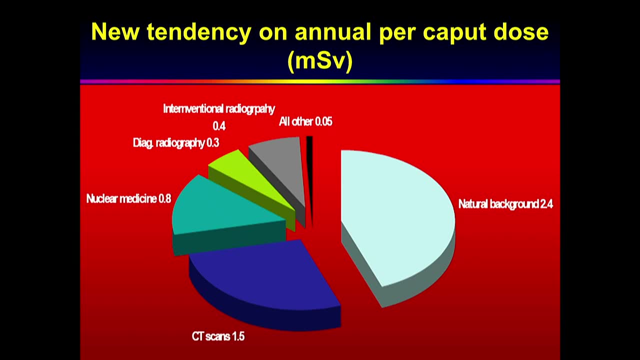 Basically making trials for medical and medical treatment projects has going for site practice. Everybody wants to have a CT, everybody wants to have a photo of inside. Also, the introduction of digital radiography. this is very interesting. We introduced, we invented, digital radiography to reduce doses. 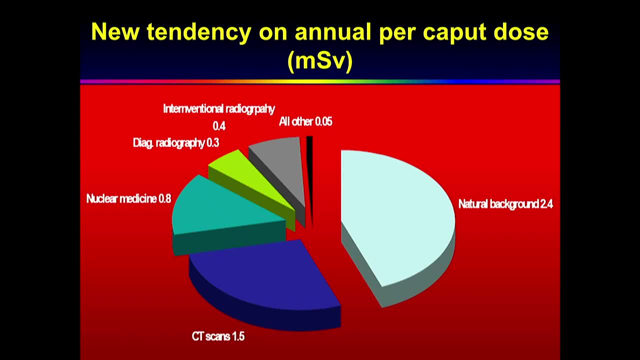 But what has happened? Like with the photos. You remember when you have to have a photo with the old system, with the film. Before having a photo you thought twice because you will ruin the film. Now what happened with the digital photography? 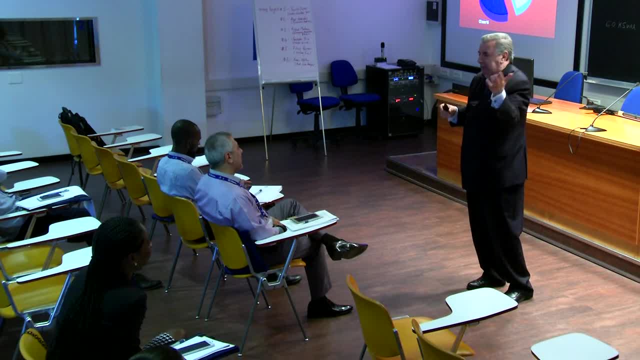 You take one photo, take another, one another, one, another one, then you select one, You delete the others. Well, the doctors are doing exactly the same with you with digital radiography: They take several and they select one. As a result, the dose of the people have increased, not decreased. 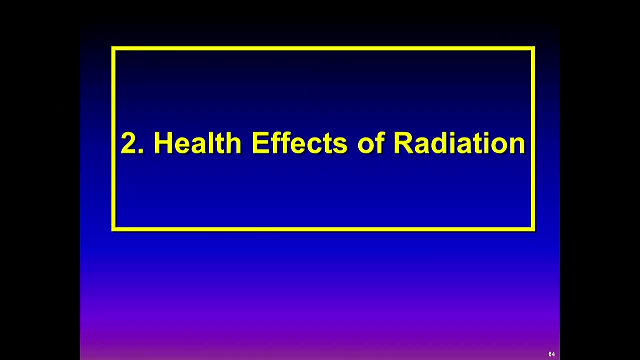 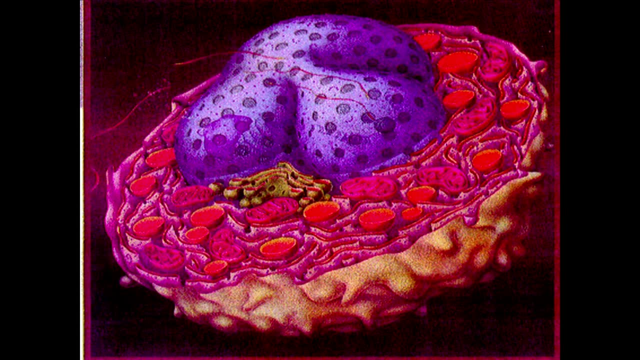 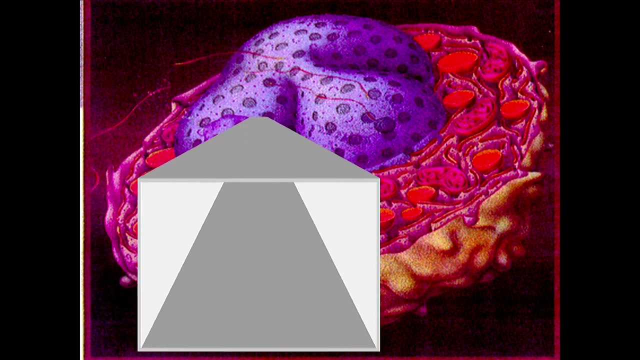 Well, let's move to health effects, The biological basis. We have to start with a more sophisticated invention in the history of humanity: The cell. The cell is really a fantastic machine. This is a picture of the cell. You know that inside the cell, in the nucleus, you have the chromosomes. 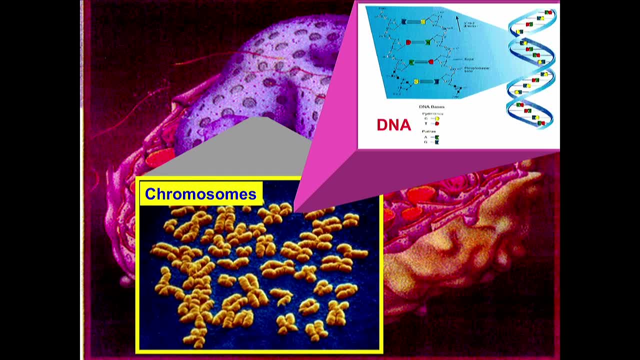 And you know that the chromosomes are the organization of a molecule, a very long molecule called the DNA, which contains a computer code. That computer code contains all the instructions that make you a person and operate like a person. It's a code like in a computer. 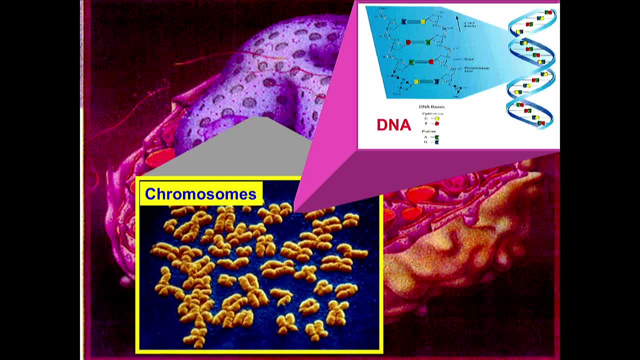 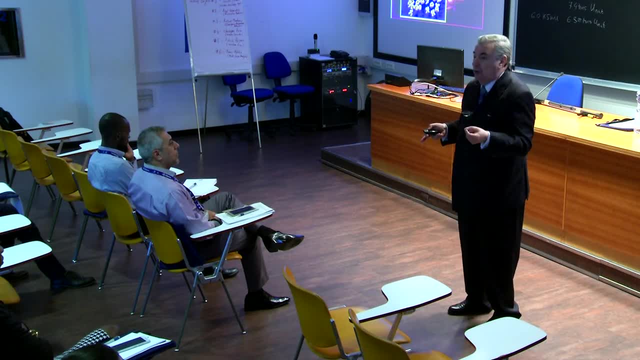 In the computer you have two terms: zeros and one. In the DNA there are four. That is the only difference. But it's a code. There are sub-programs, like in a computer, And one sub-program is called a gene. 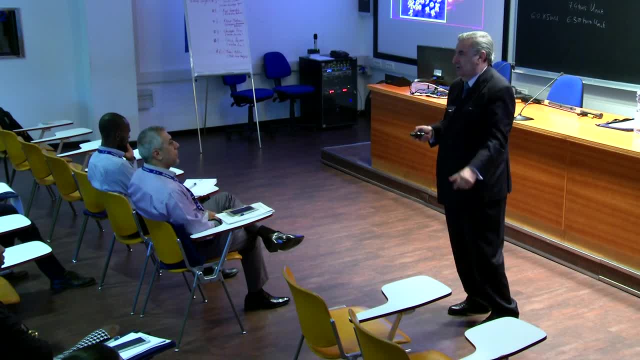 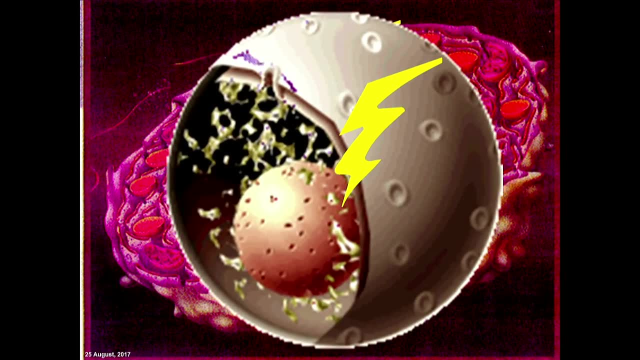 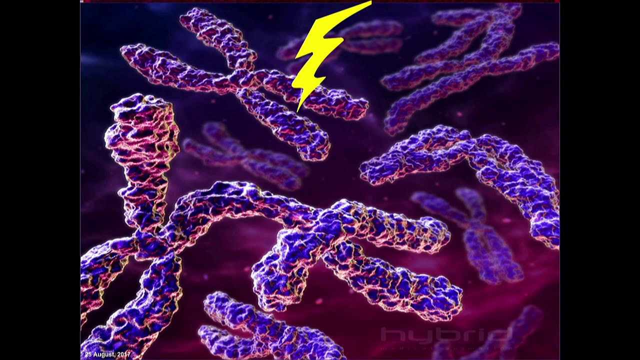 A gene is a sub-program in that code. Well, when radiation interacts with your body and interacts with the cell and with the nucleus of the cell, it obviously interacts with its chromosomes And by interacting with the chromosomes it interacts with the DNA. 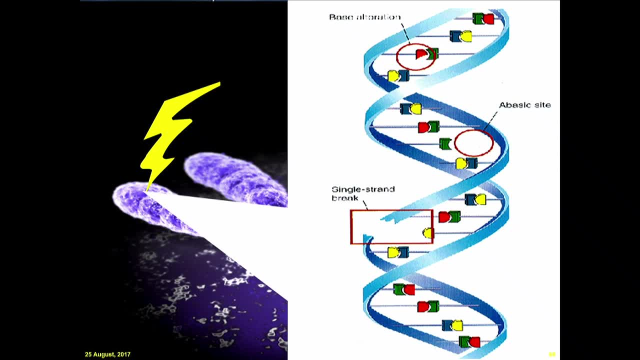 and can, by ionizing the molecules in the DNA, can make changes in the DNA. For instance, the DNA has, as you know it's, a double code. It's double just to get like in a computer. In a computer, many times things are doubled. 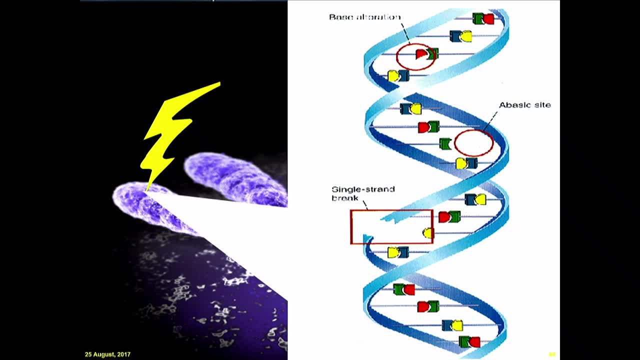 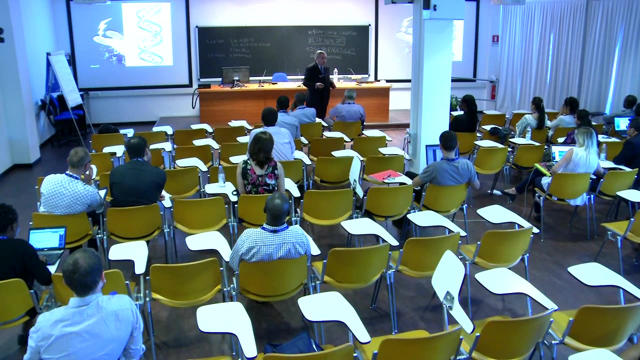 to get one as a model to repair. if something goes wrong In the body, it's the same And the DNA can be broken. Some of the molecules can be broken. These changes are called. I ask just to complicate your life. 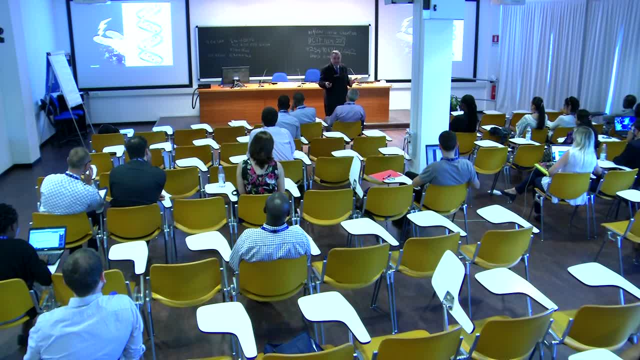 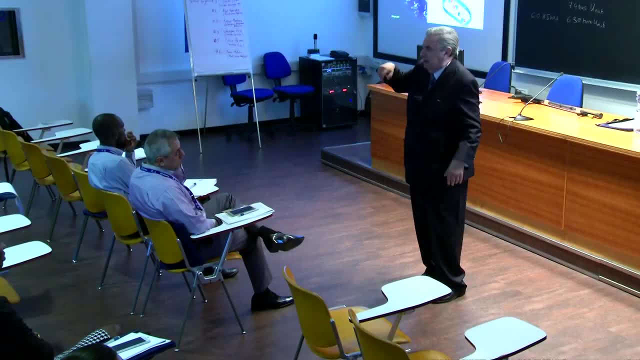 mutation. Well, people don't understand this. You say to the people there was a mutation. People understand: oh my goodness, this is a Martian. We have a person with three legs. No, a mutation is a change in the code. 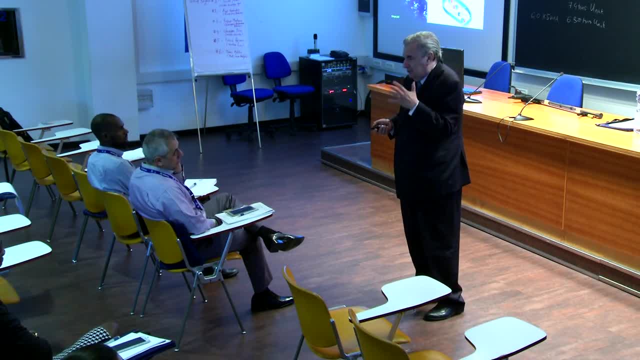 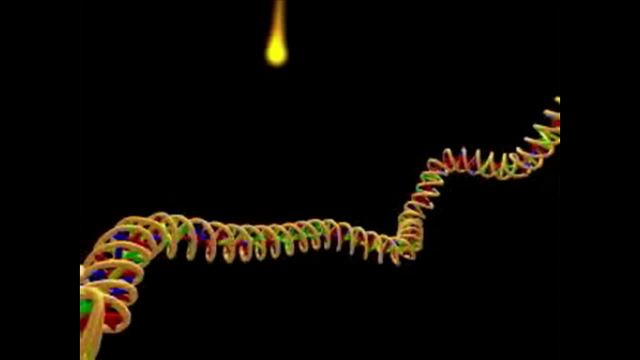 In the computer you would say a change in the code, But we say mutation just to confuse people. Mutation Doesn't work. It doesn't work, It's a bit. Well, I will show it to you how mutations work. 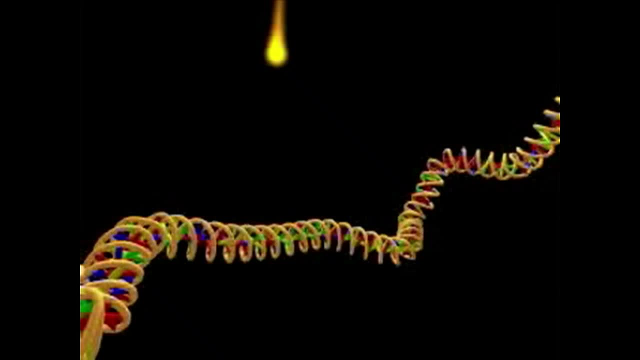 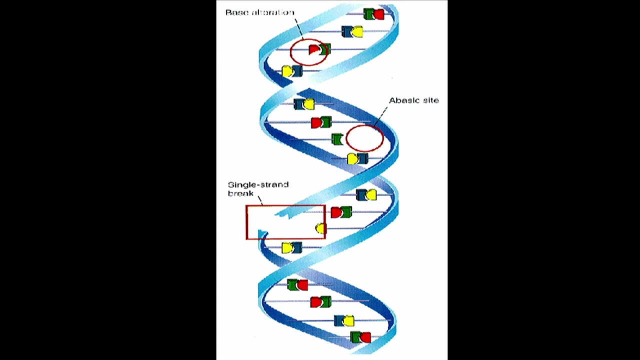 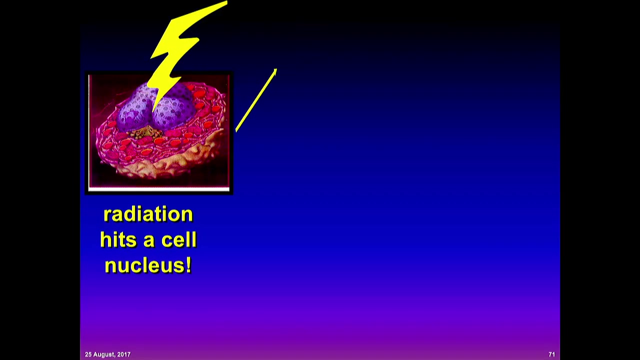 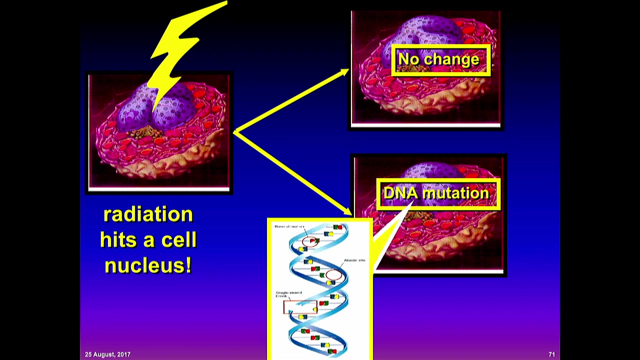 what radiation is coming interact and produce these changes in the DNA. It's a pity that it doesn't work. I will check, then why not? Well, mutation usually is simple, but the mutation can be complicated. And therefore what? the two alternatives? 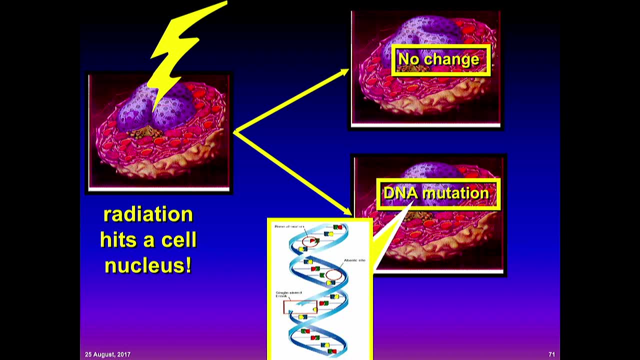 have is when radiation hits a cell nucleus. really, two things may happen: That there is no change, no change at all, because the ionization was produced, or that there is a DNA mutation. The probability is low but it may have a DNA mutation. 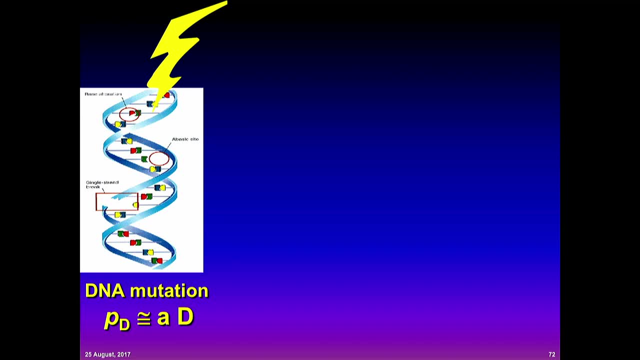 Now, if a DNA mutation occurs- and this will be more or less proportional to the dose, because higher dose, more energy, more radiation, more radiation, more radiation- If this happens, you have the following alternative: When is the mutation being repaired? 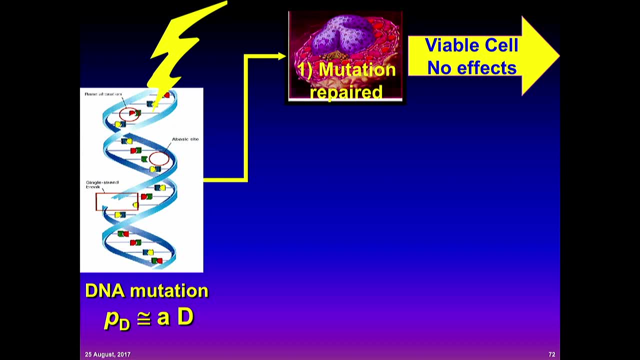 And this is very common- because the cell has a mechanism like the computer has, a mechanism to repair damage which is extraordinarily efficient, Or that the mechanism doesn't work or the mutation is so big that it cannot be repaired. If this happens, 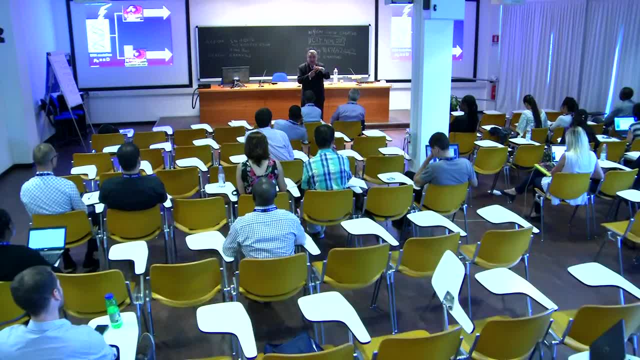 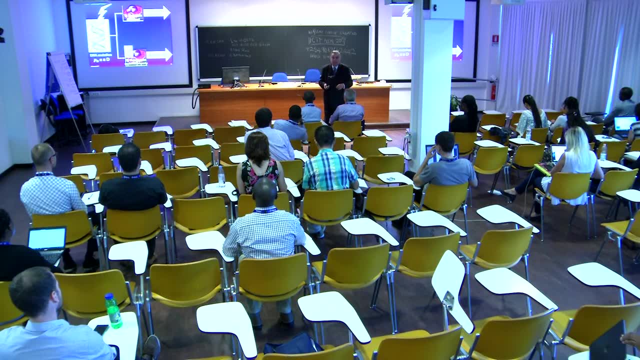 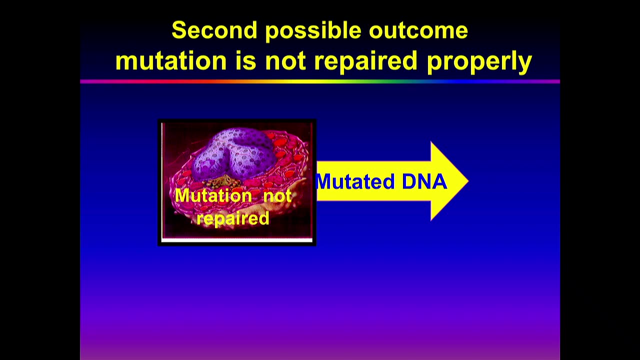 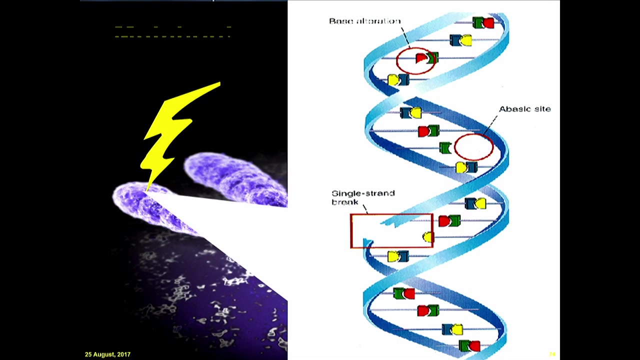 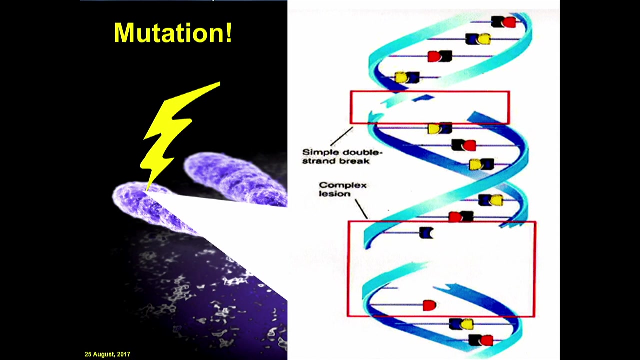 you have a mutated cell, a cell that is not the same as the others. It's a computer with different information. Now, what happens if the mutation is not repaired? You have a mutated NEA. Well, if this happens with this mutation, 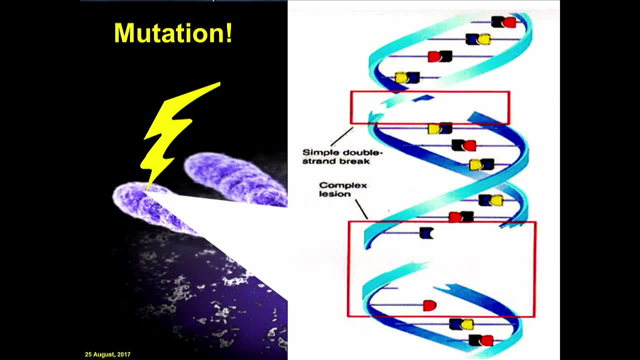 which is very big, you know, the two parts of the NEA have been damaged. For even if the cell can have a system for repair, how can we repair it? The cell tried to repair it, but repaired it wrongly and produced what we call. 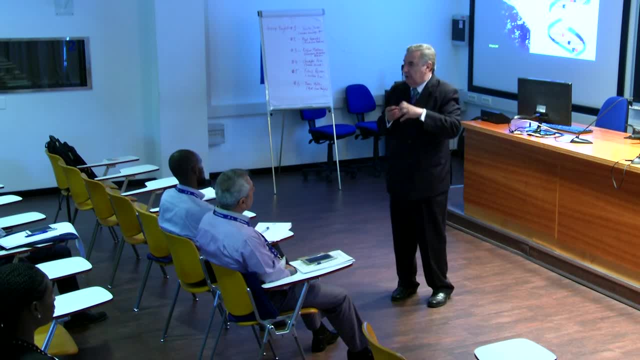 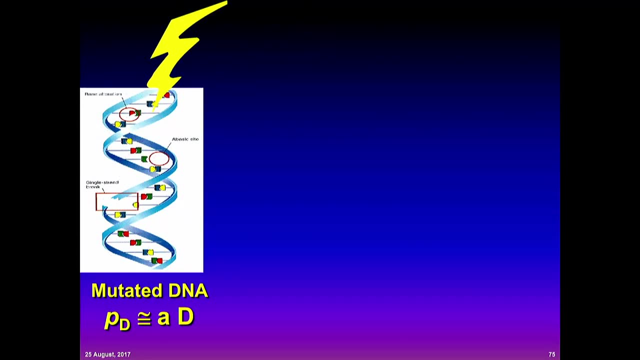 chromosomal aberration that we can see in the microscope. The chromosome became different. If this happens, and the two things that may happen, the first thing is that the cell dies due to this change. It's like any computer: You make a change in the program. 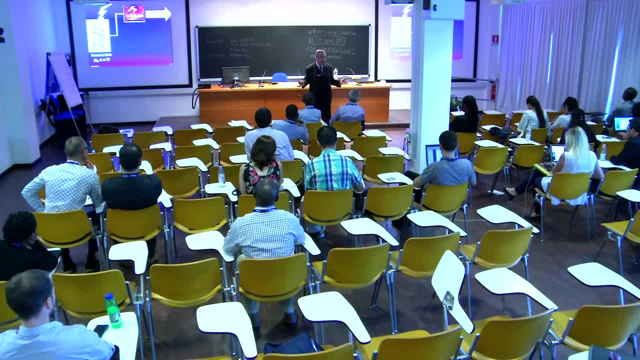 and the computer dies. It doesn't work anymore. Well, if this happens with your cell, it's not a bad thing, but new, Because in your body every day there are cells dying And other cells will come. but that is not a bad thing. 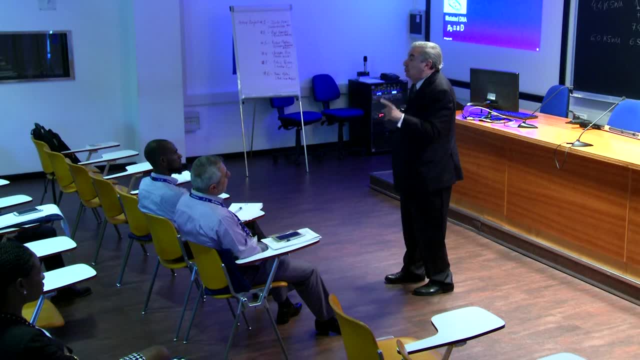 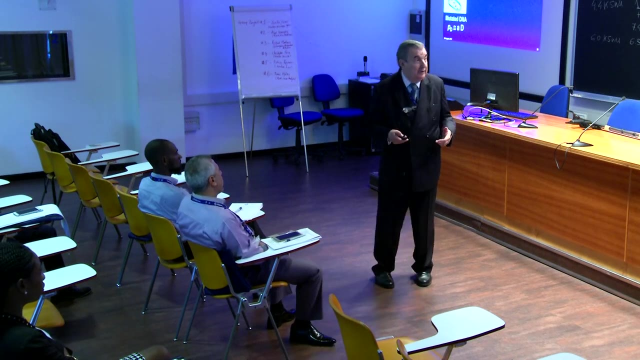 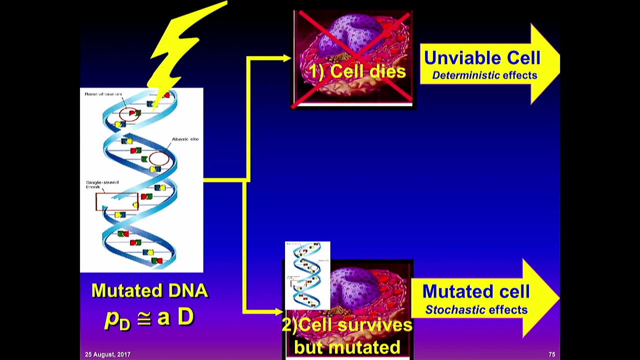 Now, if the radiation is so high that many cells die in one organ, the organ collapses, And if the organ is important, you will die. The second outcome is that the cell survives. It's not dead, It survives, but it's a different cell. 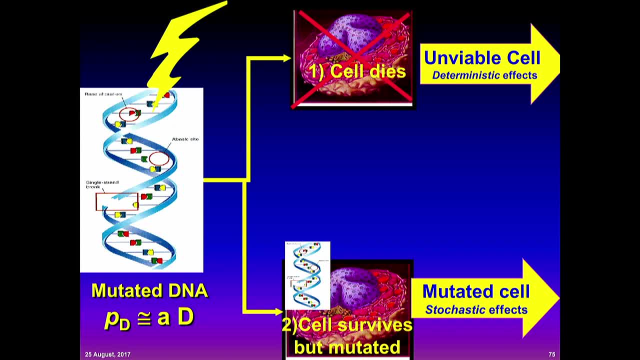 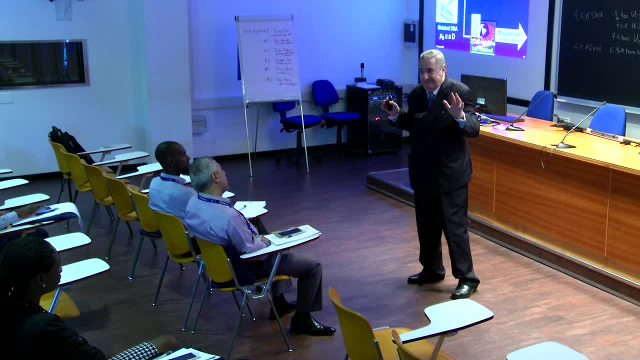 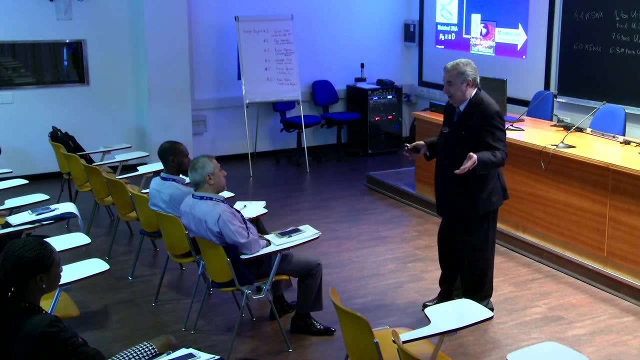 a mutated cell. For it's like if in your computer there was a change in the program and the computer continued to work, But you don't know that there was a change in the program. And well, maybe the computer will work better with this change. 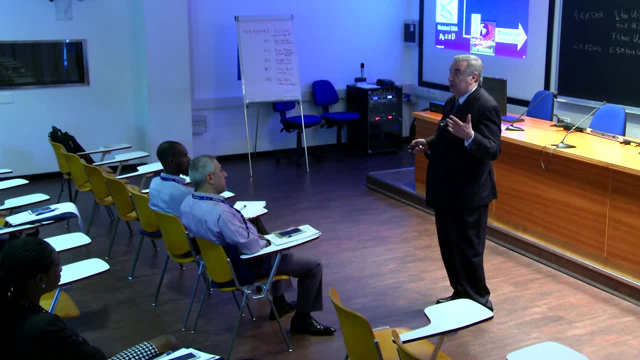 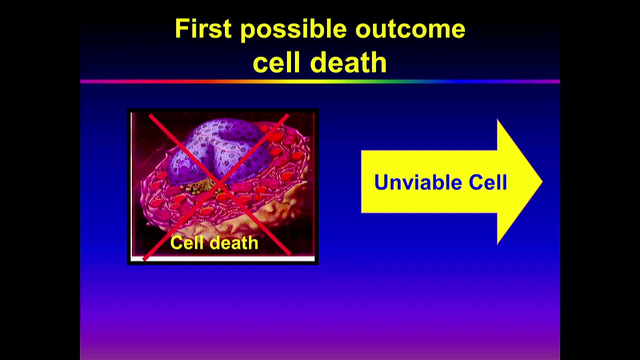 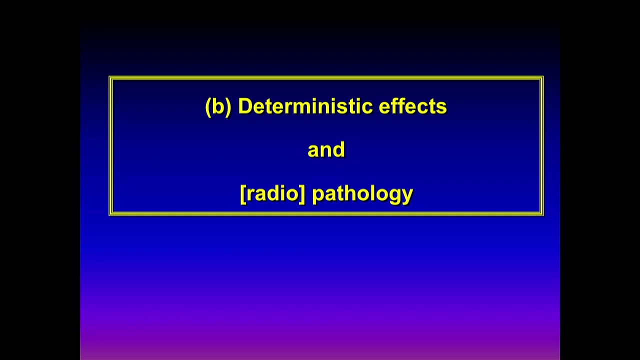 or the computer can work worse and you will not even realize it. Let's move to the cell death problem. As I said, there is an unviable cell that will be replaced, but if many occur, deterministic effects occur and these are covered. 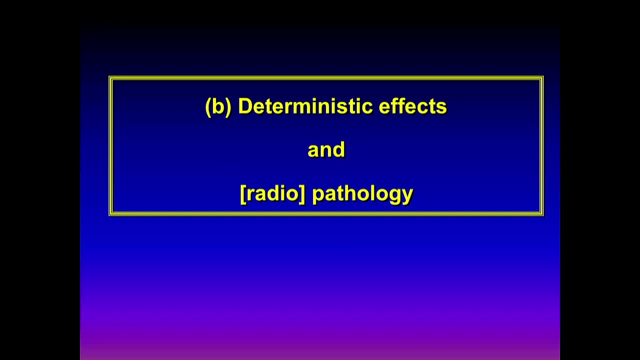 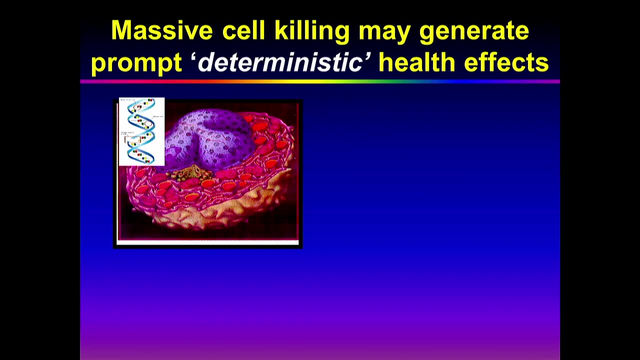 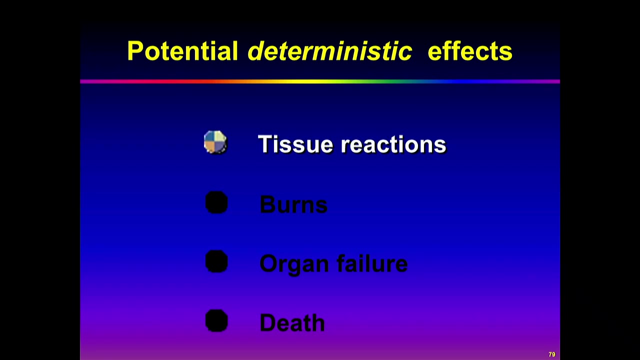 by the science of radiopathology We call deterministic effects because they are determined to occur if many cells have died. Deterministic effects can be tissue reactions, burns, organ failure or death. The occurrence of deterministic effects in the exposed individual. 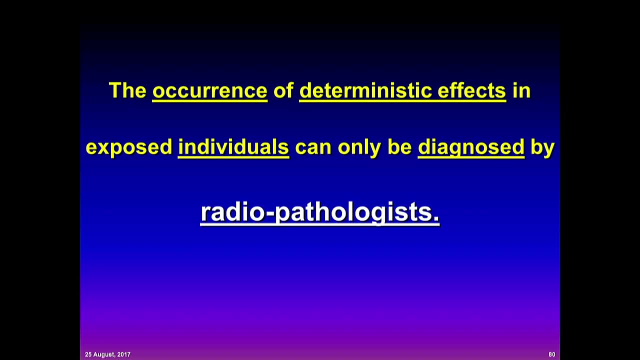 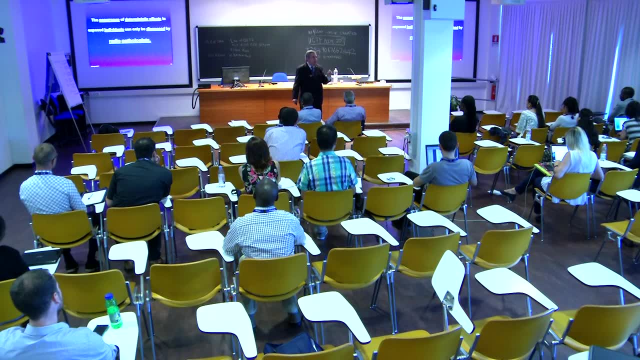 you can do it in any individual. you can diagnose one individual. you can do it in any other individual, you can do it in any other individual. you can do it in any other individual and you can do it in any other individual. 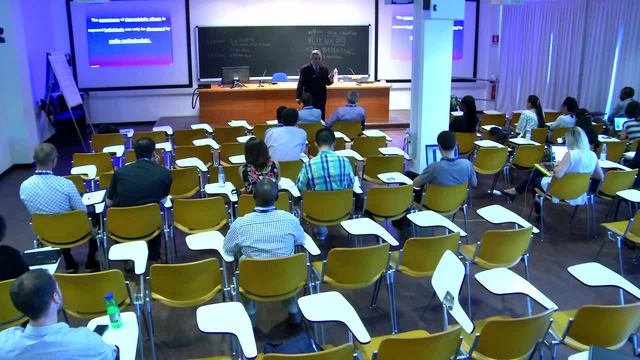 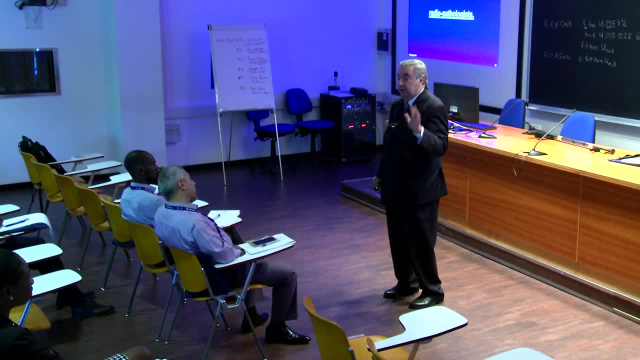 It's done by radiopathologists. For the first thing that I want to put in your mind, if, for your work in the future, it's important that you know or have at hand a good radiopathologist, and I tell you the following: 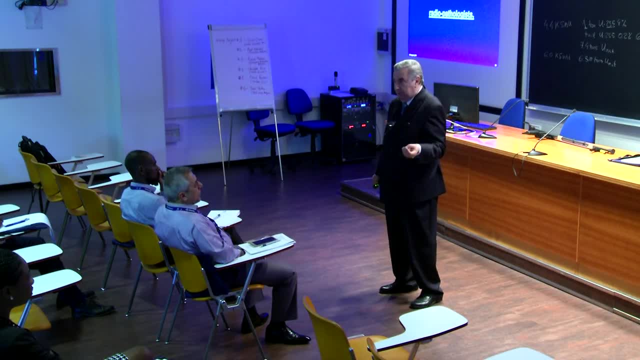 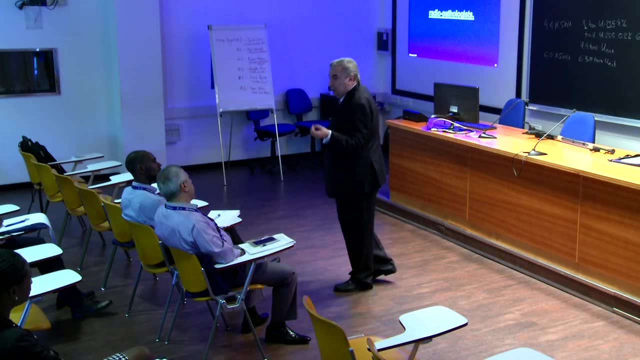 There are very few, very few in the world. For your country you can do at least good radiopathology In Argentina. we have a good experience on that in the Institute of Burned People and I recommend you to look at the same in your country. 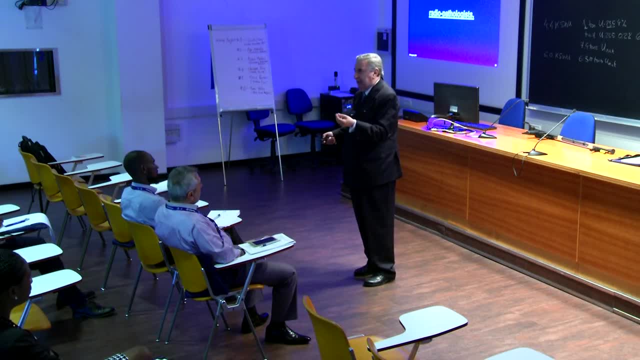 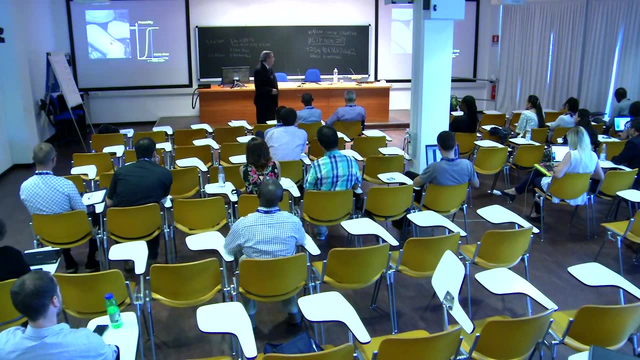 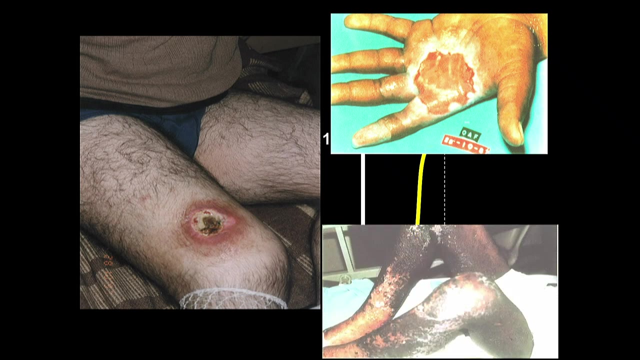 The Institute in the hospital will treat burned people. You can have there a good element for building a good radiopathology, But there are very few in the world. I tell you that When cells are dead, simple effects like this one more complicated. 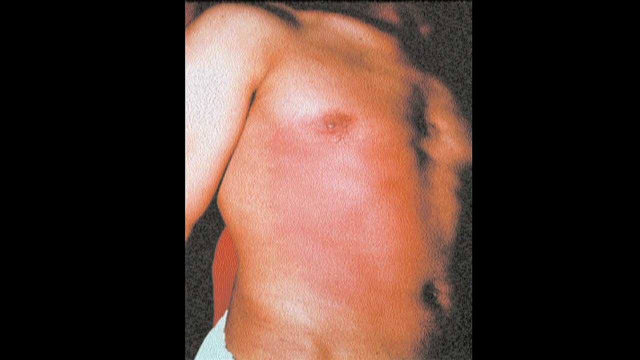 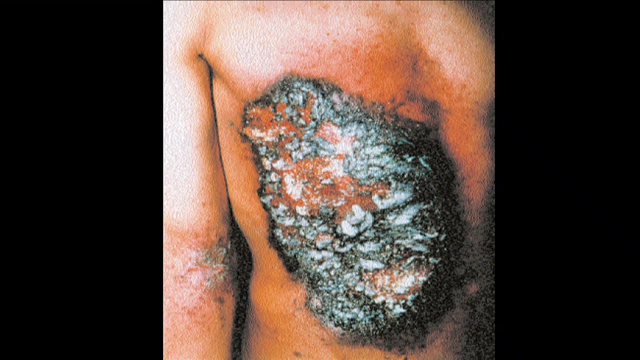 more complicated or really think that the fellow has radiation here at the beginning The doctor says no, this is nothing for radiation in radiopathology. A few days after it was red and a few days after you have this. 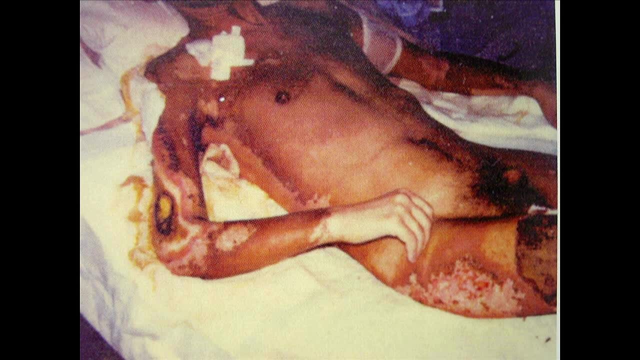 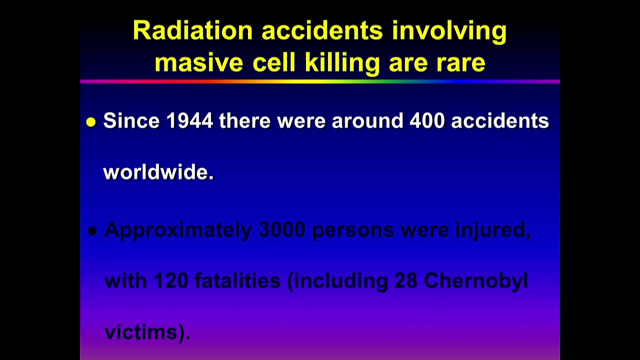 An effect like this. you know, a person completely burned for radiation can be very complicated in high dose. But very few people, really very few accidents involve high doses. See in 1994, there were 400 accidents, 3,000 persons were injured. 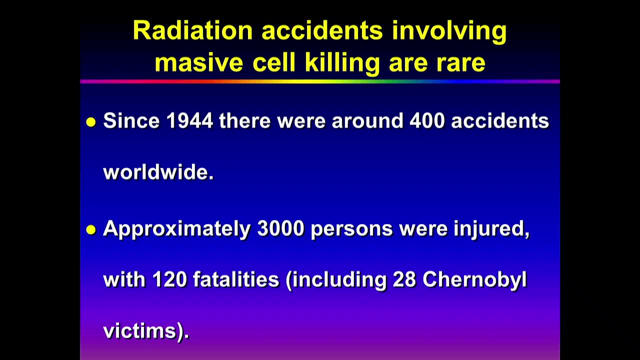 100 fatalities, including the 28-year-old Chernobyl. I mean imagine all the history of radiation. 120 fatalities is not a big big number, But radiation can be very dangerous in this case. The second outcome, as I said, 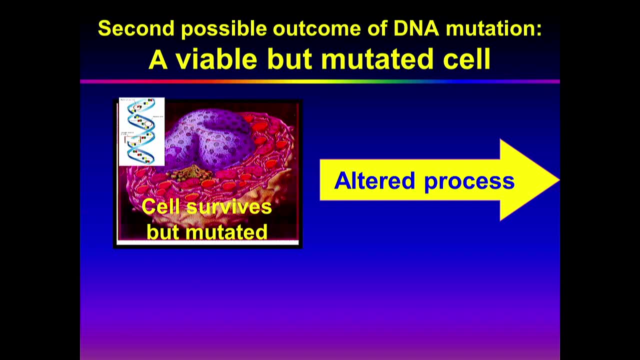 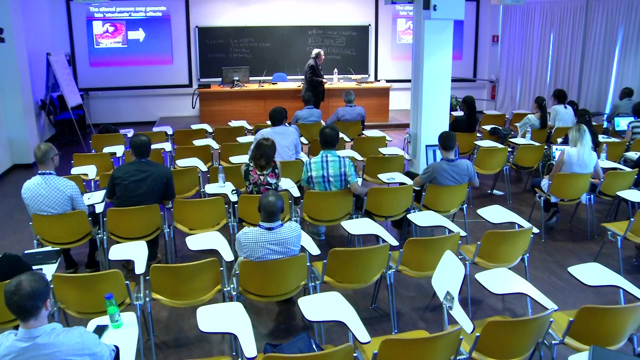 the cells survive by mutating. For the cell which produces all the information that you make what you are as chemical products, this process is altered for it's producing different things. that cell Maybe positive for you, maybe negative, These negative things, 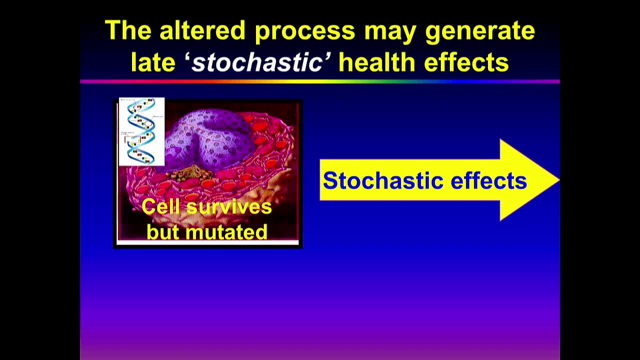 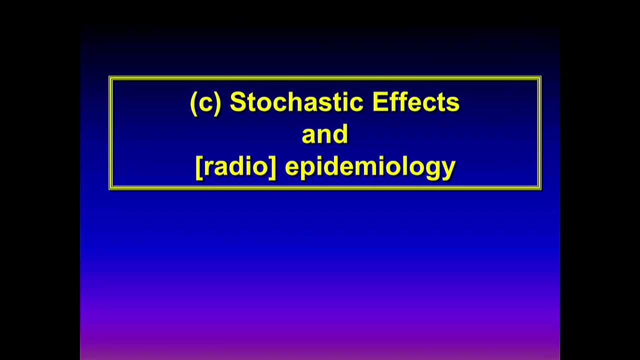 we call a stochastic effect, Again, a sentence that does not help to be understood. stochastic in Greek means at random. This effect occurs at random. It may happen or may not happen, And they are studied by the science of radioepidemiology. 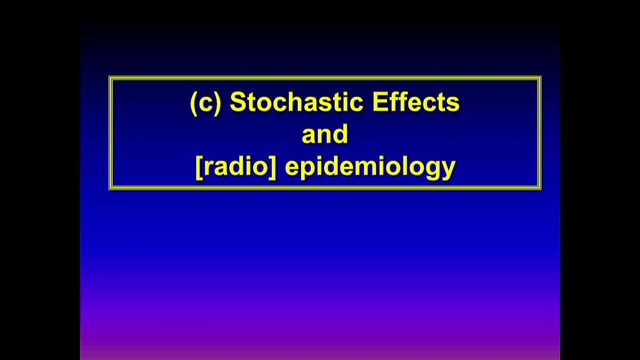 An epidemiologist is not a pathologist. An epidemiologist is a statistical person. He looks at a population. Here you have a population that was not exposed. Here you have a population that was exposed And he sees that there are more effects in this population. 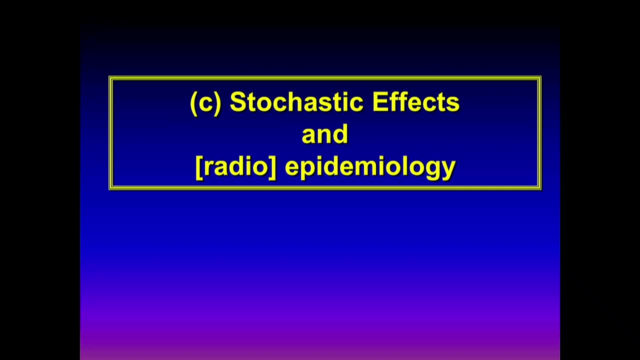 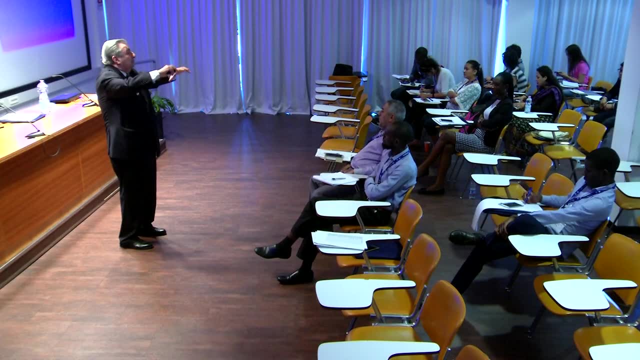 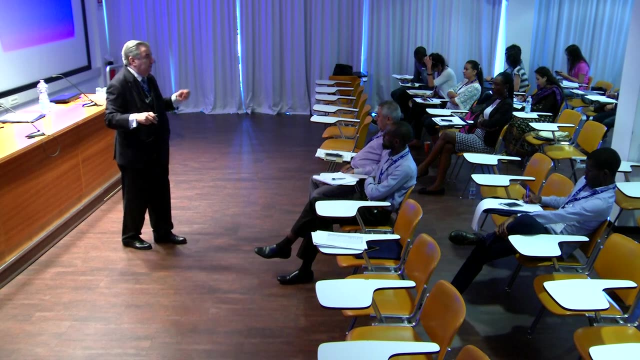 statistically. An epidemiologist- it's important that you understand- cannot diagnose an effect in one individual. He cannot. He diagnoses effects in one population. But this is important for you. There are very few epidemiologists in the world: radioepidemiologists. 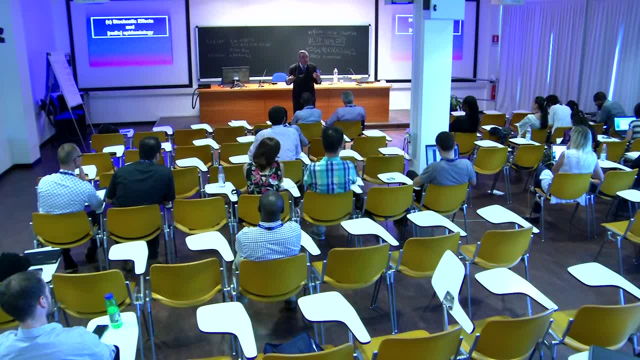 And in that in my country we have failed. We could not build good radioepidemiologists In Argentina. there are no radioepidemiologists. We need to rely on outside people. For another lesson for you in your country: 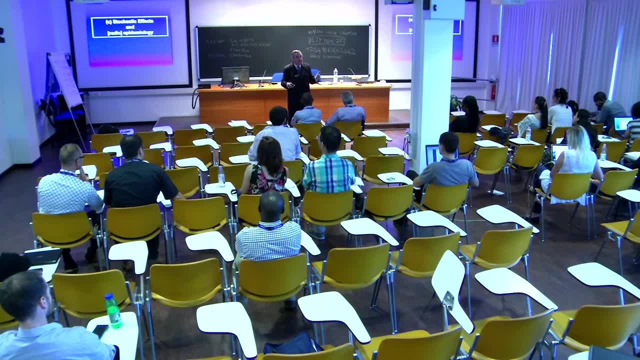 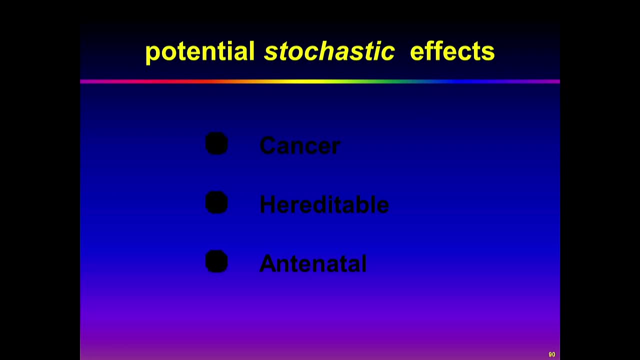 remember, try to get a good center of radiopathology, a good center of radioepidemiology. What are the potential stochastic effects, these negative effects produced by the change in the cell: Cancer, hereditary effects and antenatal effects. 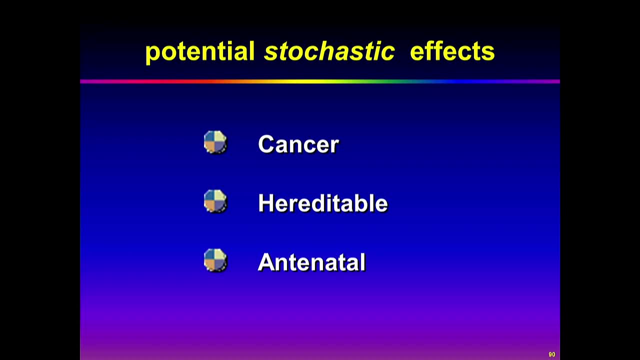 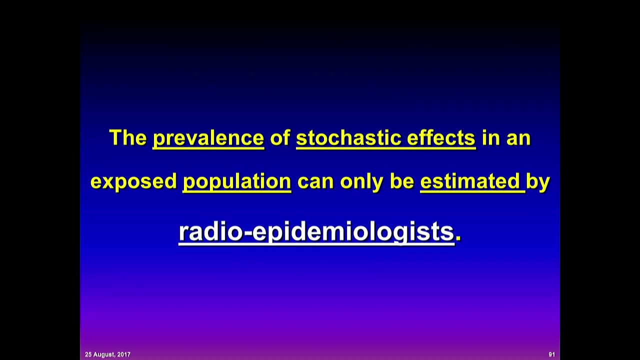 effects that have occurred because the person was irradiated while in utero. These are three things that we have studied very deeply. The prevalence of these effects in an exposed population, remember, can be estimated by radioepidemiologists. It's in a population. 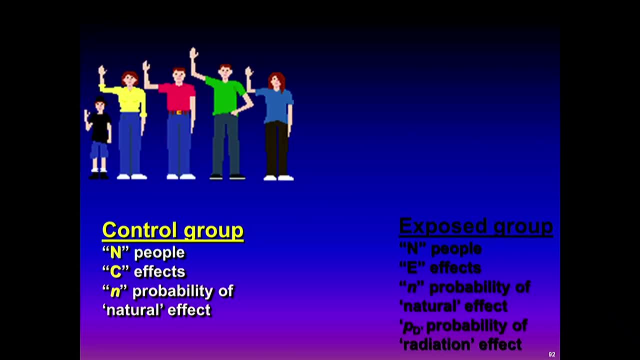 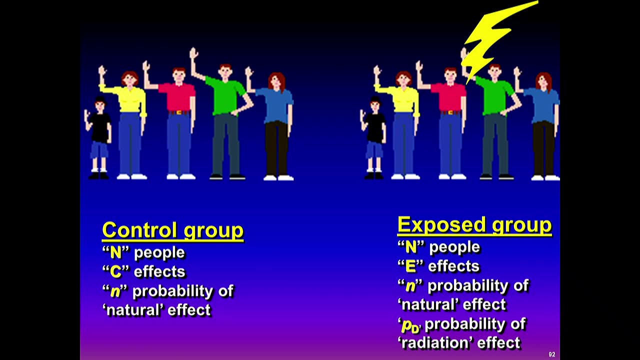 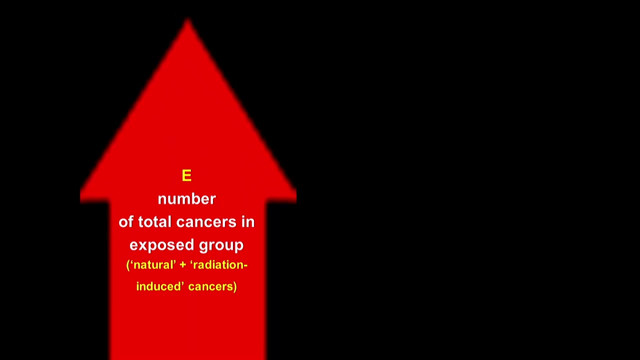 not in one individual. What the epidemiologists do? they have a control group and an exposed group and compare both groups. This is what the epidemiologists do basically, And that is not easy because you have the number of cancers in the exposed group. 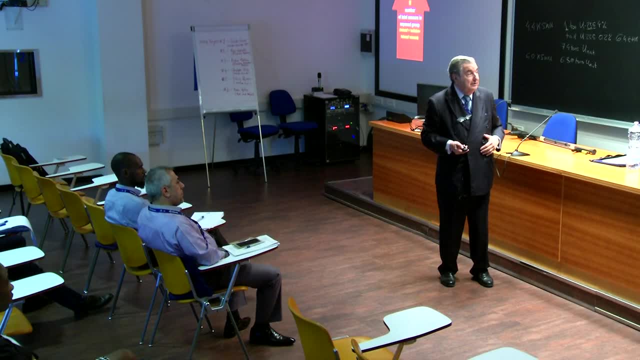 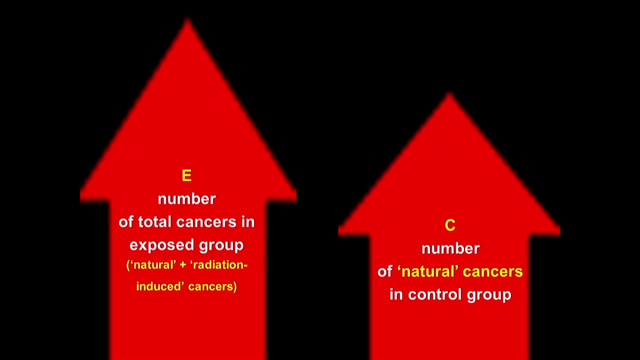 which oscillate statistically, but the non-exposed group also have cancers, cancers that were not produced by radiation. 25% of the people get cancer In this room. 25% of us will get cancer. Have good luck, But it's like that. 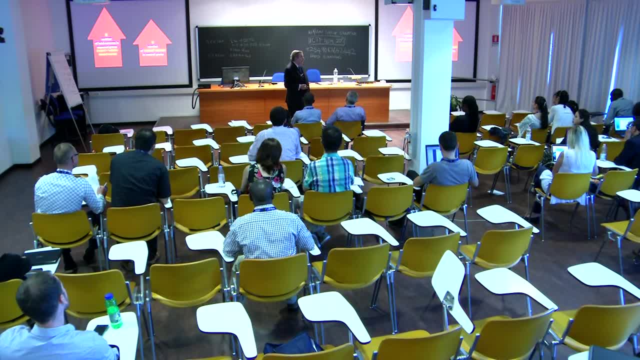 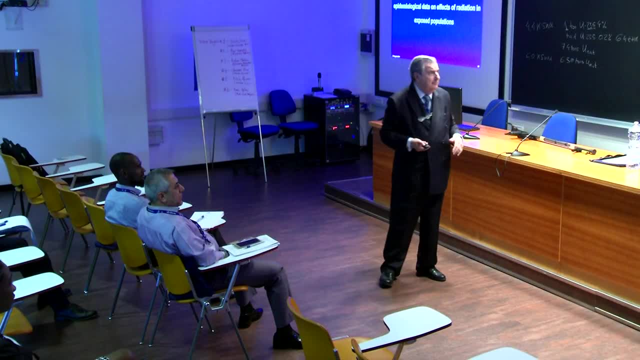 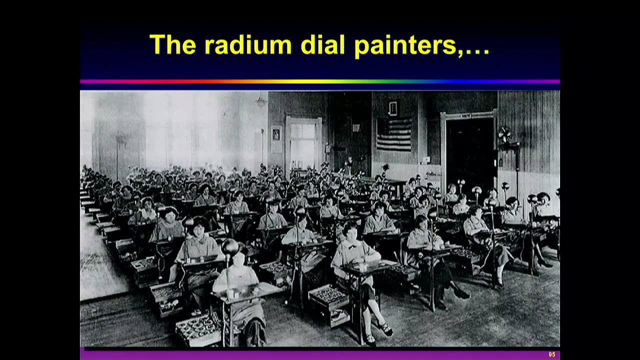 And these numbers also oscillate And the epidemiologists have to see this difference which is oscillating, also Not easy, And SCARE have reviewed many, many, many epidemiological data. The first one I mentioned yesterday, these radium girls. 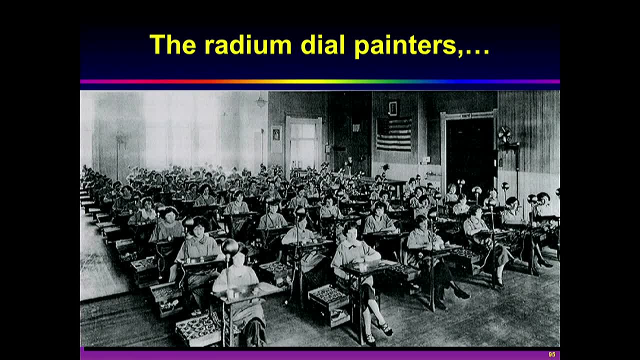 The girls that were painting dyes with radium and putting their pencil in their mouth. This was the first big epidemiological study. These girls died, all of them of cancer of bones, because the radium has the same chemistry with calcium and goes to the bones. 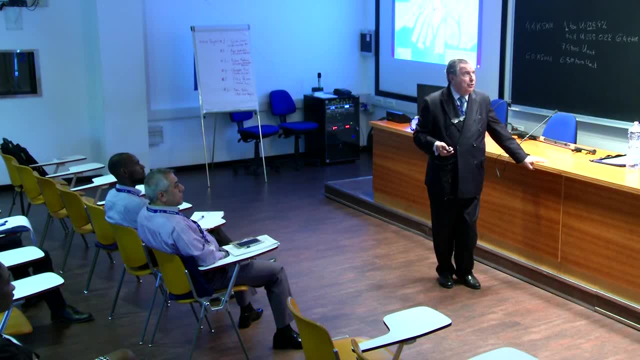 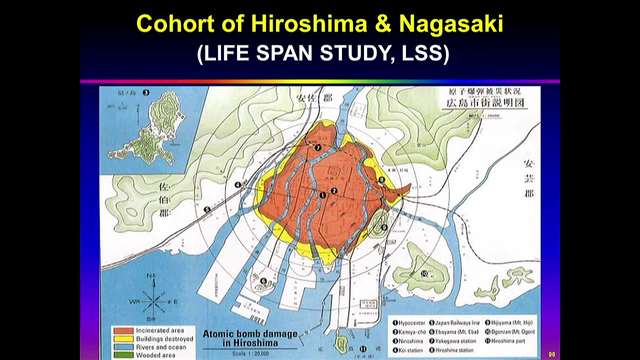 And many others, But obviously the main one was the cohort of Hiroshima and Nagasaki. Well, cohort is a word that we use also to mean a group of people. I mean, we confuse people. Why don't we say group of people? 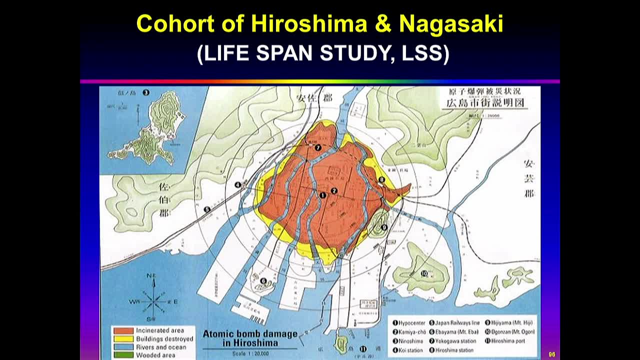 No, cohort. Cohort is a group of soldiers in the Roman army. Well, you have there the map of Hiroshima. The red area was destroyed by the bomb. Well, the area of sufficient dose for deterministic effect was this area. First lesson: 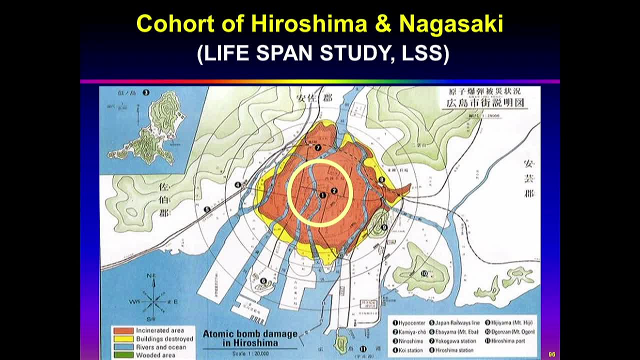 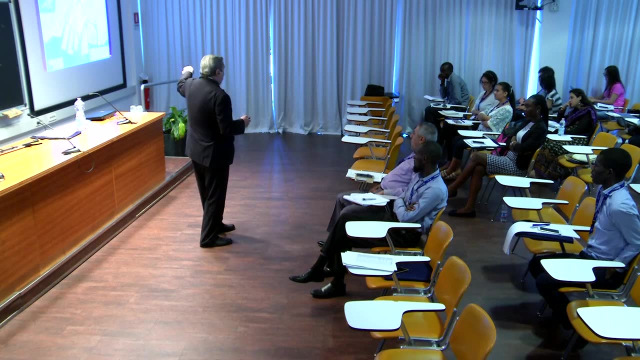 that nobody will believe you. In Hiroshima, people died, many people, 100,000 people died Not because of radiation, Because of the bomb Explosion. The people in that circle would have died if they would not have died, But they were not killed. 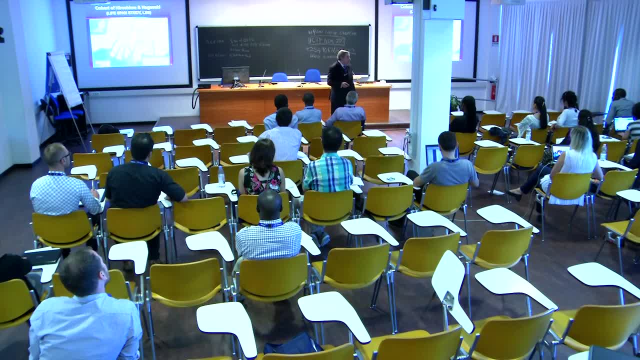 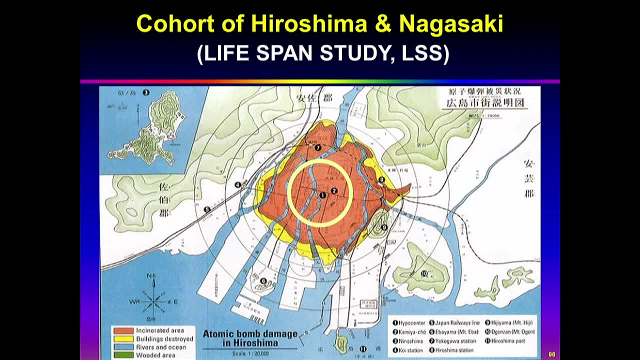 But they were killed by the bomb first. But you know, in Hiroshima, many people, people living here, they were not killed by the bomb, not by direct radiation, not by deterministic effect, but they received radiation For they were prone. 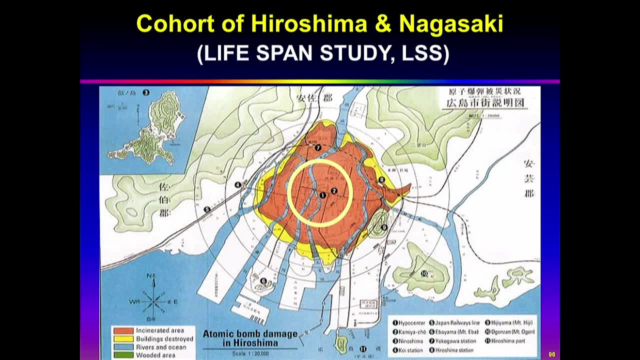 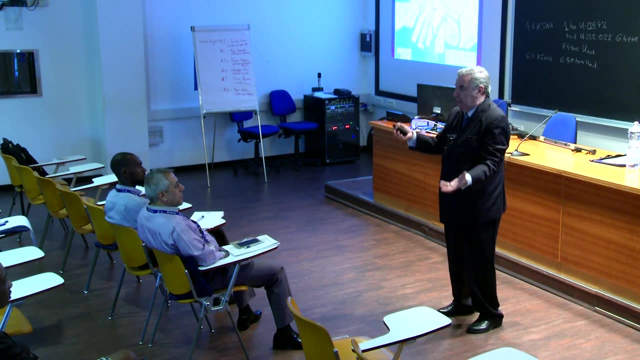 to have stochastic effects. And, interesting, in Hiroshima there are many mountains, as you see around. There were people behind these mountains who were shielded by the mountain, for they did not receive radiation. For we have there an ideal situation for making a good epidemiological study. 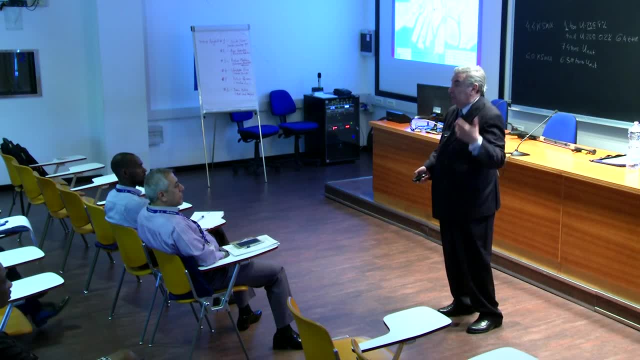 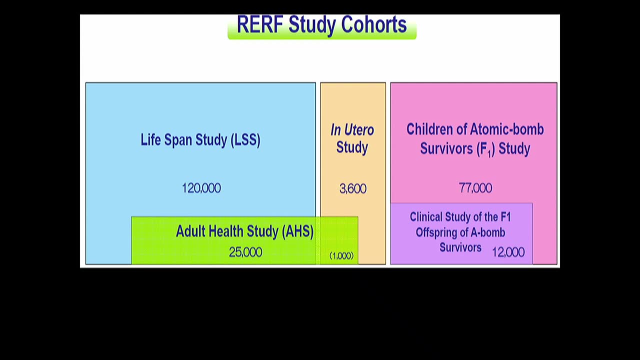 Have people exposed, People not exposed, But the people exposed were exposed to very high doses. Well, this study was done in Japan with the so-called RAF Radiation Effect Research Foundation One. They are just a few weeks ago and there are new information. 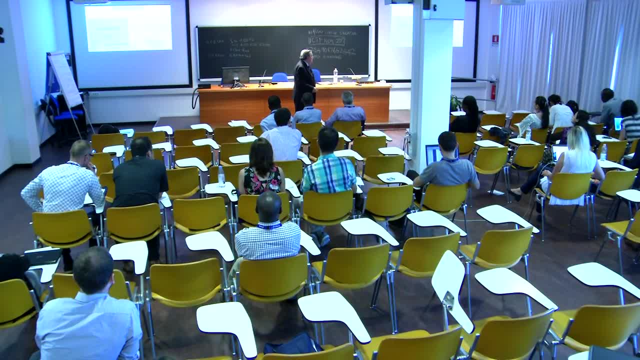 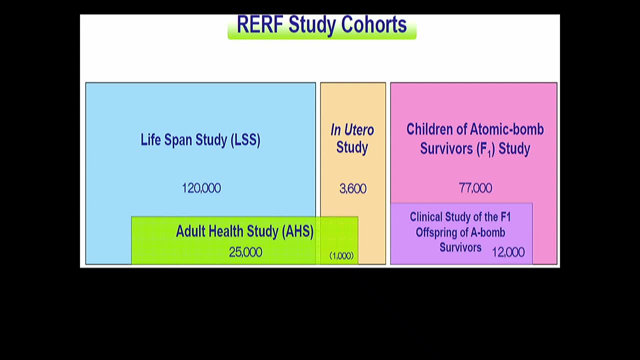 Really, what I am presenting to you is more updated information. This study includes 120,000 people for cancer and leukemia, People that were in utero at the time of the bomb, 3,600 for a lot of information, And children of the survivors. 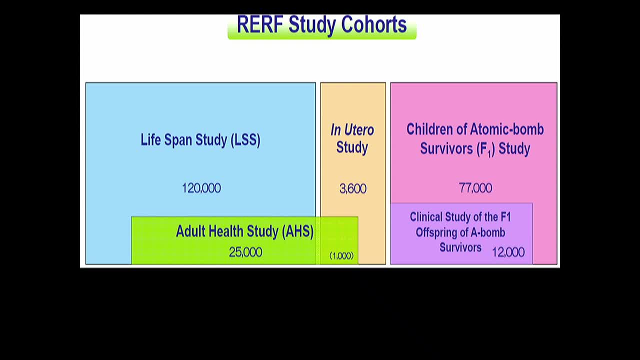 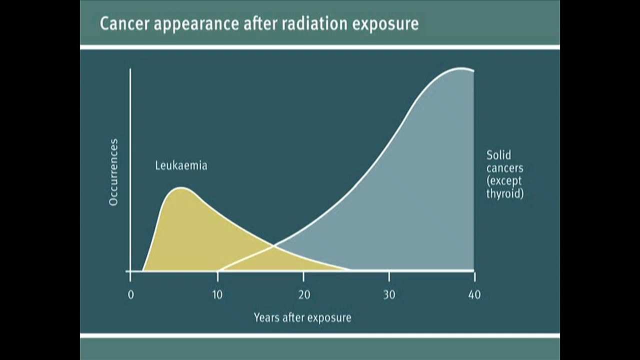 70,000.. For we can study cancers and leukemia, hereditary effects and antenatal Antenatal effects with very big, big population. Let me show you the result: Cancer- Definitely. there was an increase in leukemia that now has gone down. After the year, 10 years after the explosion, has been an increase in solid cancers. that still is there. This is crystal clear for high doses. Remember, after the nuclear explosion the doses were very high. At these high doses the mortality was in the order of 5%. 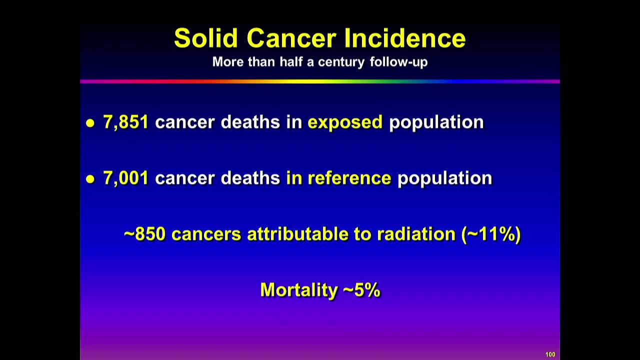 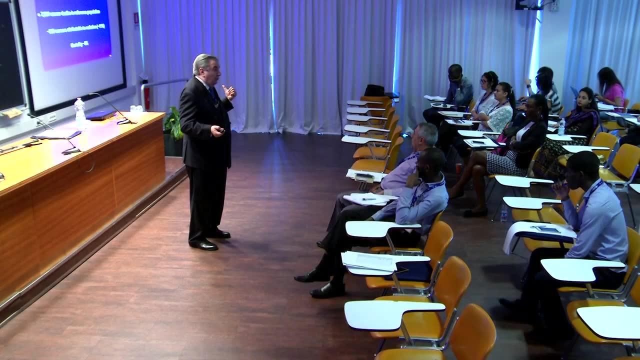 850 cancers, over 7,000 cancers. These were in the exposed population. This was in the reference population. From here you can get the conclusion: If, with a nuclear weapon, with this very high level of doses, you have only this amount of effect, 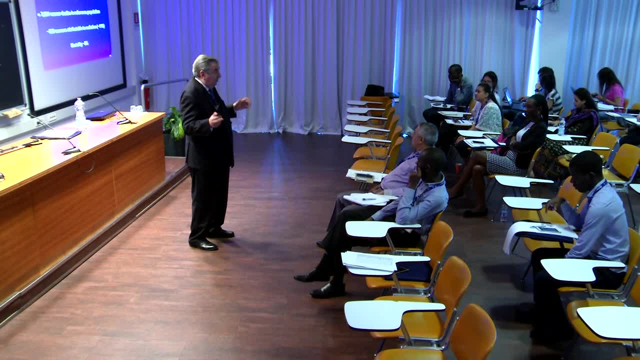 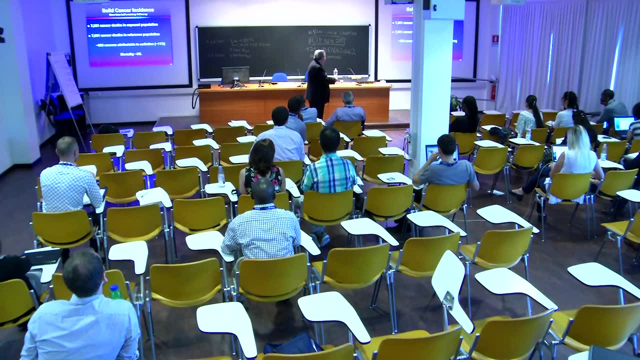 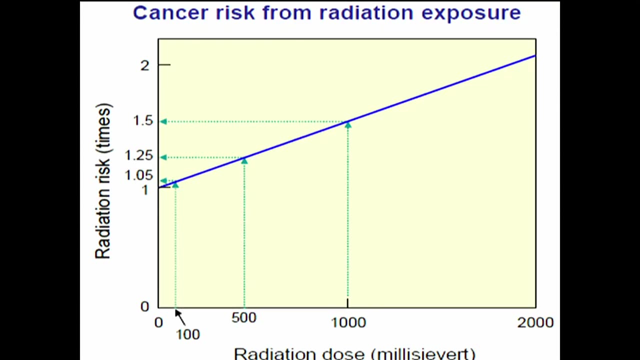 radiation should not, could not be so risky Because this was a nuclear weapon. remember, this was very, very, very high And the difference between normal cancers and cancers of people irradiated was relatively small. in proportion With this basis, UNSCEAR estimated the cancer risk. 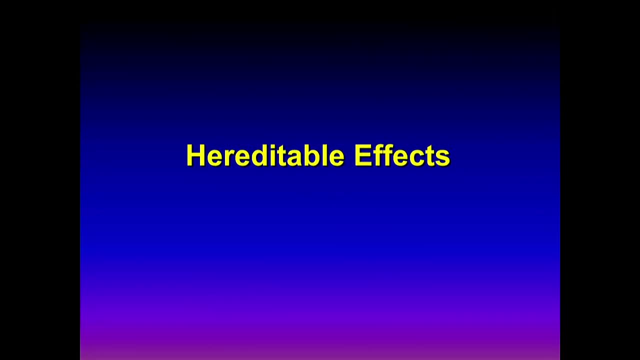 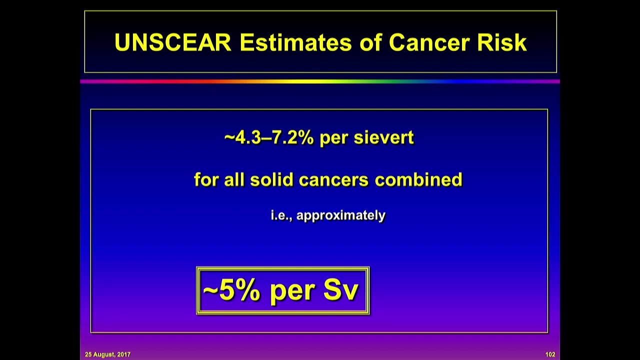 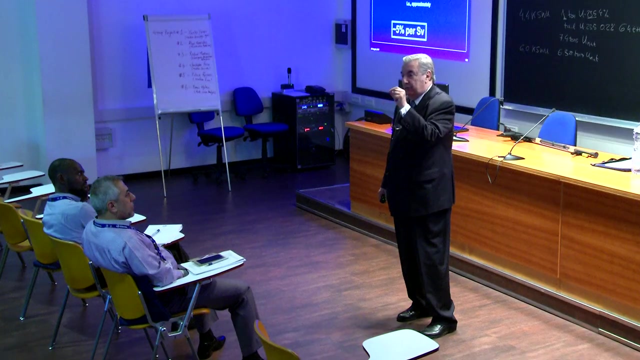 in approximately 5% per sievert. for higher doses, 5% per sievert, But it's a very low number. no, It's 5%, 4,000 millisieverts For a 0.005%, or you have to put another two zeros. 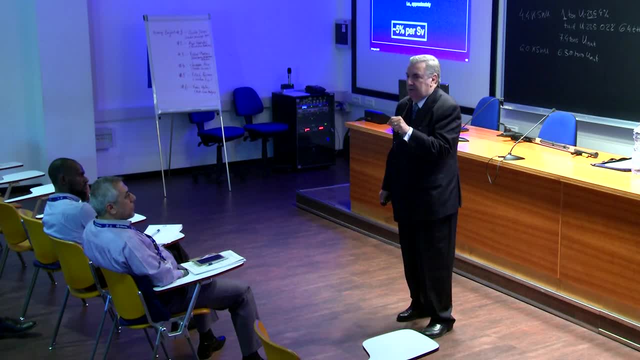 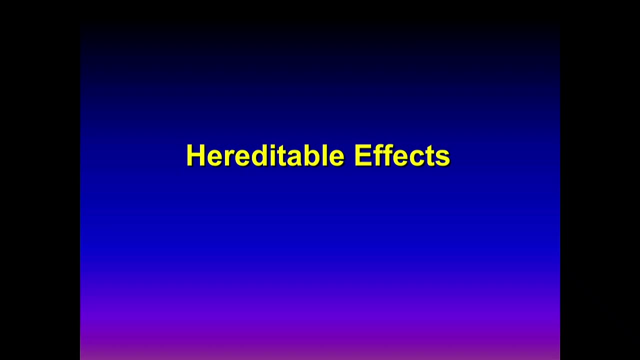 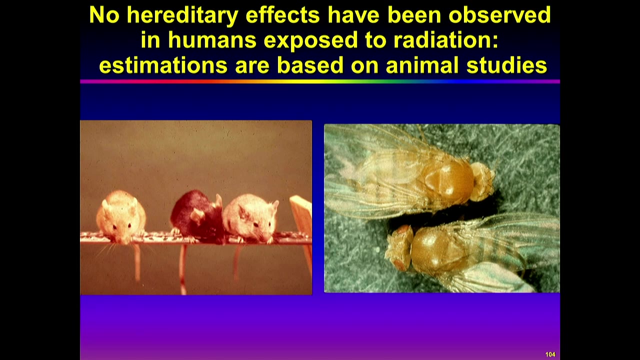 per millisievert, Very, very, very low risk. And the risk that is evident only at high doses. What about the hereditary? Well, we observe this hereditary effect in animals. we reproduce a lot, like the fruit flies, for instance. 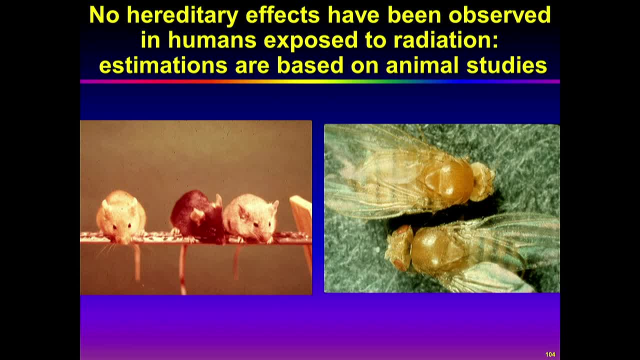 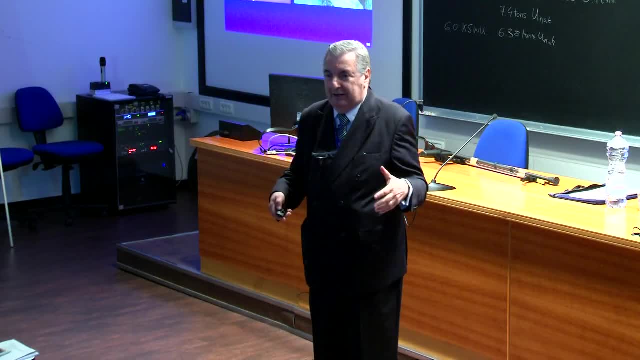 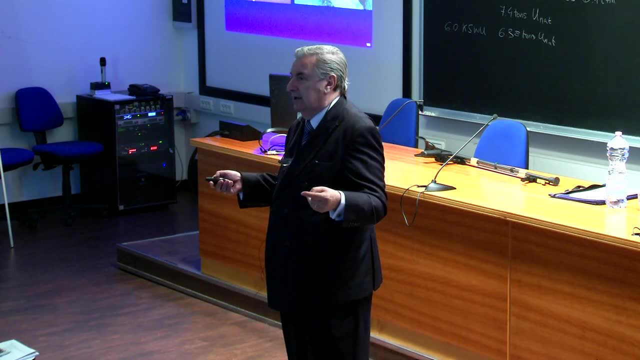 But in the big study of Fukushima we have been unable to see a single hereditary effect. For all the blah blah blah on Chernobyl and Fukushima of hereditary effects after the nuclear are wrong, An invention of the media. 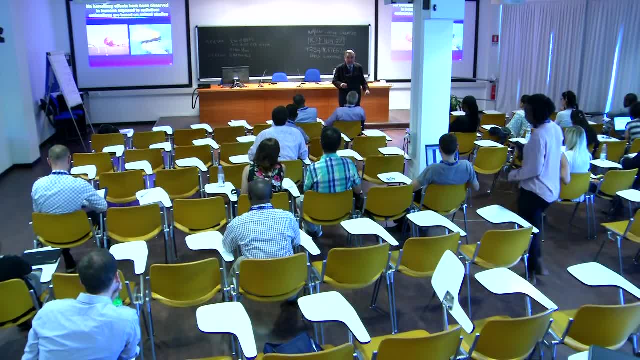 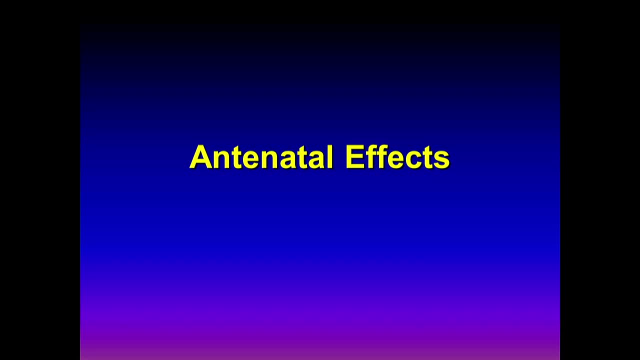 In Hiroshima, there was not one single hereditary effect after an study as big as the one that I showed Antenatal. Well, again, we have studied thousands of children that were exposed while in utero And we know that in this period of pregnancy. 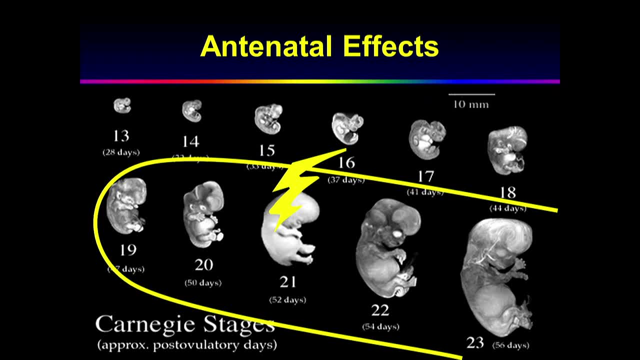 something should have happened with radiation, because in this period of pregnancy our computer here is being cabled, All the cells are being connected And if you affect the fetus at that time you can affect the connection. This is the reason why pregnant women 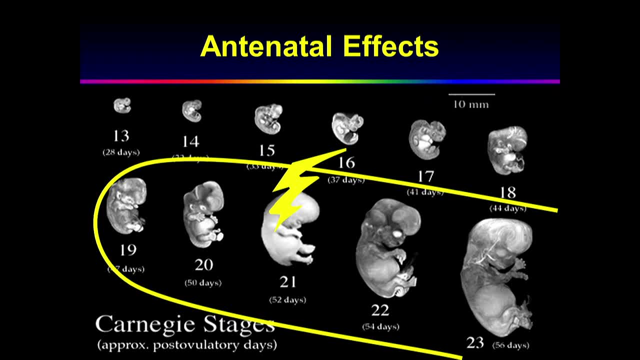 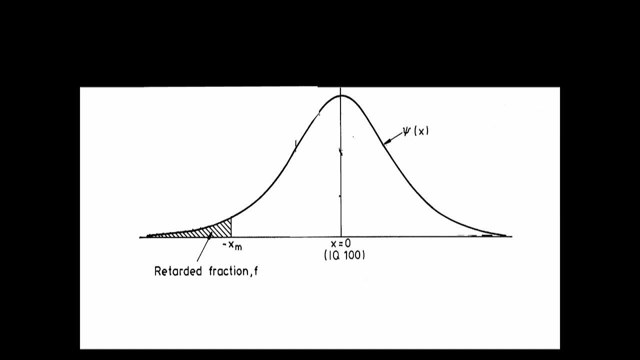 should not drink coffee or do things that can affect this connection, And we suspected that something could be, For this was very heavily studied by studying the IQ of the children who were born after being irradiated in utero. The IQ is a measure invented by doctors. 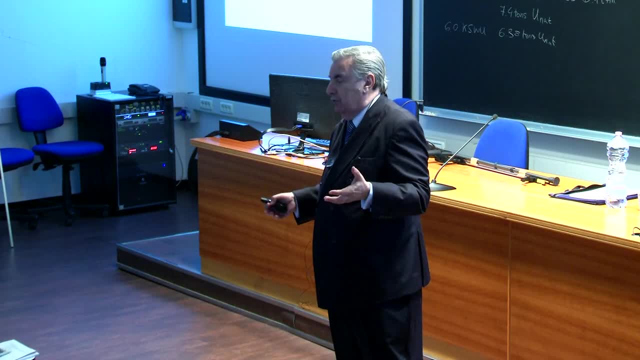 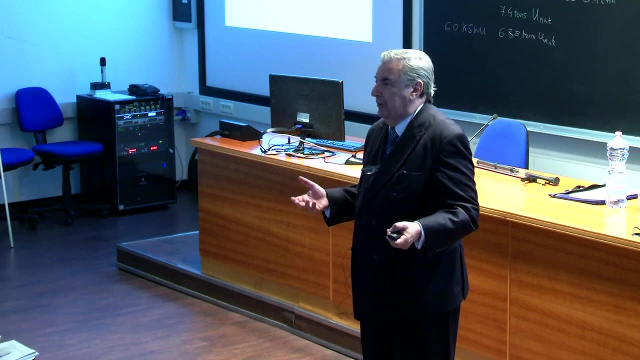 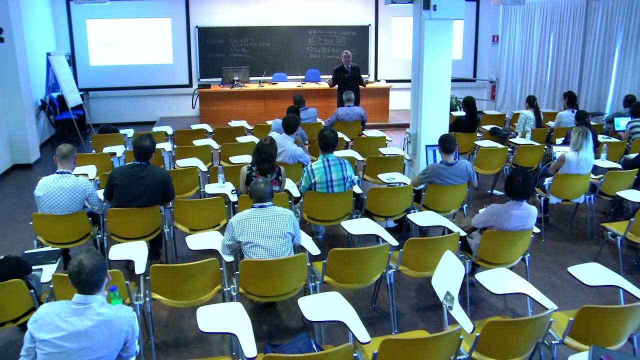 If you take a group of children that you see in one school, you measure the IQ following certain rules. A high IQ normally means that they are very good for mathematics. They are clever children. A low IQ normally means that they are good for playing football. 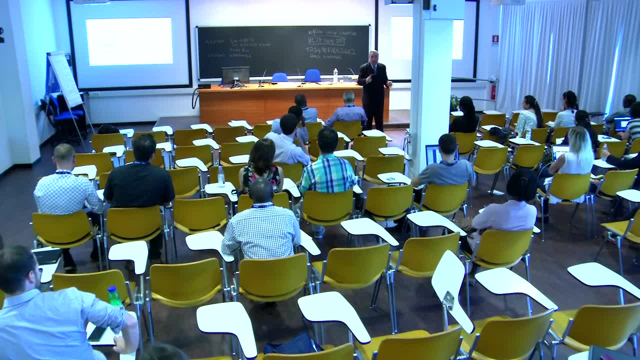 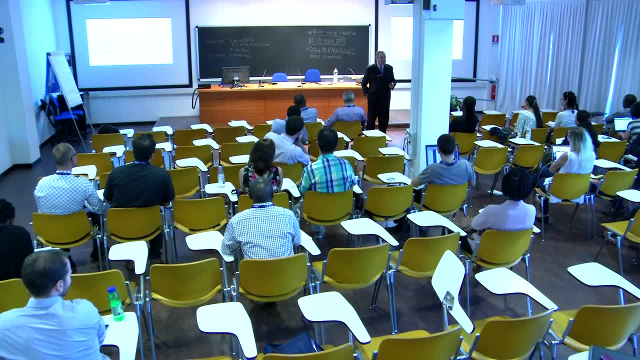 And usually the one playing football will get much more money than the one playing mathematics. Probably Messi was in this part and he's getting one million euros per hour or per week, every single day. And the doctors, just to confuse us again. 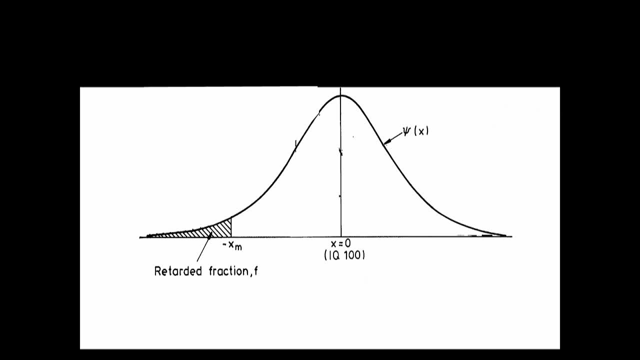 they call to the children that are in this area retarded fractions. Well, they are not retarded children, I tell you. They are children that are not good for mathematics, basically. Well, we measure this IQ following these rules And what we discovered, 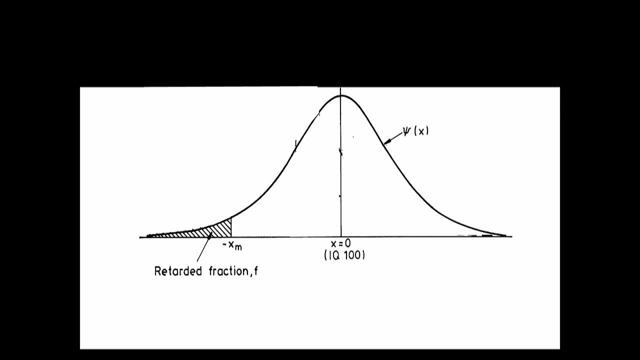 is that these children in Fukushima exposed to a very high dose when they were in utero. the IQ moved to the left, for the so-called retarded fraction was a little higher, But the doses at which this happened was 1,000 millisieverts. 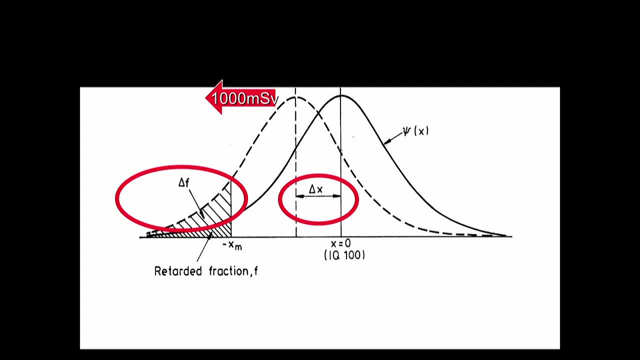 a very high dose And low doses. they were not the effect of the children's irradiated in utero. Again, this is very important because women in particular are very concerned And this has done a lot of damage, One of the biggest damages. in Chernobyl- for there was no like that in Fukushima- was that practically all pregnant women decided to abort because they were so afraid. But it's convenient to know that radiation at low levels does not produce this antenatal effect At high levels. yes, 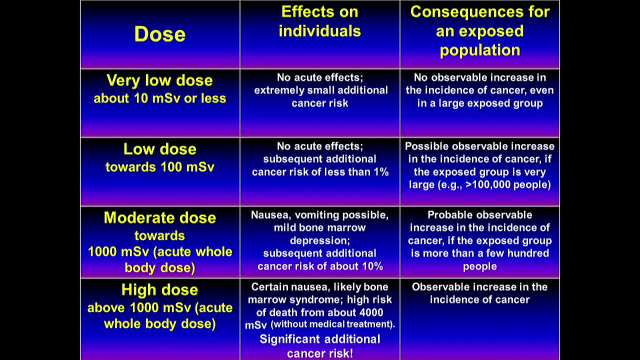 Takeaway points I will give. There is a table that you have there that gives a good summary of low doses: nothing Up to 100 millisieverts. something appears Above 1,000 millisieverts. yes, appears the effect. 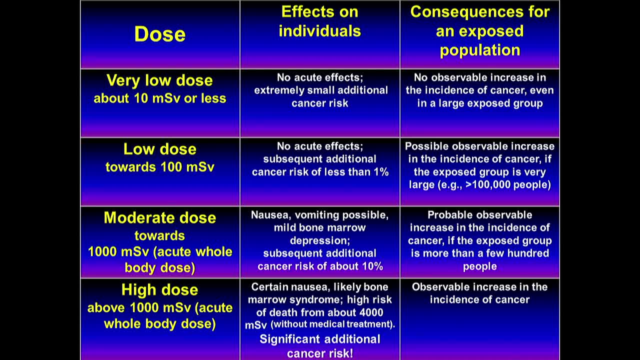 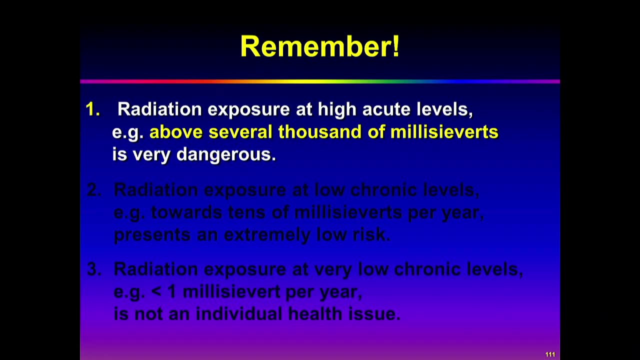 High dose is above 1,000 millisieverts, where you have the real effect of radiation. Well, this table shows you that the real problem of radiation is in the top, not in the bottom, Sorry. Yes, Remember radiation exposure. 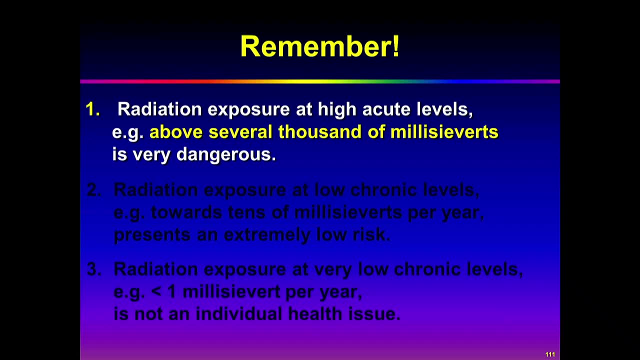 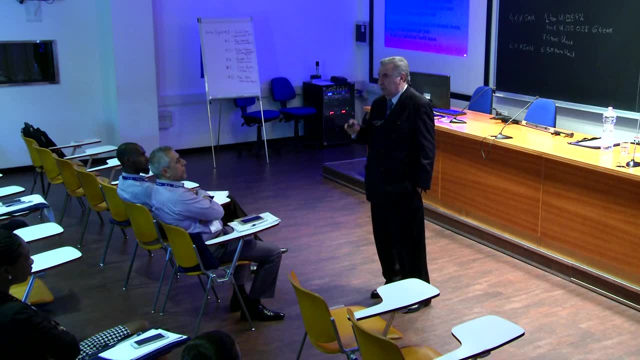 at high acute levels. yeah, this is a very good point. It's a mistake that. It's a very common mistake in our profession. Every time that we use the word dose, normally what we meant is effective dose, But we don't say it. 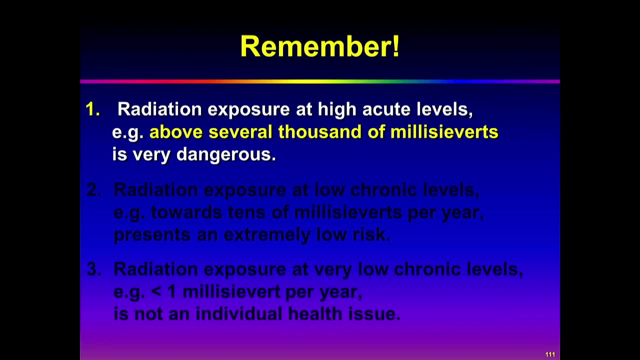 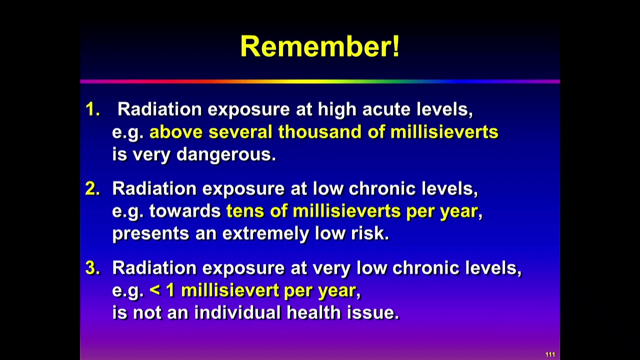 And that is It really is a mistake. At high levels it's very dangerous. At low chronic levels in the order of 10 millisieverts very, very low risk And at the level of our operation it's not a health issue. 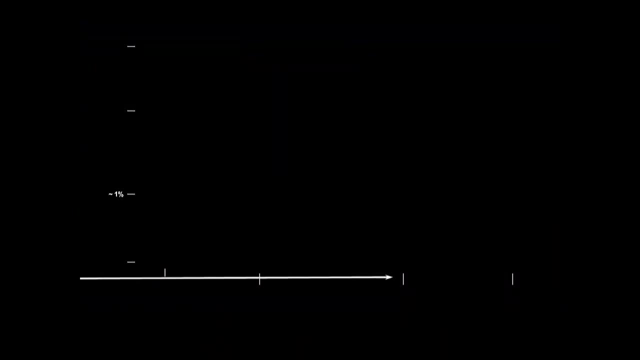 This is basically the conclusion that you have to have in mind. I tried to put in a table, in a graph, what I have explained to you. First of all, at one sievert, 1,000 millisieverts start the tissue reaction. 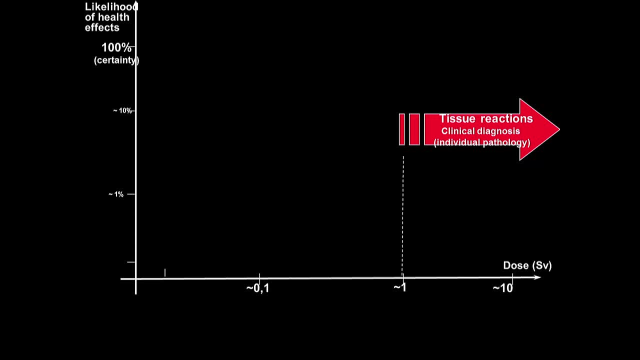 Clinical diagnosis, individual pathology and the probability of getting this increased very quickly. with dose At around 7,000 millisieverts, you will die. I know only one case in the world that got that dose and was saved. It was a Russian in Chernobyl. 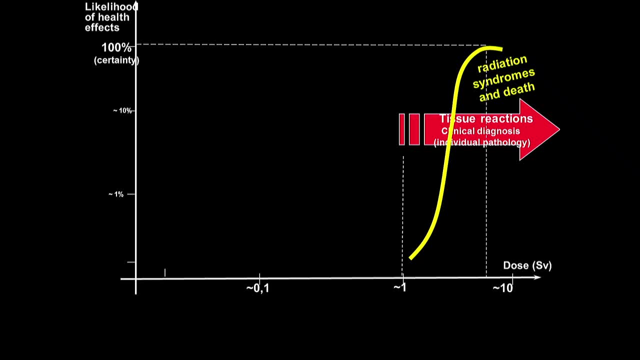 because he was attended in one of the best hospitals in the world and with the best radiopathology. at the time It was Dr Angelina Guskova, But I'm scared to tell us also that at 1,000 millisieverts- 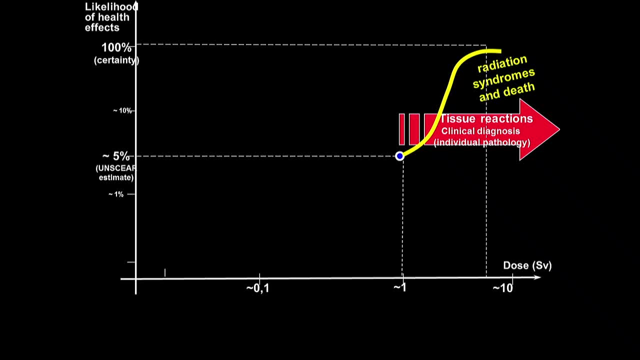 there is an increase of getting cancer of 5% per millisievert. Remember, this is logarithmic, logarithmic, logarithmic Below here, and it's important to say below here, because this is a limit of pathological knowledge. A pathologist doesn't know anything. 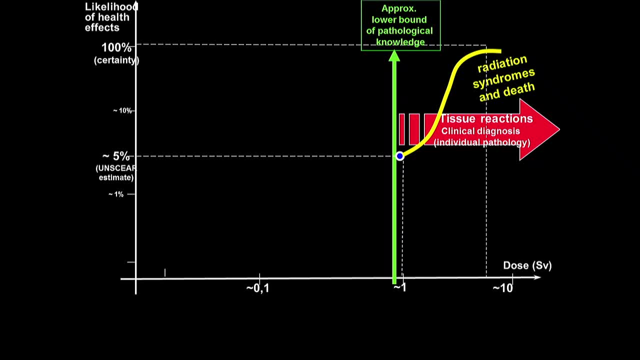 below there. For when a doctor says, no, you are okay. blah, blah, blah. 1,000 millisieverts pathology. you cannot see anything Below this. there is an increased incidence of malignancies. We know that. 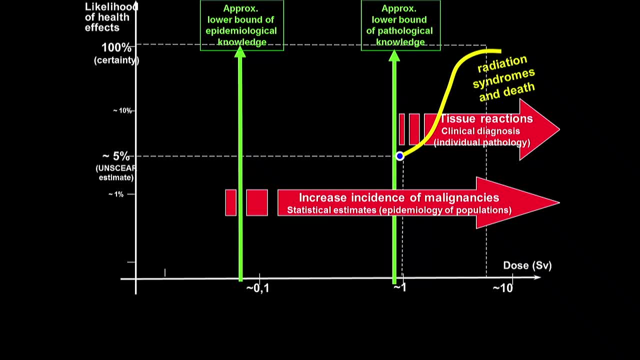 And epidemiologists start to see this around 100 millisieverts, above 100 millisieverts, And the increase is more or less linear. Epidemiological assessment, therefore, is between 100, above 100. But below 100, we do not have any data. 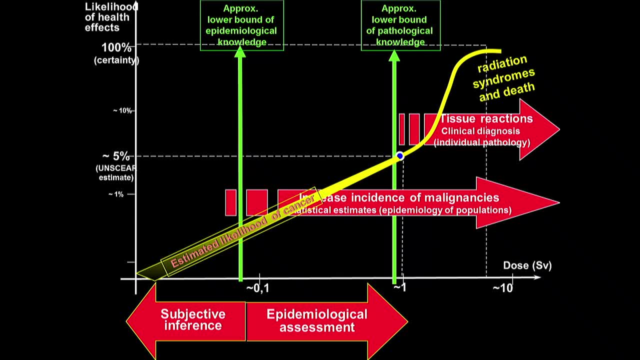 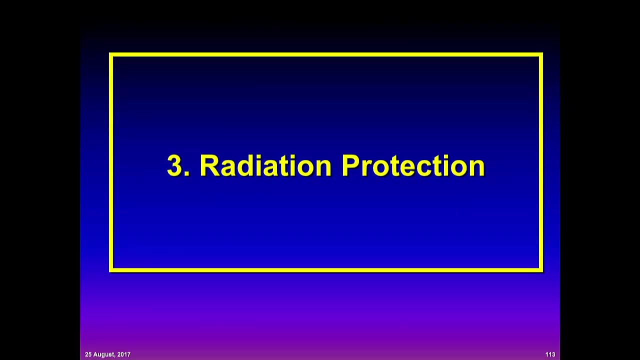 We have subjective inference And this depends on the person who made inference. inference Above 1,000,. yes, you have individual diagnostics by pathologists. Please take this in mind, because it's important. what is coming Now? let's go quickly. 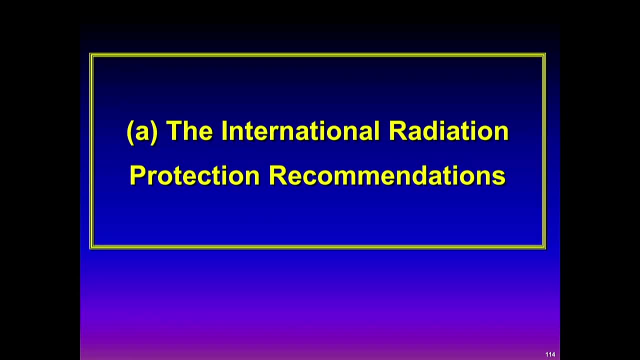 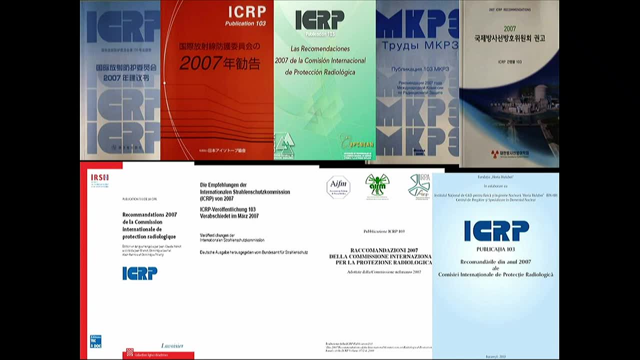 through radiation protection. The international recommendations in this document of ICRP. all of them are in many different languages. I can get a copy in the language that you prefer, except in English. In English you have to pay, But in all the other languages 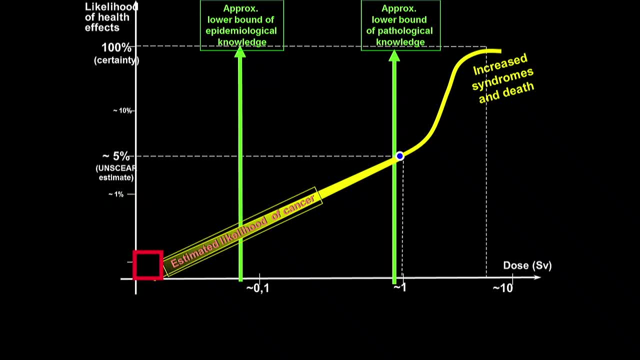 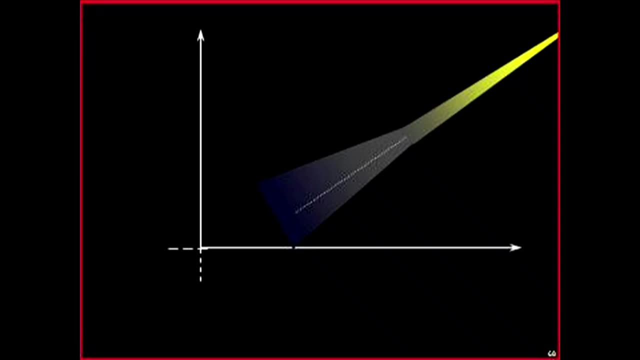 it's free of charge. The basic paradigm is what you do here, because the doses that we are working are there, not in the top. Here we don't know anything really. There is no data. You need to have a subjective inference. 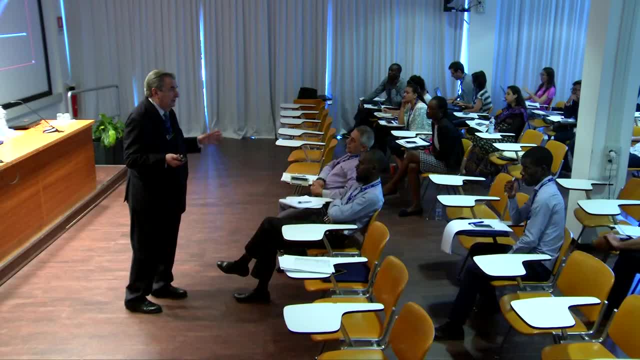 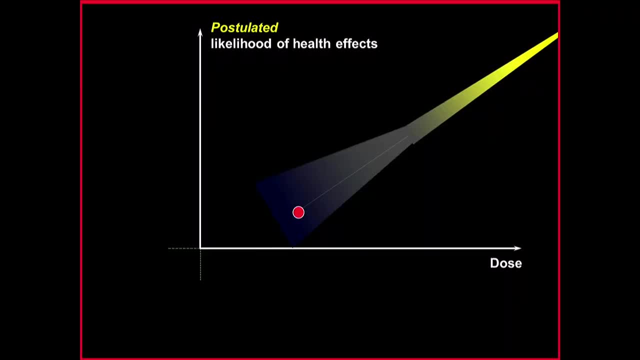 I tell you what ICRP has done can be criticized. The paradigm ICRP took is the following: Above background, which you saw, is very high, above background dose can be up to 100, and above background dose can be up to 100. 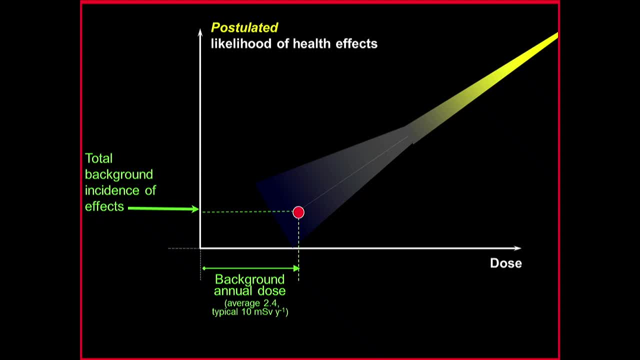 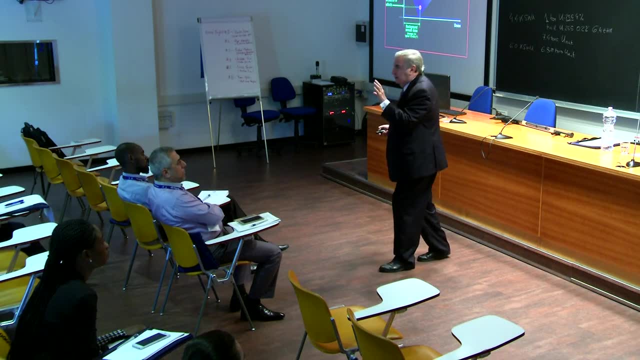 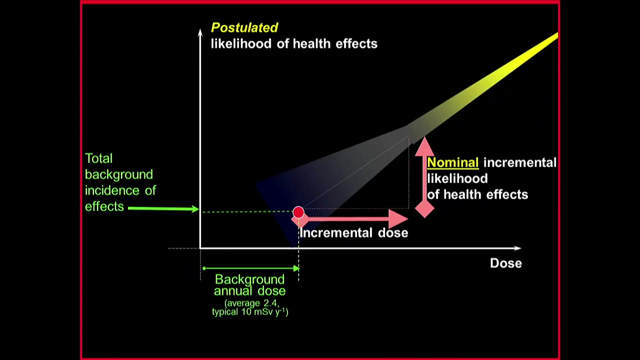 The incidence, which is also very high, 25% above that ICRP said. for protection reasons, for ethical reasons of protection, you have to assume that an increment in dose may produce a nominal increment in probability. You cannot prove that. 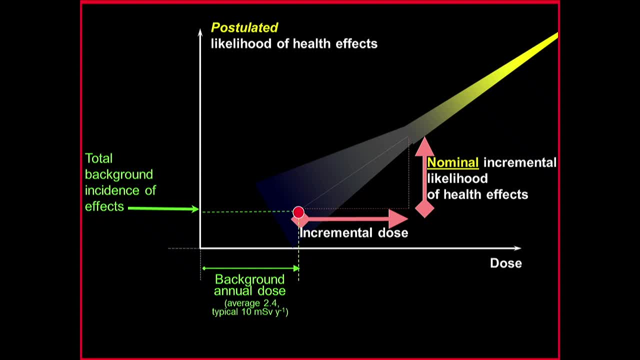 It's just an ethical approach. You can say: well, this is a nominal risk factor And the relationship between this and this is called nominal risk factor And the radiation protection is built above this paradigm, which has no basis in science. It's a subjective inference. 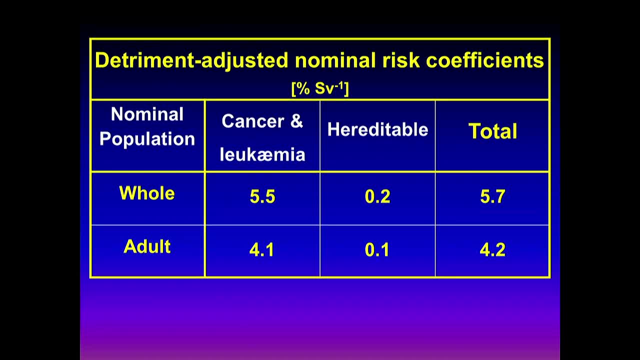 Of course it's not like that. I mean there are reasons for it, but the risk factor here for the whole population is in the order of 5%. Look, this risk includes when we know that there are not, but since we don't know, 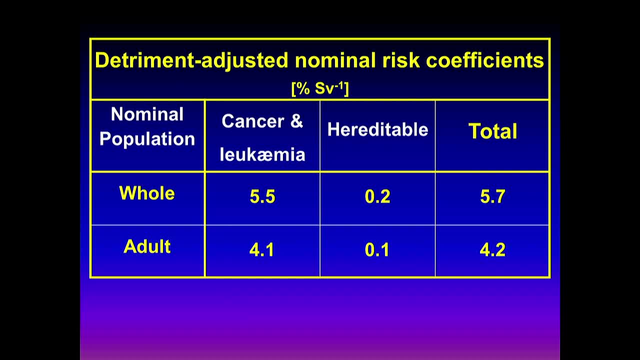 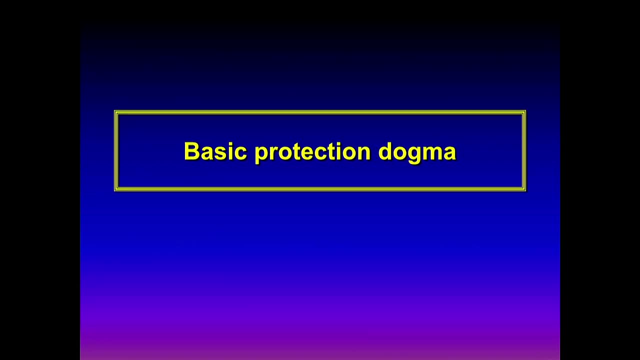 whether it may happen in big, big populations. we put the risk factor here: The whole and the adult. The whole is bigger than the adult because it includes children. The whole is bigger than the adult because it includes workers, Radiation protection in practice. 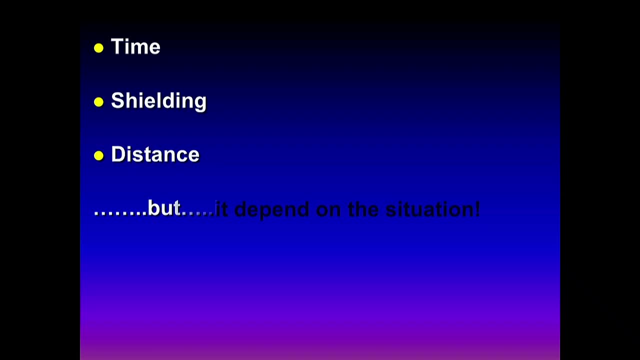 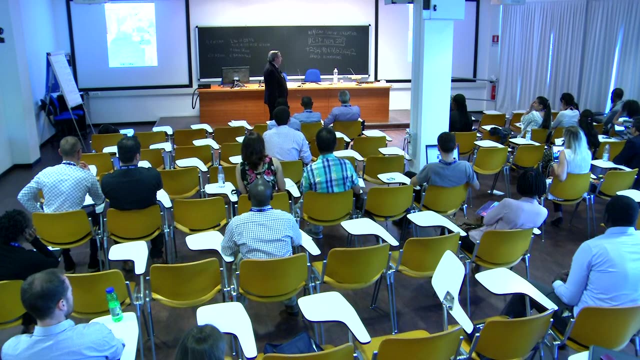 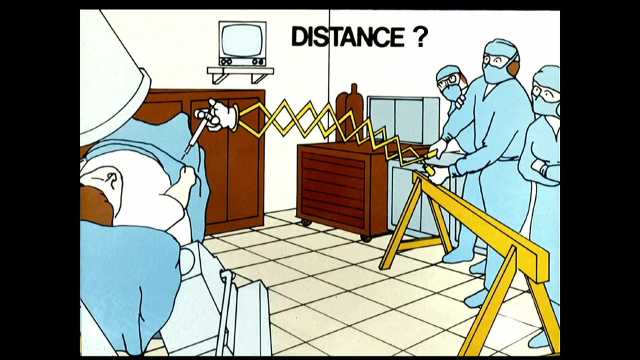 has a basic dogma: Time shielding distance. But of course this depends on the situation. It's not so easy, For instance, for medical doctors. do you believe that the doctor can work like this, To shield or to take distance? 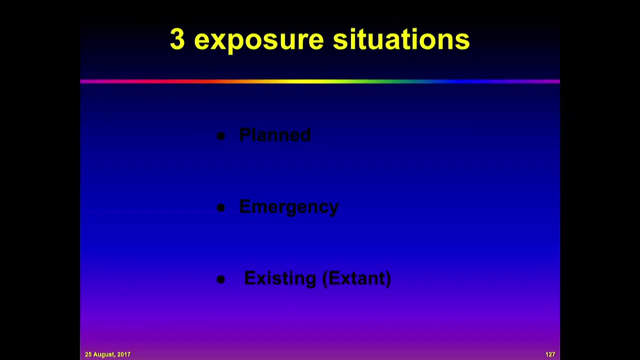 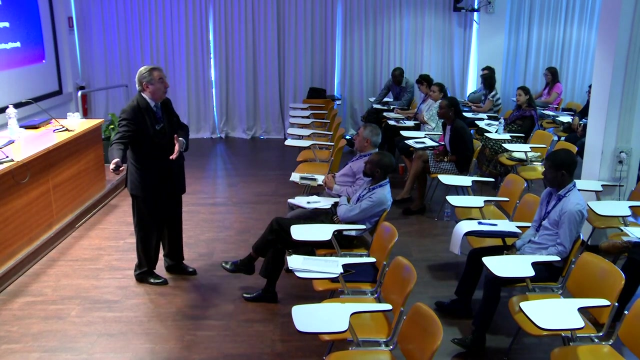 Under this situation, we created three exposure situations: Planned, emergency and existing Planned. when you can plan and you can decide what to do. Existing what is there? You found it. The people in India found Kerala Certainly not. 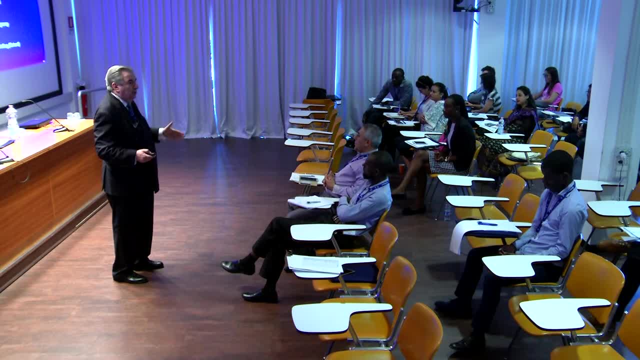 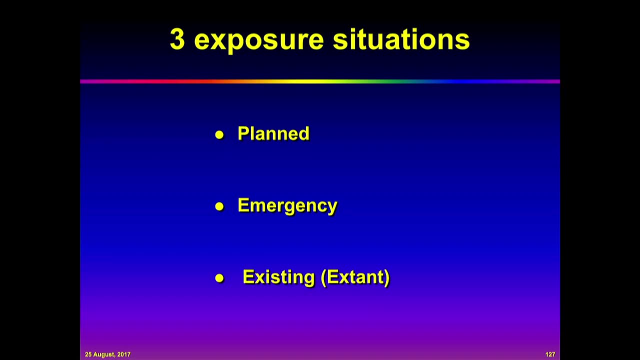 We will evacuate La Paz, the capital of Bolivia, with two million inhabitants, Or emergency. By the way, we use the word existing, but really the proper word in English is extant, not existing. This was a big mistake, because the Americans told me that. 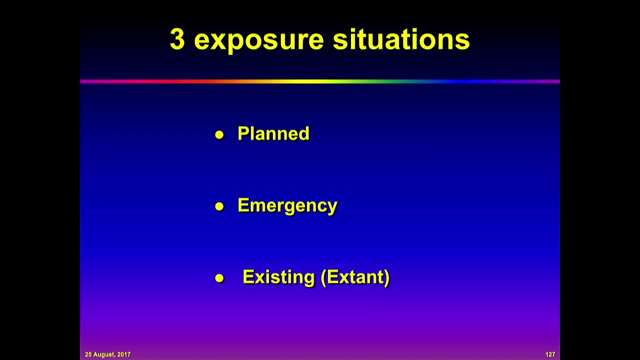 extant, never crosses the North Atlantic. It's a word that you can understand in England but not in America. An emergency? Well, the emergency has happened. You have the emergency, You have to do something, not that you plan it for the emergency. 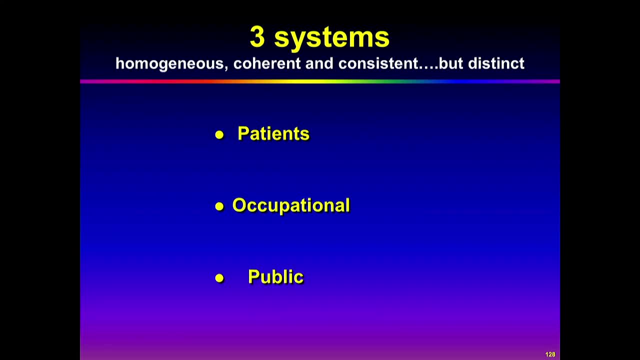 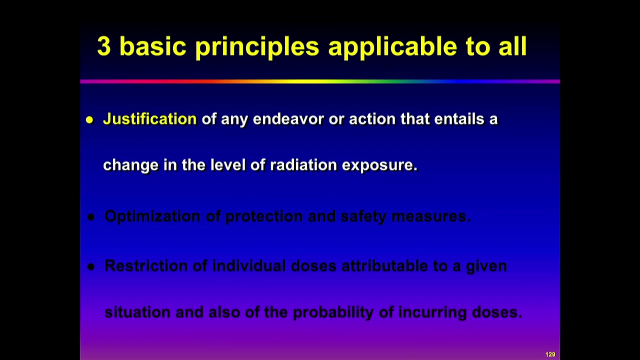 We have also three systems: One for patients, one for the patient and one for the public. Different subjects, really. The patient is getting benefit from radiation, The worker also, and he knows the public doesn't know what to do. The basic principle applied to all. 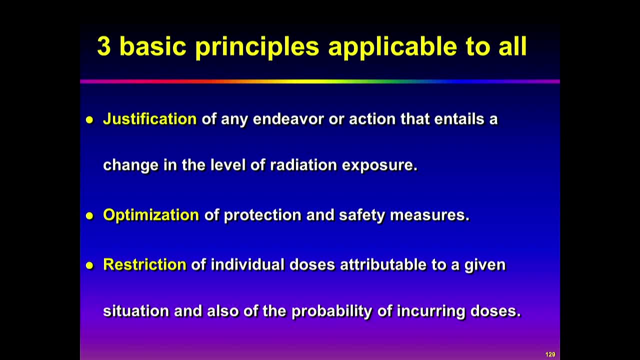 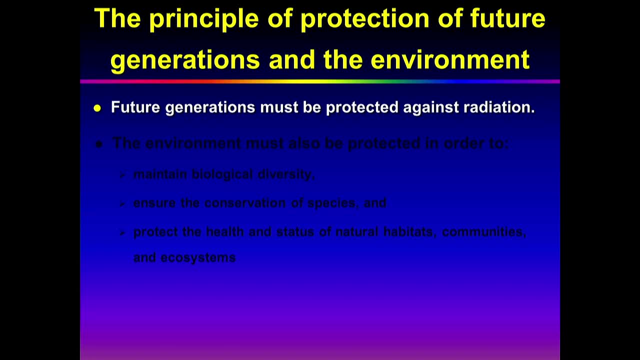 is justification, optimization of protection and restriction of individual doses, And the additional principle introduced by the agency is protection of future generations and the environment. The question of the environment is very cultural, you know. I always ask the environmental people: what do you mean by environment? 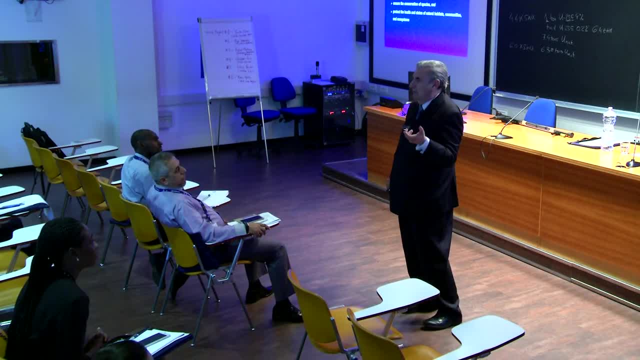 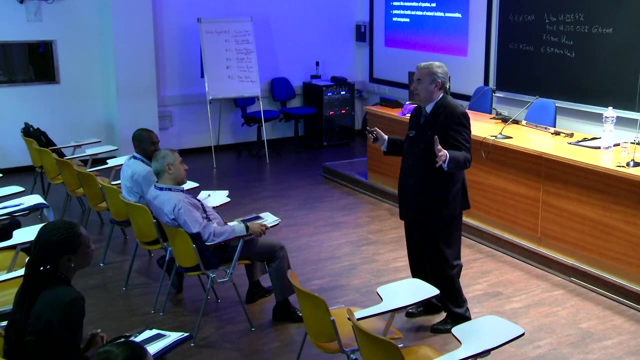 If I have a mosquito in my room, that mosquito is the environment. In that case, you don't protect the environment. If I have a mosquito in my room, I kill it. Or you want to protect the spice that feeds mosquitoes. It's a different thing. 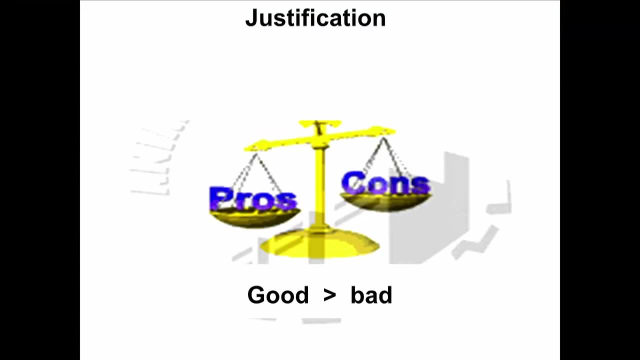 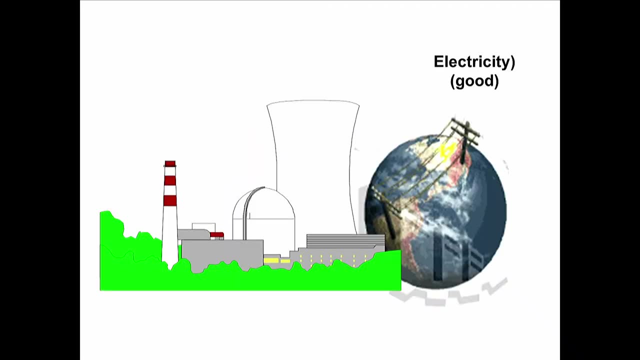 It's not well defined. the environment Justification is a balance between good and bad. For instance, a nuclear power plant produces bad releases And your role is to make that installation will be justified if the good is bigger than the bad. 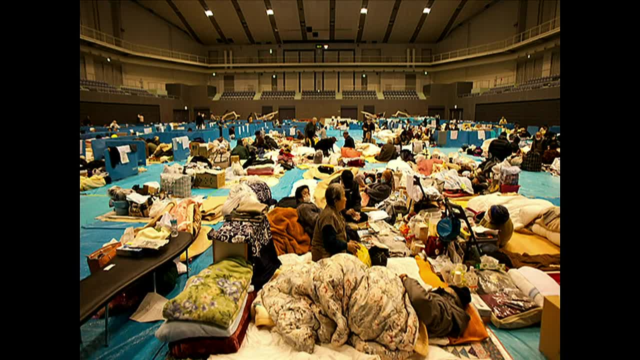 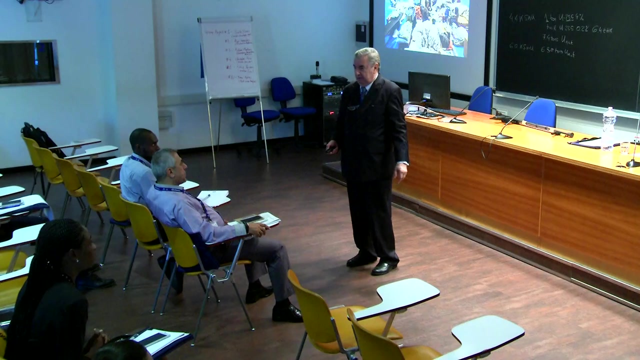 Very difficult to balance. But justification is also justified for inter-evacuation of people. Was evacuation justified in Japan? You know how many people died because they were evacuated. Serious problem? Very easy to say no, it's a little radiation. 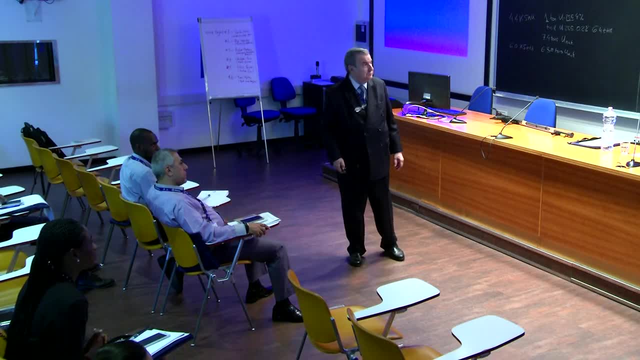 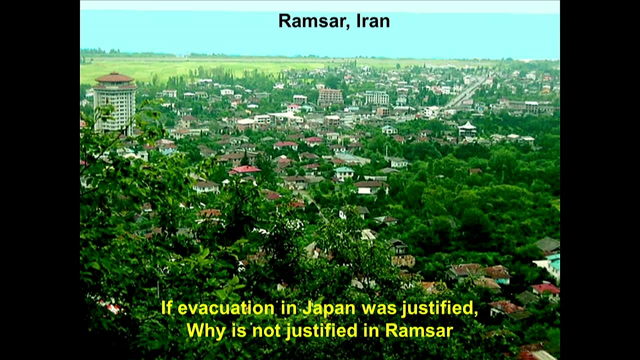 Evacuate everybody. When you evacuate people, people die. For instance, this is the city of Ramsar. If evacuation in Japan was justified, why we don't evacuate Ramsar? Look, the people of Ramsar will believe that we are crazy. 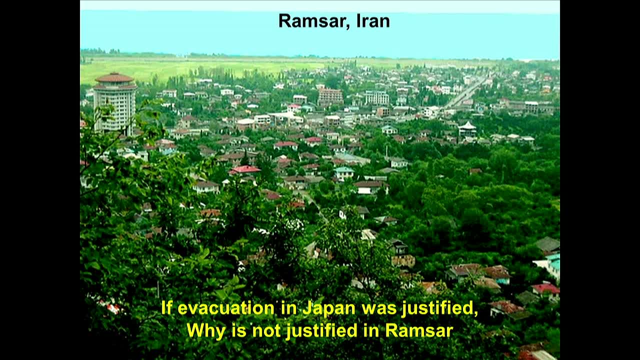 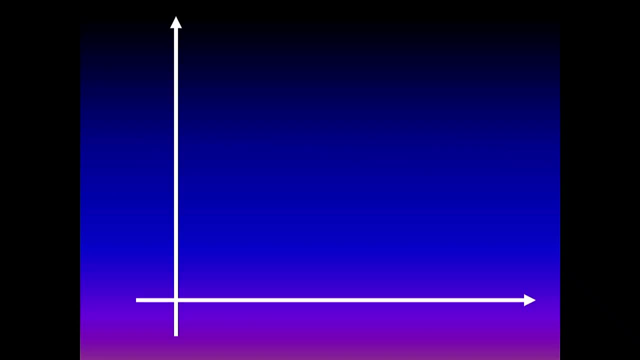 This is a beautiful city. They are having caviar there, but they don't want to evacuate Optimization: Optimization means do the best under the prevailing circumstances To make it short. if you plot the level of protection, as much protection you put. 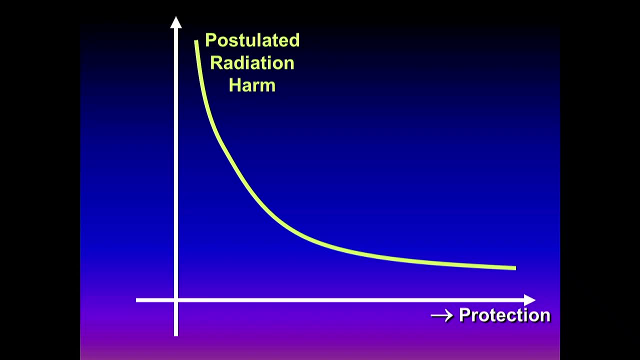 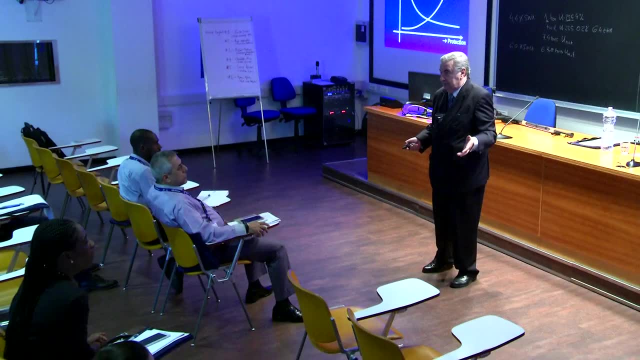 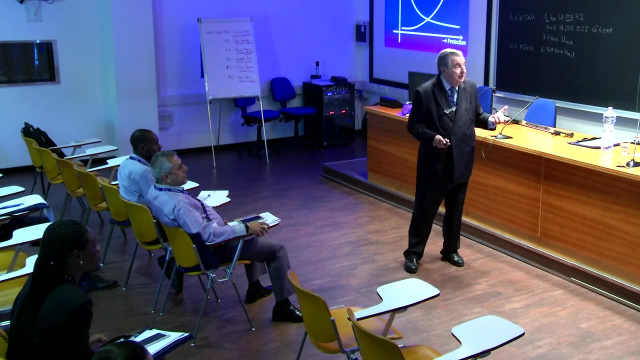 the harm will be lower, lower and lower, But the societal effort will be higher, higher and higher, And societal effort means social harm. You kill people. Optimization tells you: try to balance these two types of things. If you put the two together, 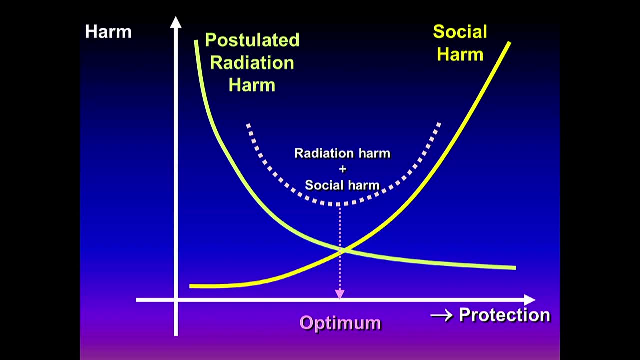 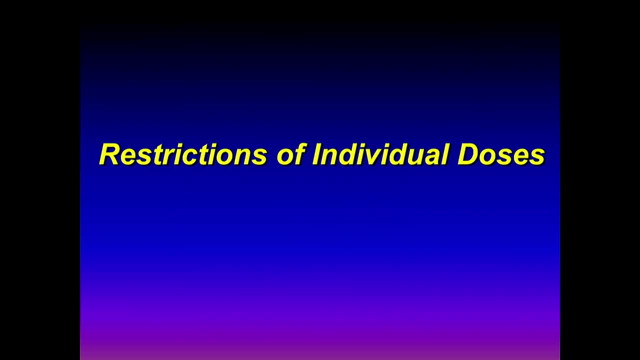 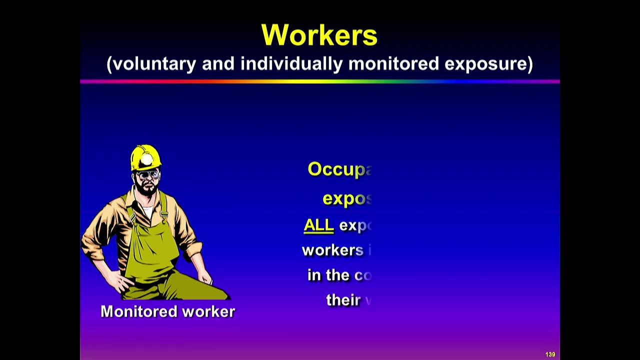 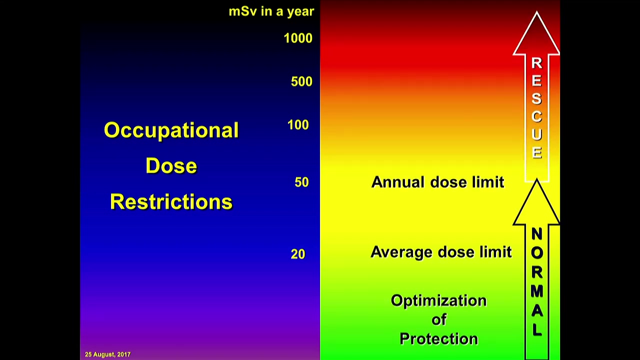 probably the one that gives the minimum. the optimum is the result of optimization. This is, in a few words, what optimization means. And then restrictions of individual doses For workers, who is voluntary, can be controlled. These are the standards in this moment. 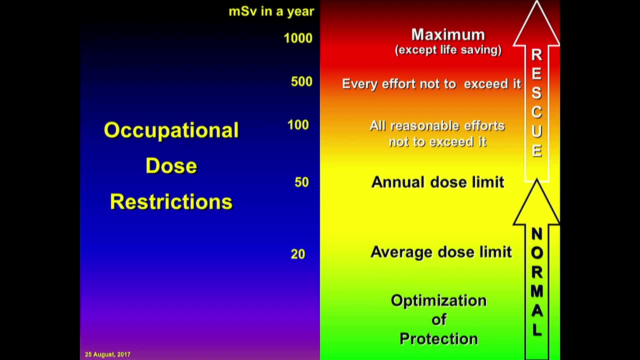 50 millisieverts of annual 20 of average optimization below, except for rescuers, who can't receive high dose because they're rescuers. Nobody asks him to be a rescuer. Nobody asks somebody to be a firefighter. They know that they have more risk. 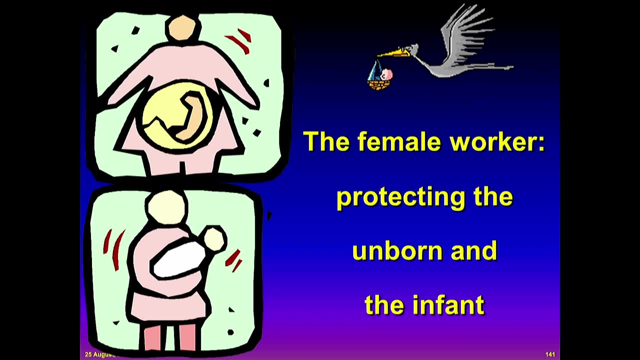 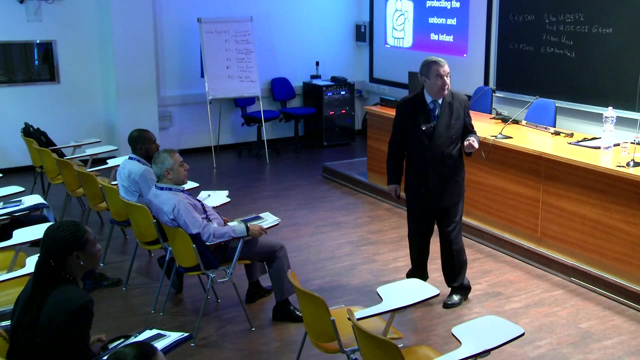 They do it because they like it, because they want to. The female worker is especially protected because of the problem that we mentioned: The unborn. not only the unborn, also the infant, because one typical case is the female worker getting contamination passing to the child. 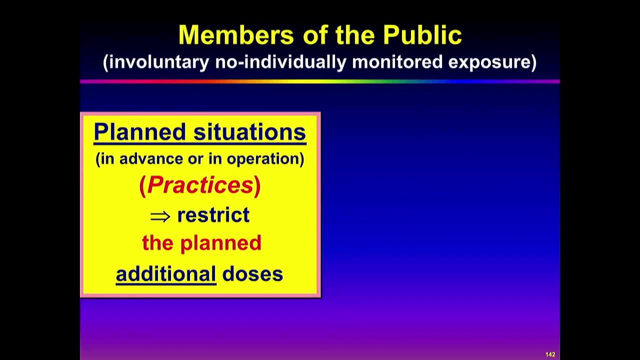 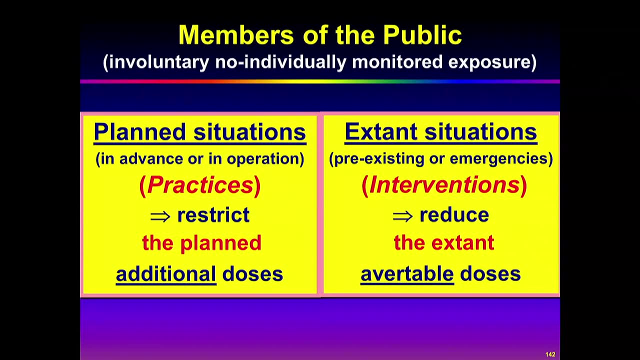 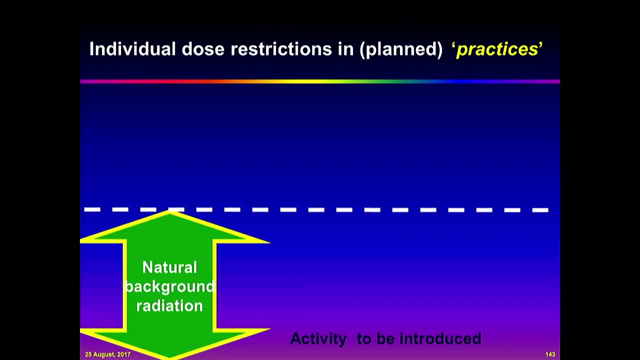 by giving milk, breast milk. They are in a planned situation where you can restrict the planned additional dose, or in an exhaled situation or in intervention. The situation is what it is. In a planned situation, you will have natural background, you introduce an activity. 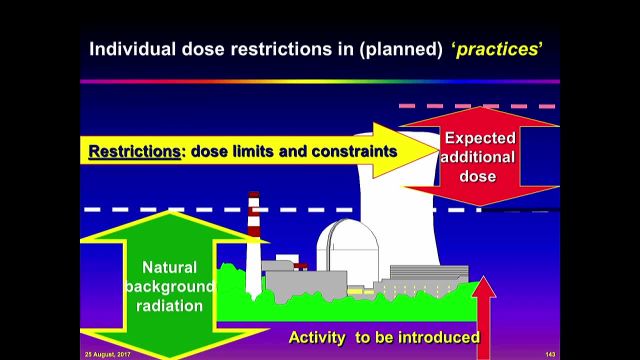 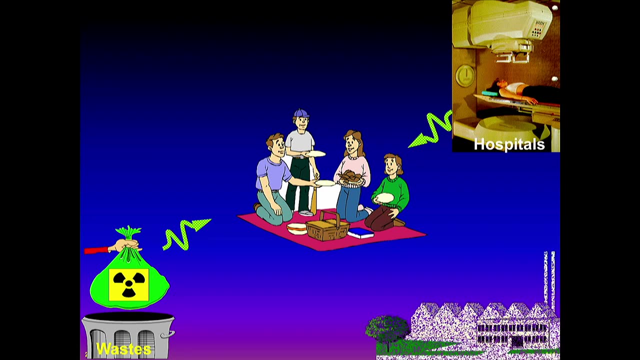 for each nuclear power plant and you know that the doses will increase- very little but will increase, and you have to apply restrictions. These restrictions are called dose constraints. Why? Because the dose limit applies to the radiation from all controllable practices. 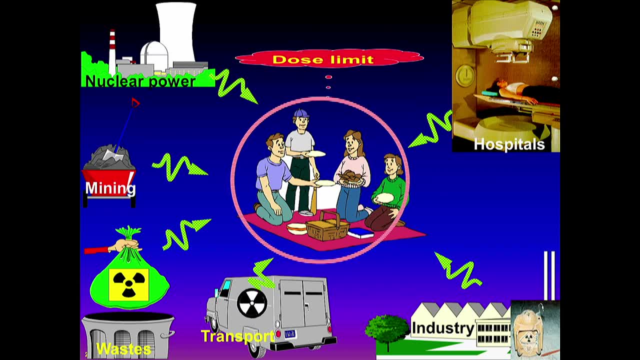 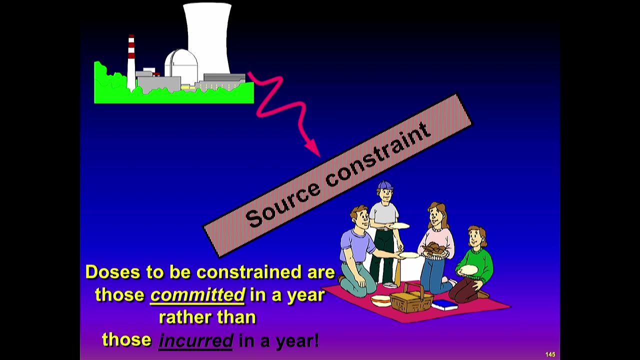 all the things that the authorities control. they have to apply a limit to the radiation of all this. To be sure of that, every part has to be constrained, and they apply a dose constraint to a given installation which is normally lower than the dose limit. 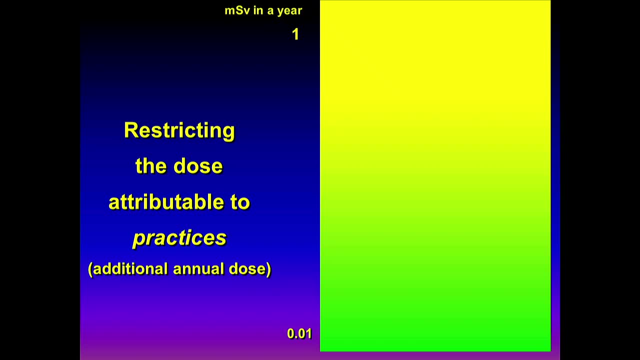 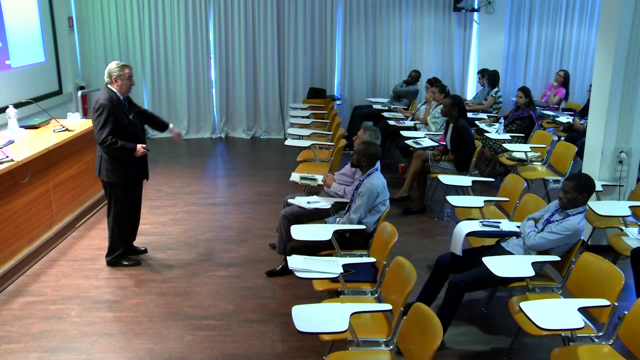 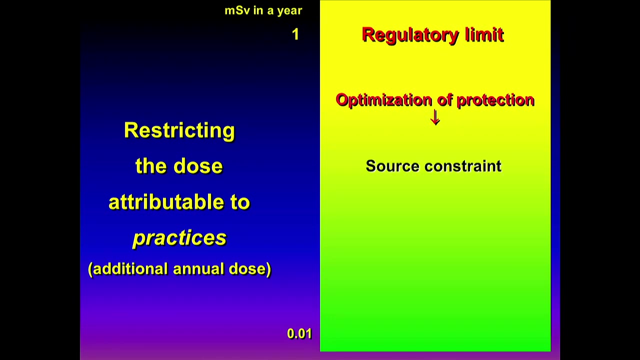 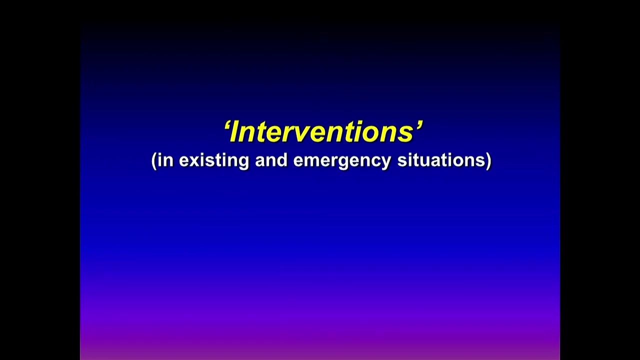 The values in international standards is one millisievert per year for dose limit. Remember that background is more than that, but this is the delta above background. This is the regulatory limit. optimization below the dose constraint is normally one-third of the limit. 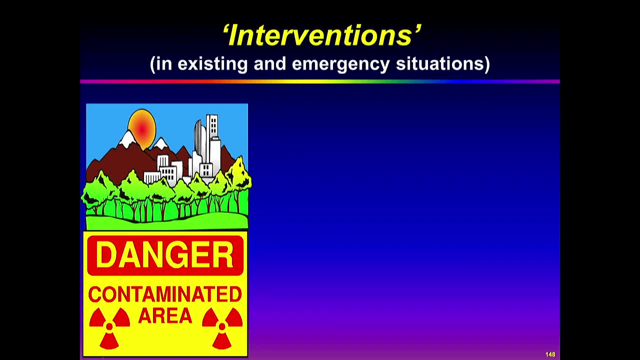 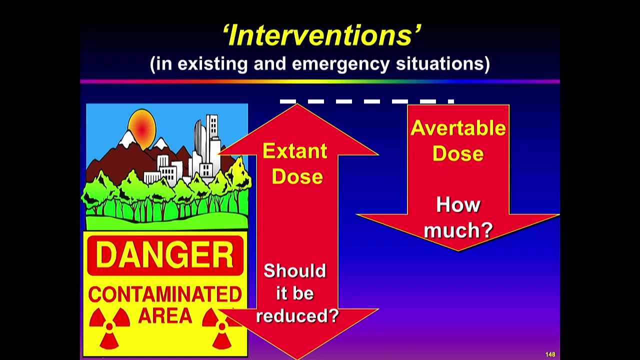 but in an emergency or existing situation, you don't have extra dose to control. What you have is an extra dose, and you as yourself. should it be reduced? Well, if you can reduce it, the answer is yes. how much do you have? 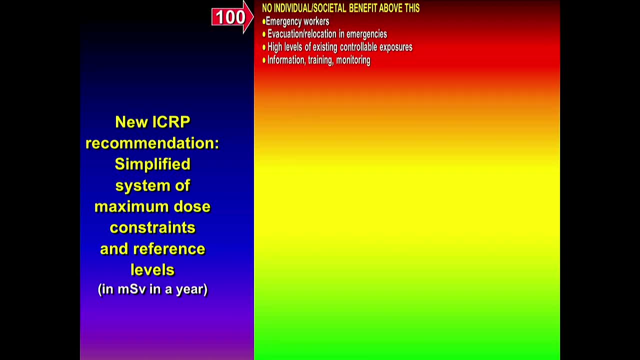 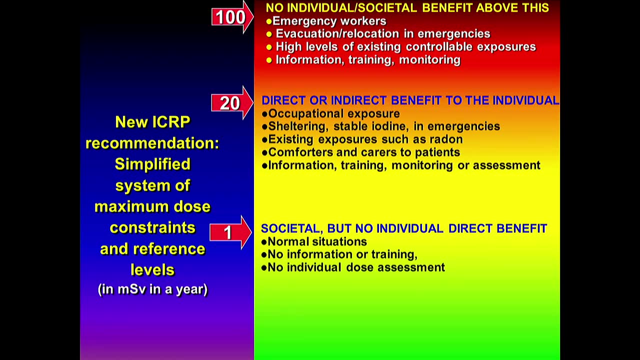 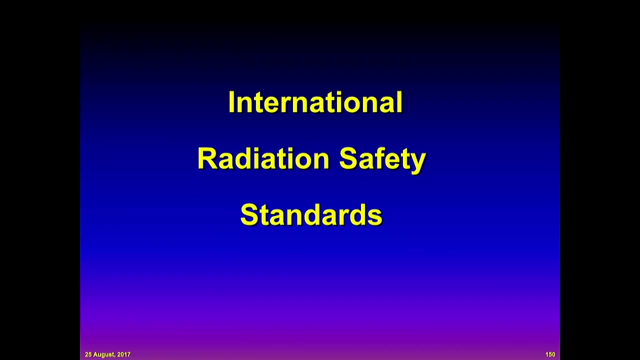 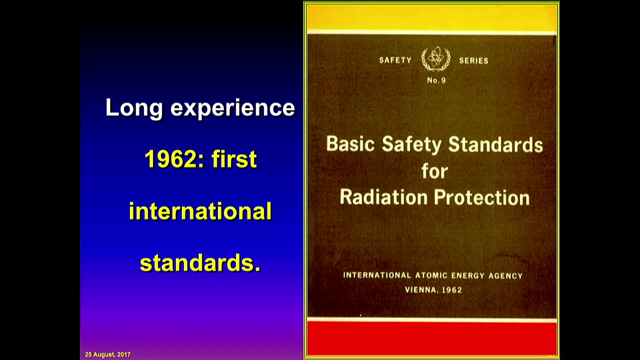 to avert the dose. Well, ICRP has recommended a number of levels for this situation, going up to 100 millisieverts per year. The international radiation safety standard has taken all this philosophy and included it in the standard. They have a lot of experience. 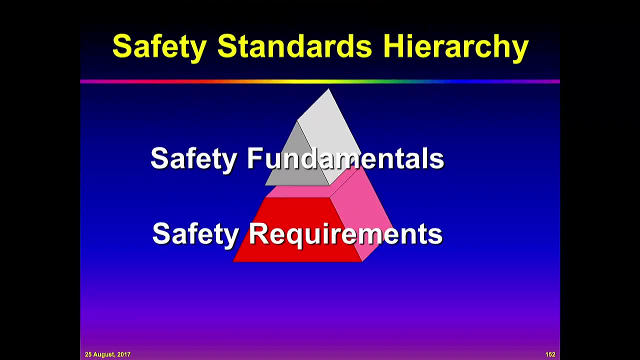 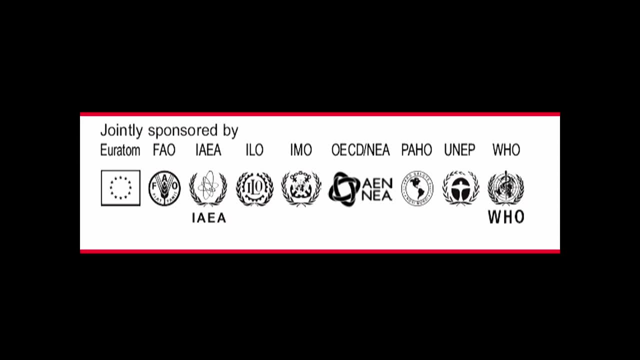 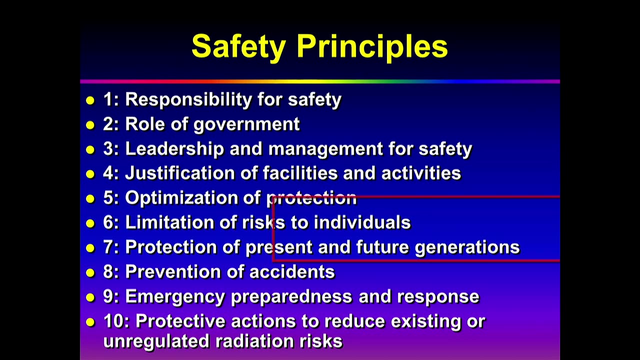 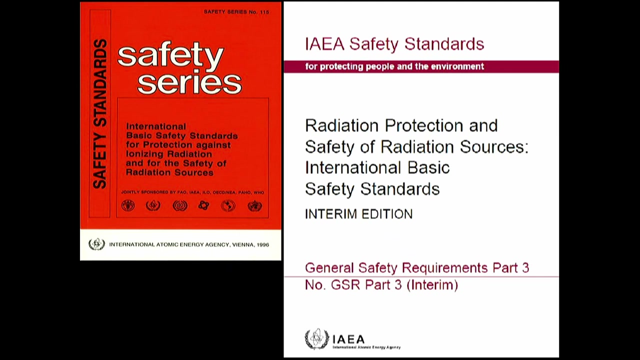 the agency. there is a hierarchy of the standard- you saw that yesterday- and these hierarchies, supported by all international organizations, include ten safety principles, four of which come from the radiation protection area, and the radiation protection standards are these two: the red one is the old one. 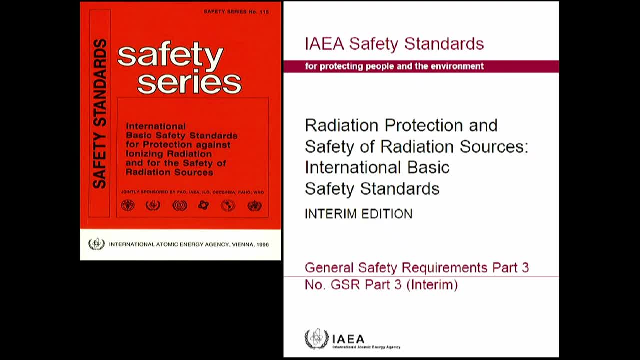 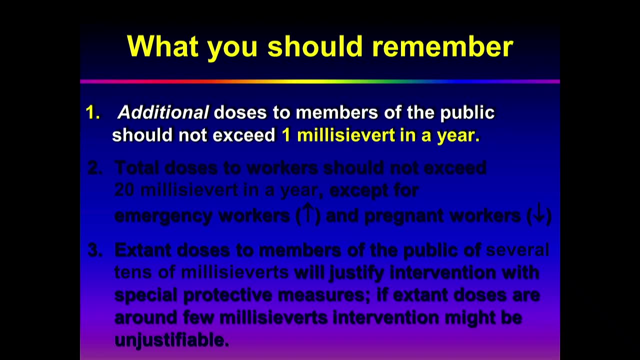 which has been approved and there are not very big changes between these two Take away points. Additional dose to members of the public should not exceed one millisievert. Total dose to workers should not exceed 20, but the margin can be higher. 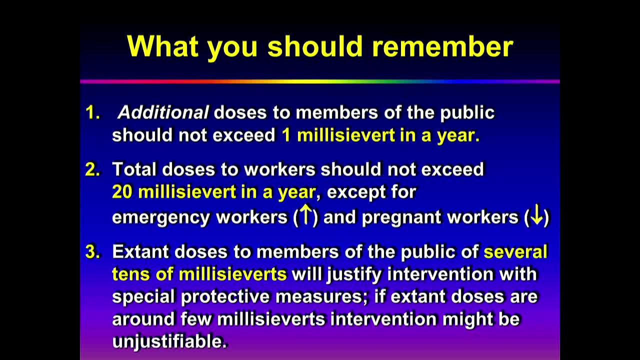 and pregnant. lower Extant dose to members of the public of seven and ten millisieverts will justify intervention with a special protective measure If around one few millisieverts the dose is less than one millisievert. the dose is less than one millisievert. 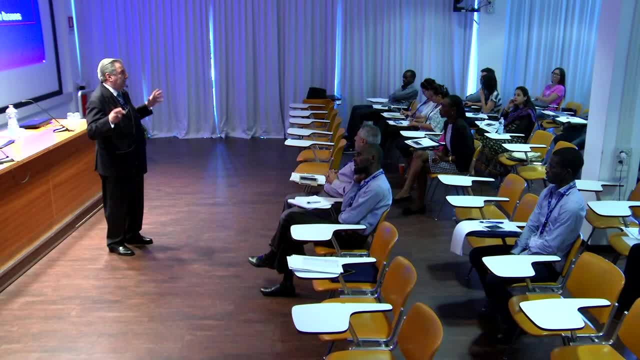 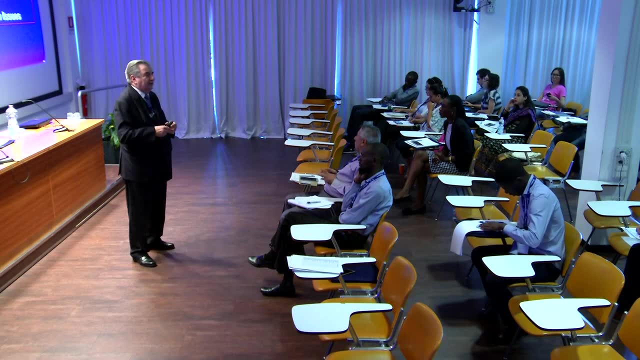 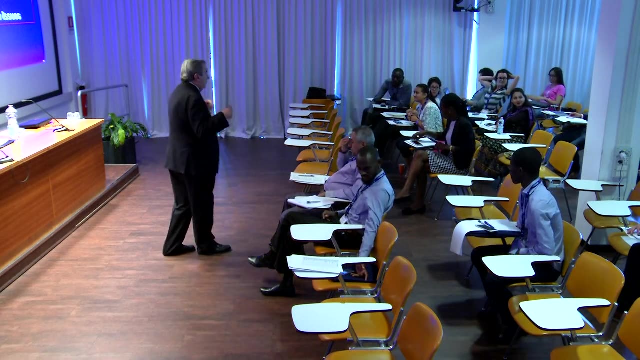 Second part of new issues. I will do that in the afternoon because I want that these new issues, which are the more important, you concentrate well in these new issues, and now, as it is 10.30, is a good time for coffee. 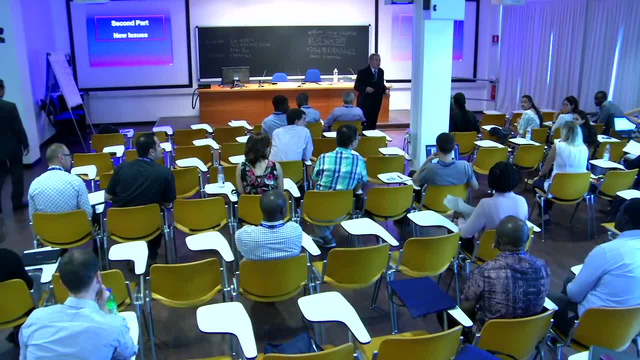 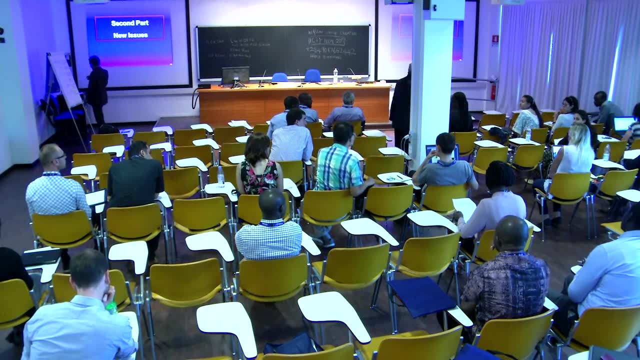 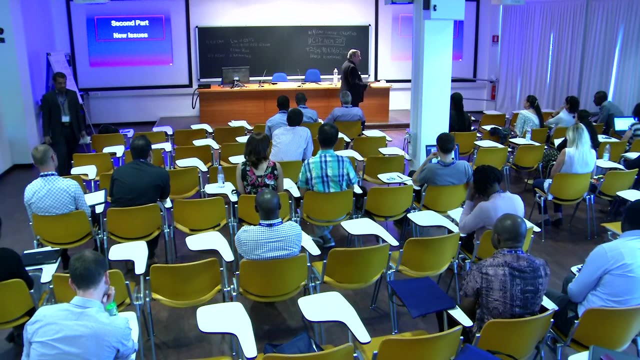 okay, Good, Any question before we go to coffee? Quick question please? Ah, that is a good question. Well, I will give you to you, my personal experience. Well, the question has to do with something that we discussed yesterday. If iodine is a very big problem, if in Chernobyl it was the only big problem because children got milk with iodine. iodine goes to the thyroid and you get thyroid cancer In children, not in us, particularly in my age. 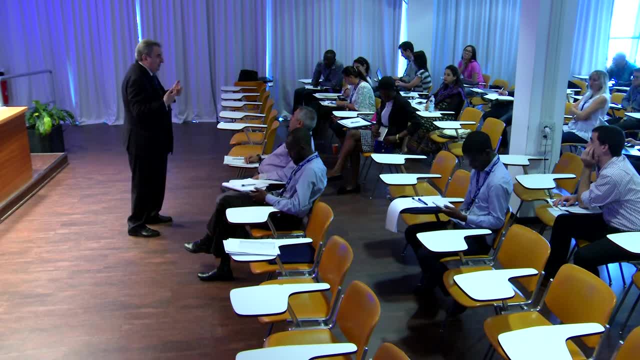 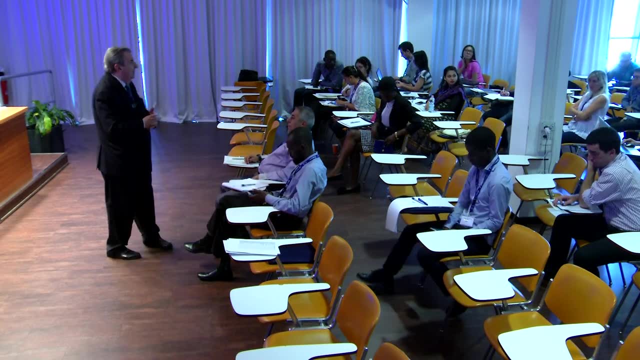 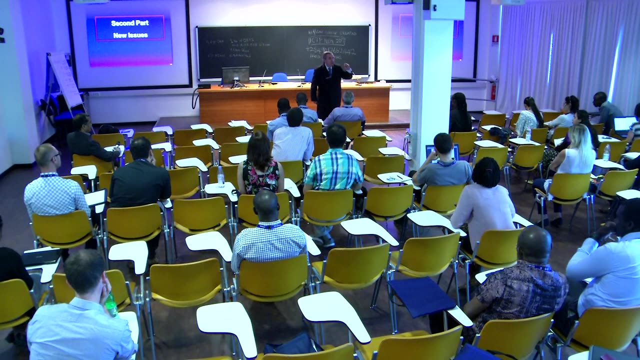 stop the world, basically. but for the children it's very active, For one technique- of which I'm sure Rafael will talk more- that is being used in Austria, for instance, is to have pills of iodine- non-radiative iodine. 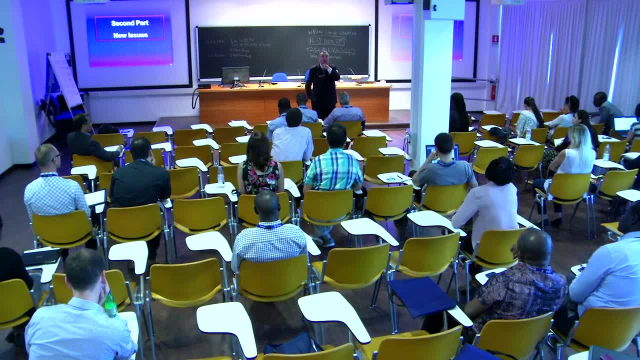 that, in theory, if an accident happens, you have to give to the children. this iodine will go to the thyroid of the children because the thyroid will be full of iodine. My personal opinion is that this technique- probably Rafael will say differently- 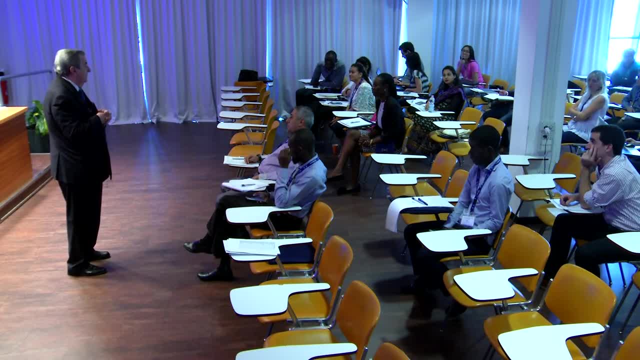 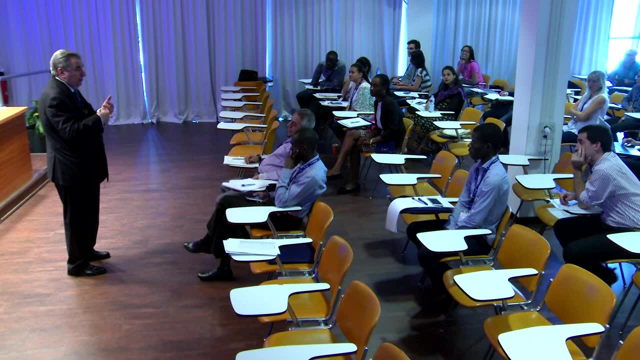 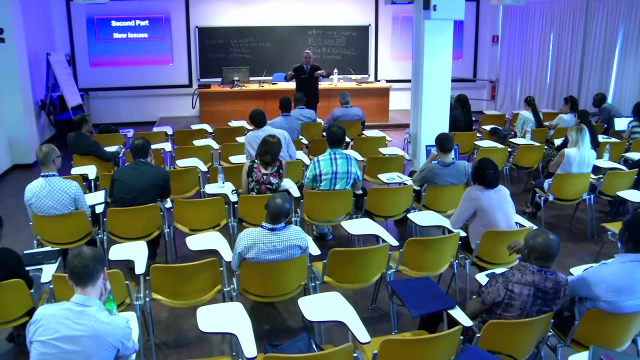 but my personal opinion is that this technique is a nonsense. I will explain to you why. First, because the iodine has to be changed continuously, because with time it changes the properties. For it's a very big operation in Austria going to the school. 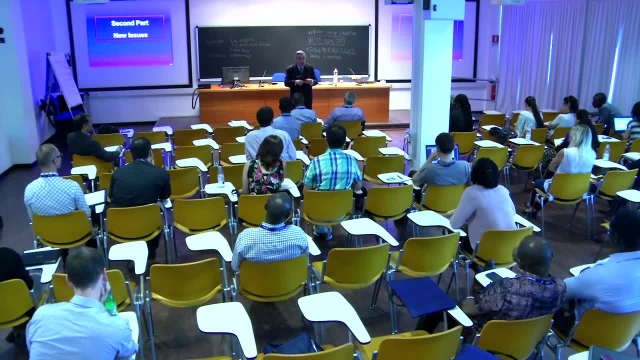 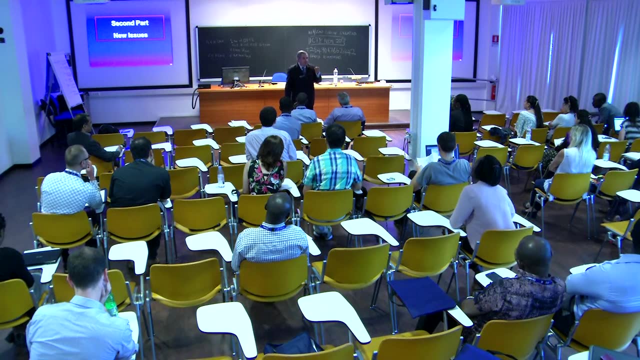 second, this iodine is not innocuous. Given a lot of iodine you can have other risks. And third, because it's not necessary. The best way to stop the radioactive iodine go to the thyroid of the children is not to give. 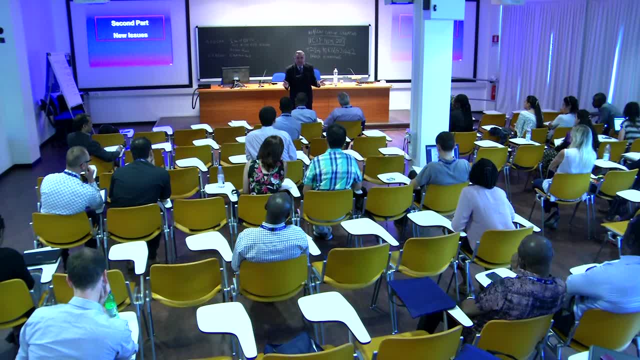 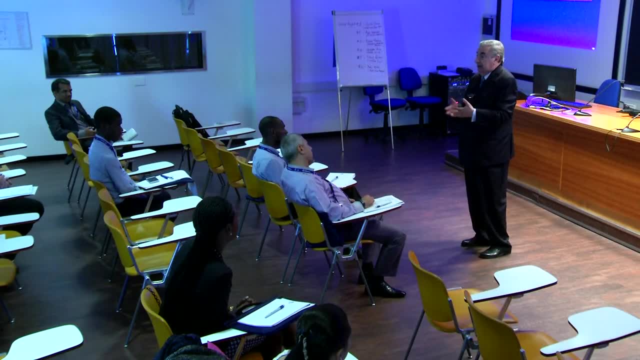 contaminated milk to the children. It's much more easy And in fact in Chernobyl this happened in countries where the people know what was happening, Even in countries that are not particularly well organized, like Poland. In Poland, the precipitation. 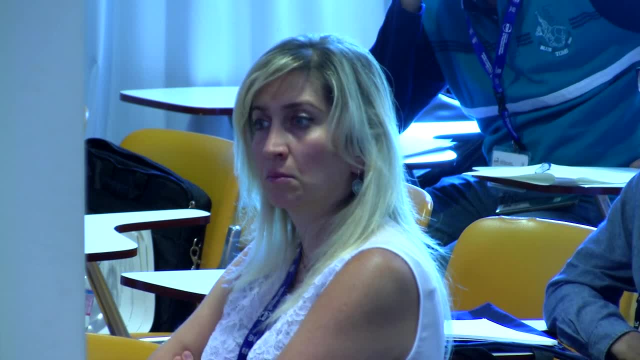 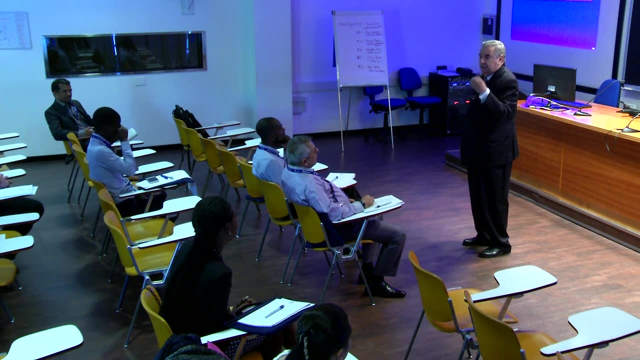 of iodine was very big. You know what the government did: Went to the radio and to say: mothers, please, during a few days don't give to your children fresh milk, Give condensed milk. That was all In Poland. there is no one single case. In Japan. there was not one single case. Why? Because the Japanese stopped the distribution of milk. This is much more easy than the pill. Now, if you're in a country with your government, do not tell you that there was an accident. 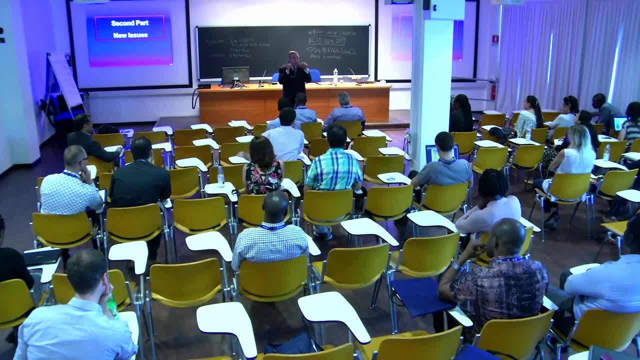 This is what happened in Belarus in particular, When the Soviet Union didn't inform. Then the mothers didn't know anything and they continued to give milk to the children. But if the pill would have been there, it would have no effect, because the government 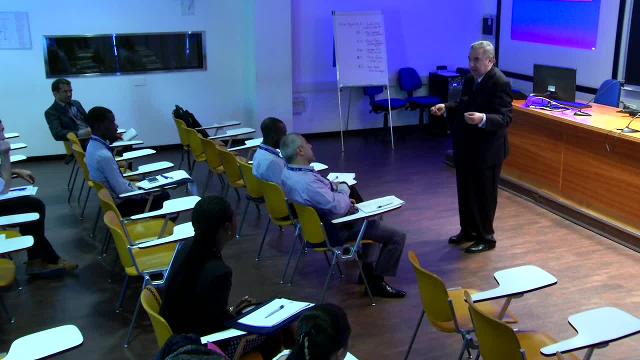 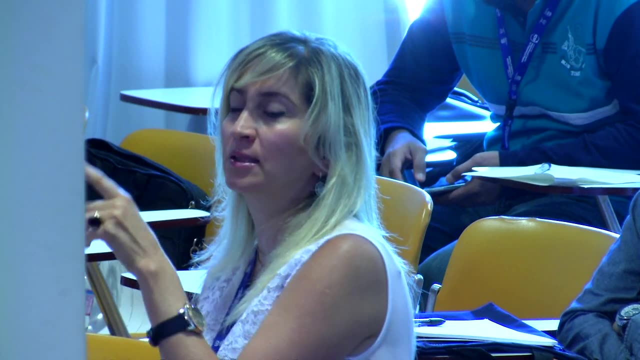 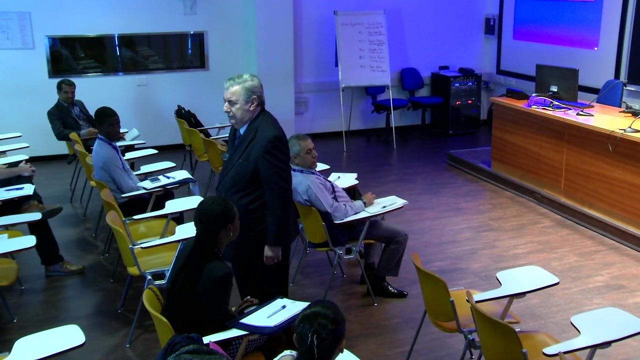 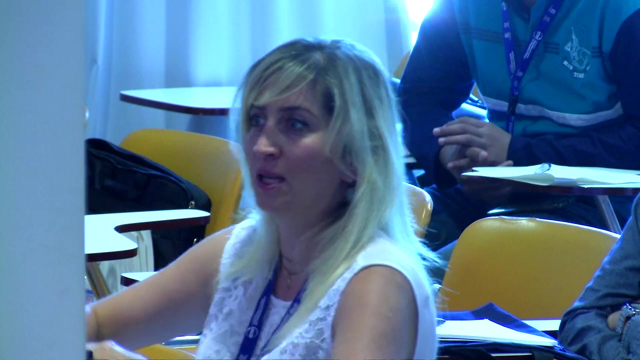 would not distribute the pill either. This is my personal opinion. So the third thing is, if an accident occurs, the third thing that you have to be sure, milk should not be given to children. Punto, Fresh milk, Fresh milk, That is a good point. That is a good point. I mean you. by evacuating people that are in a very, very low radiation area, you can even increase those who are not people. You move the people to an area where the natural radiation is higher. It will not be decay. 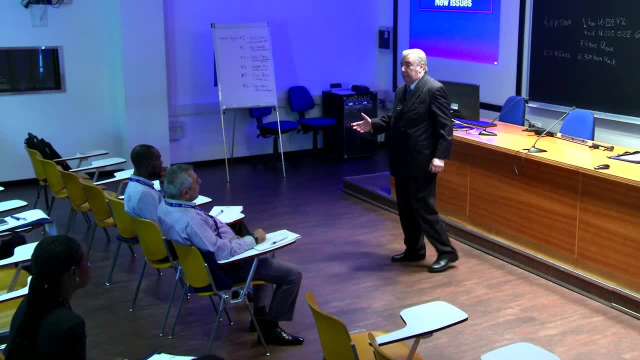 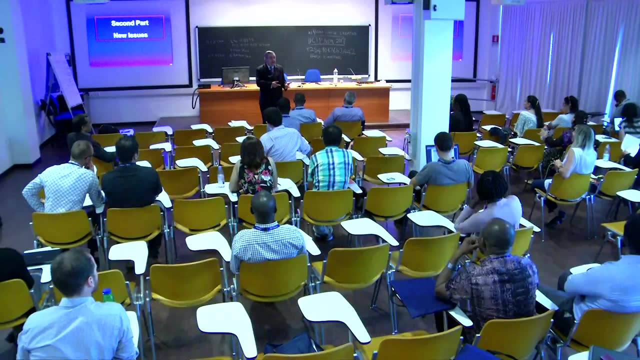 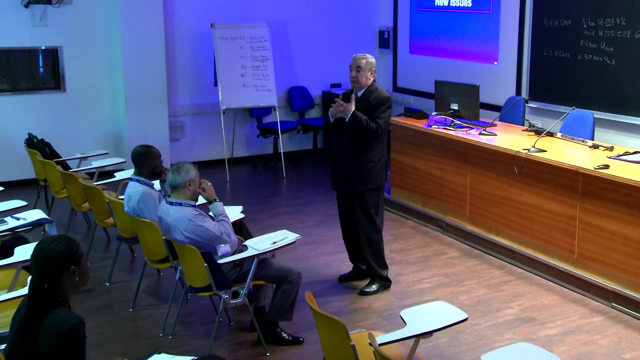 but suppose an accident in an Indian plant decides to evacuate the people and to send them to Kerala, They will receive my doses to be in Kerala than to be in the plant. These are the problems with the issue of evacuation. First of all, as I mentioned yesterday, it's a language issue. Evacuation is not the same as relocation. It's not the same as resettlement- Two different concepts. In Japan, the same word was used for the three. People didn't know whether they were going forever. 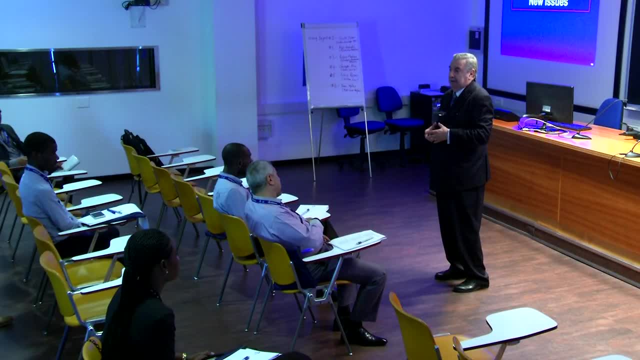 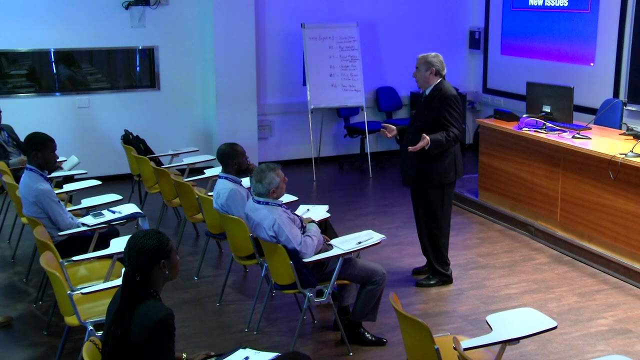 whether they were going for one hour And Rafael will talk about. I mean, evacuation is a possibility, but there are other possibilities before that have to be considered. The first thing is a more simple one, that is, to shield. I mean to shield yourself, not home. 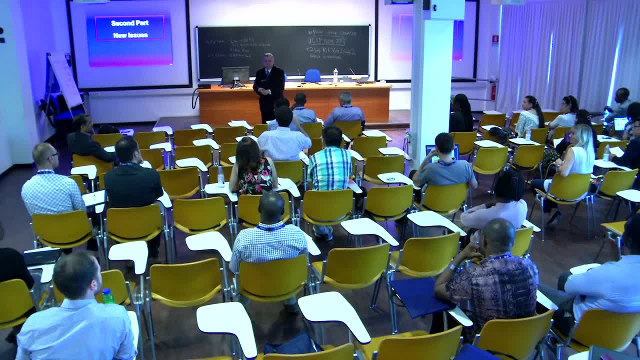 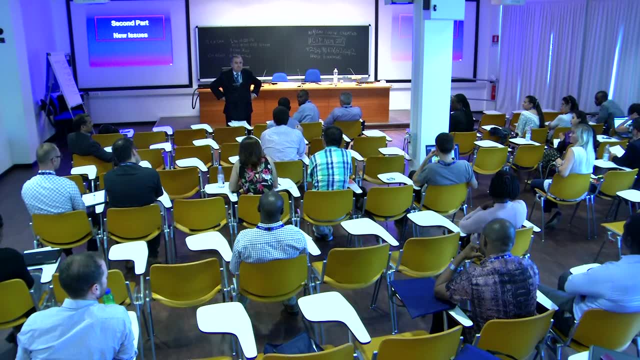 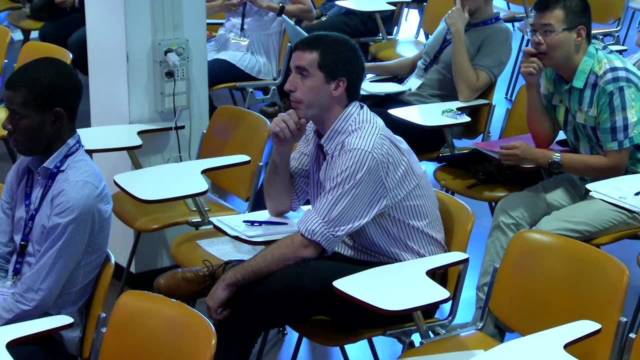 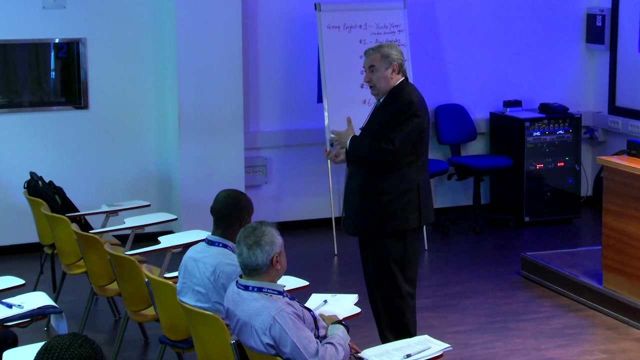 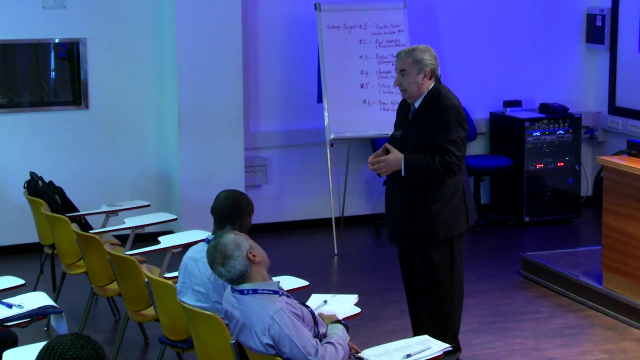 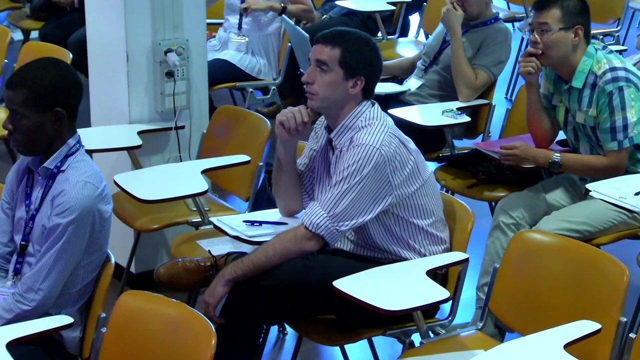 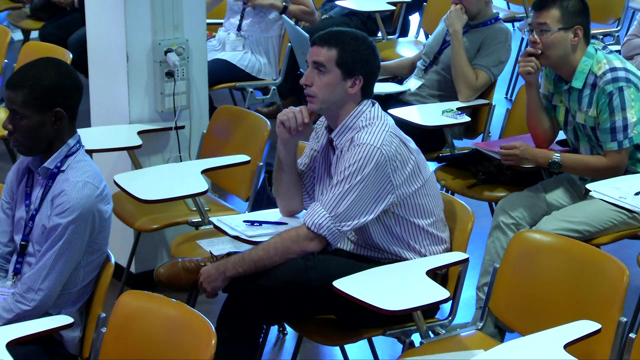 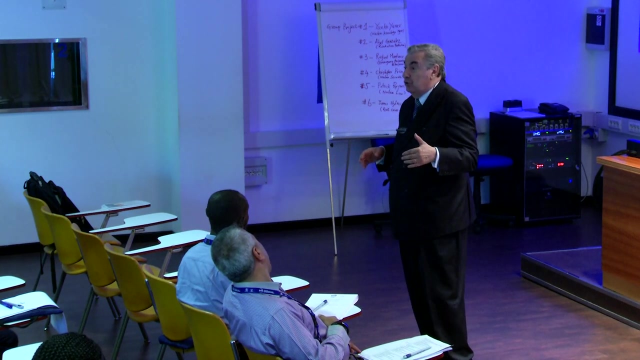 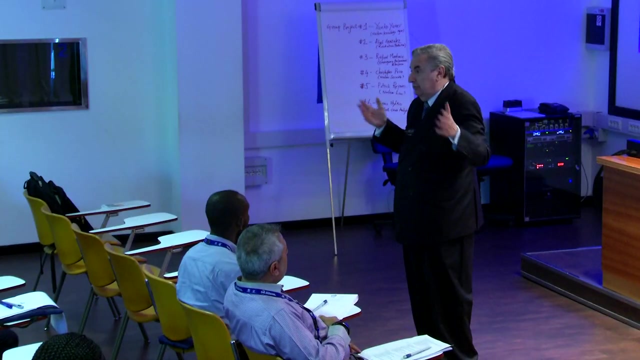 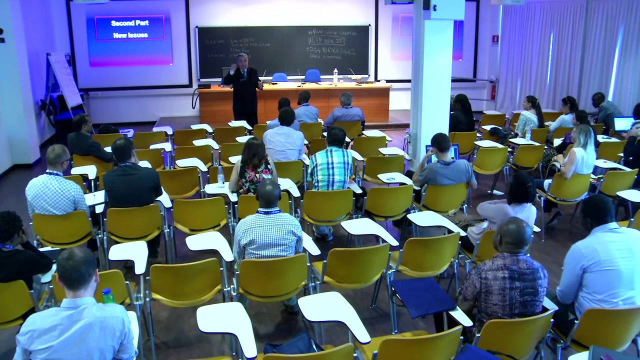 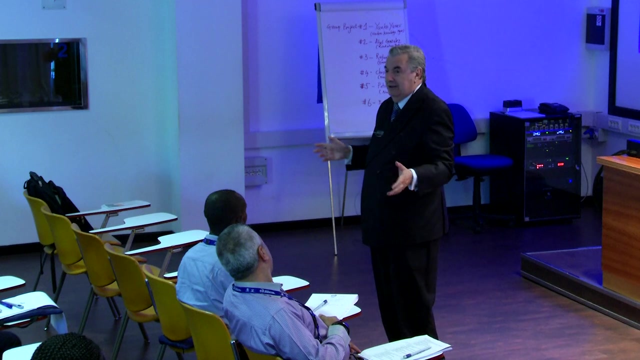 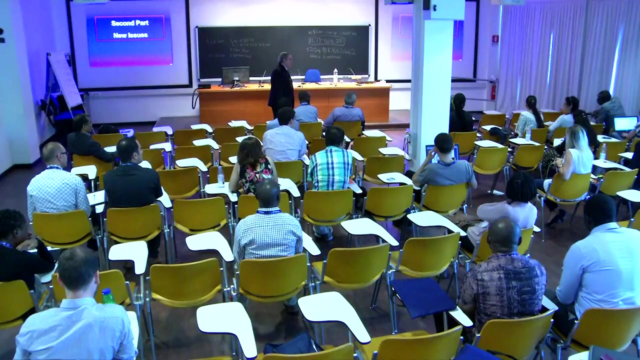 Any other? Yes, please. 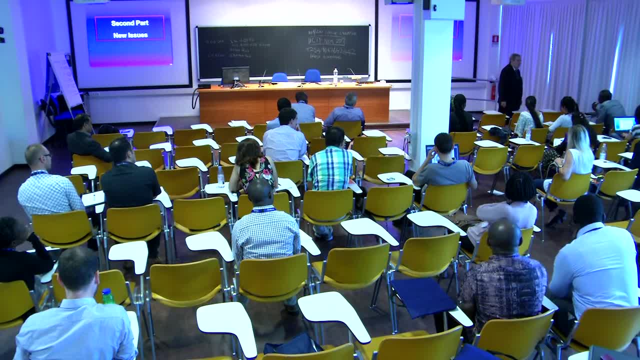 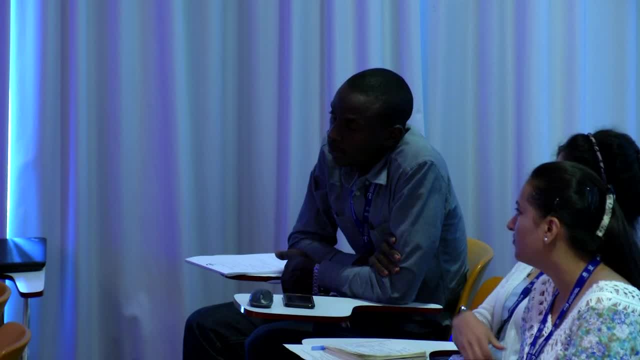 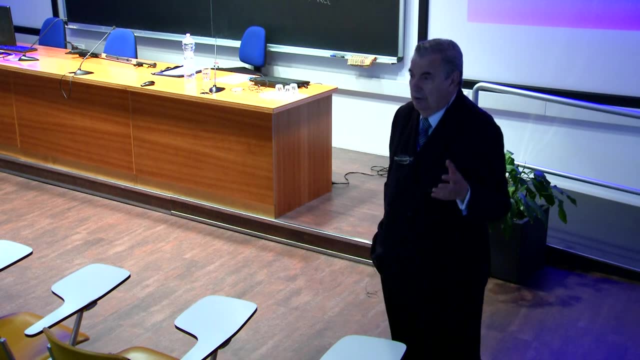 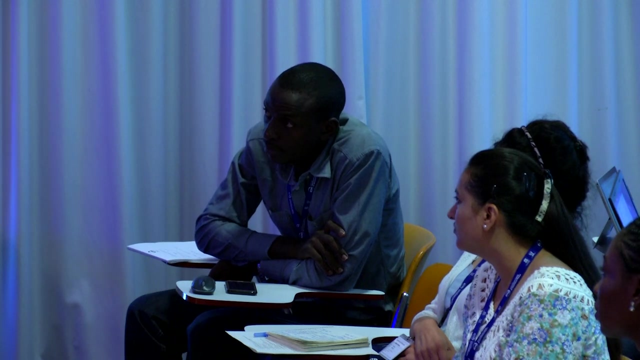 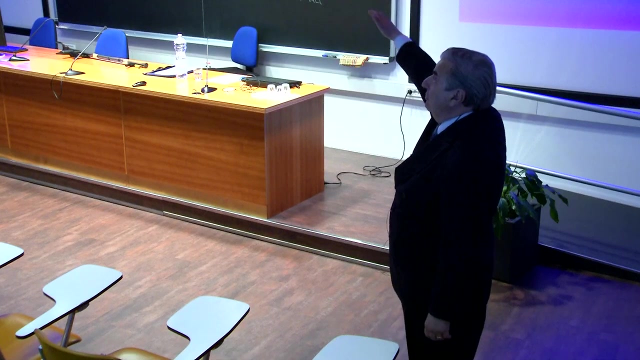 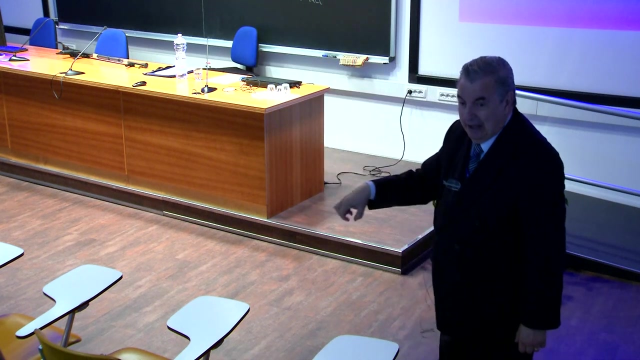 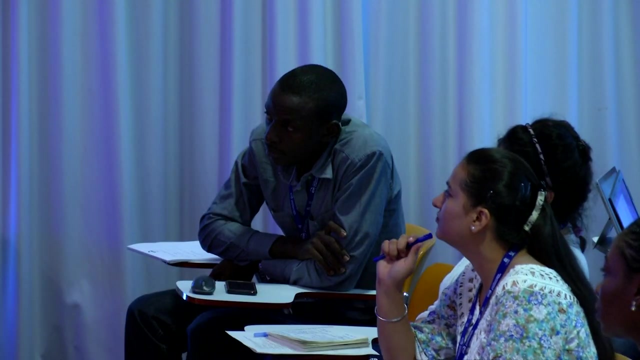 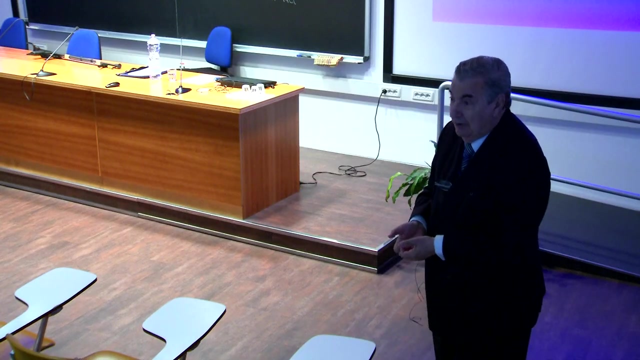 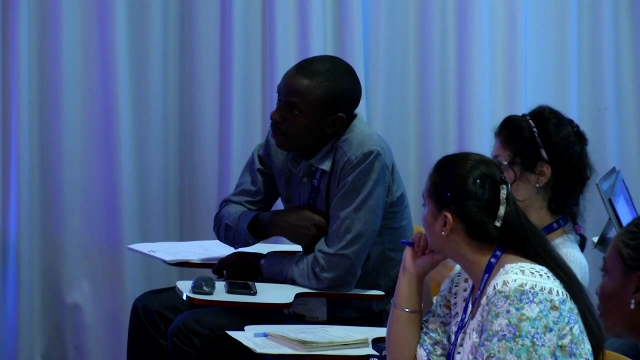 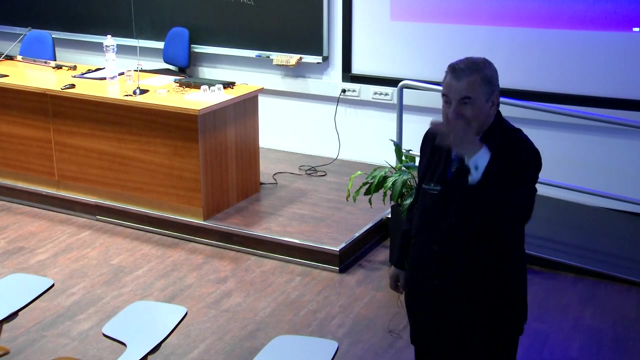 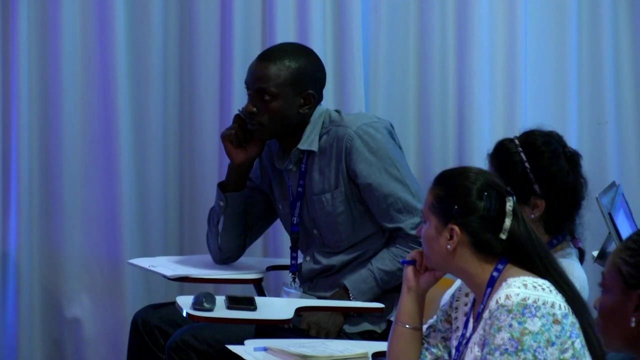 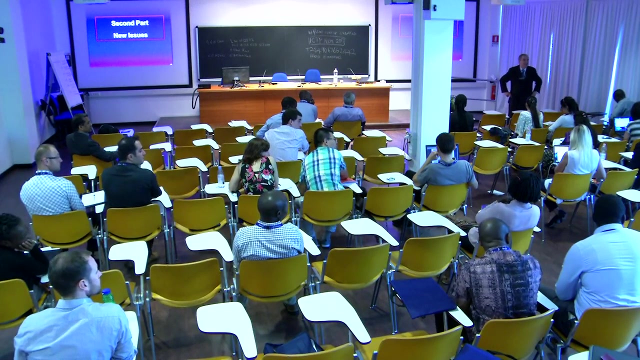 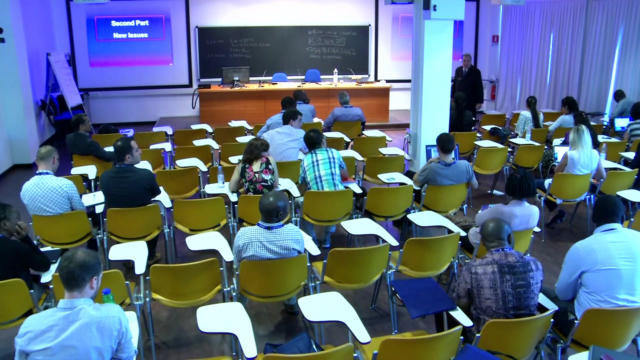